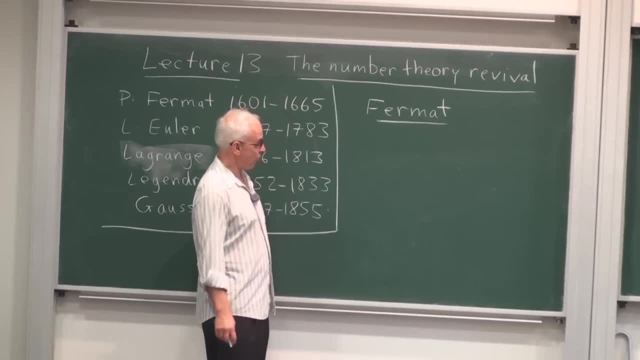 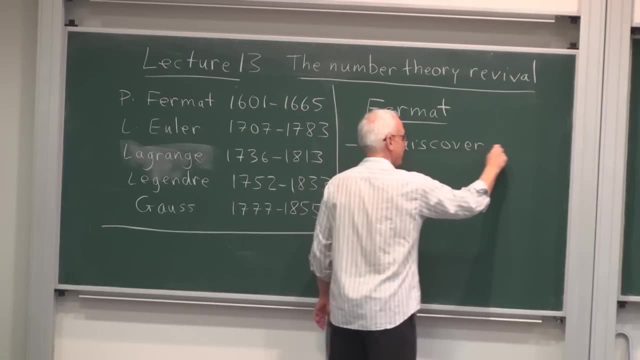 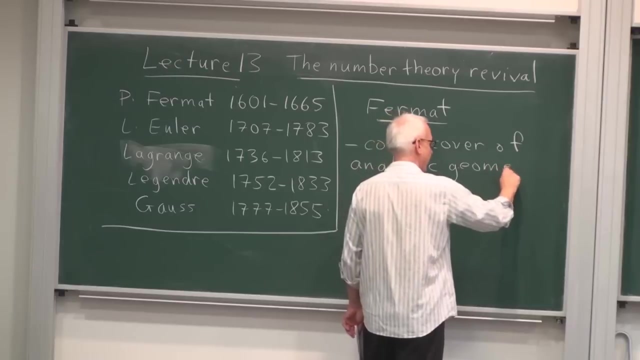 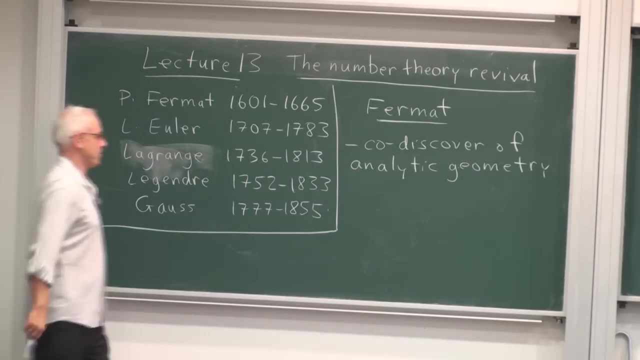 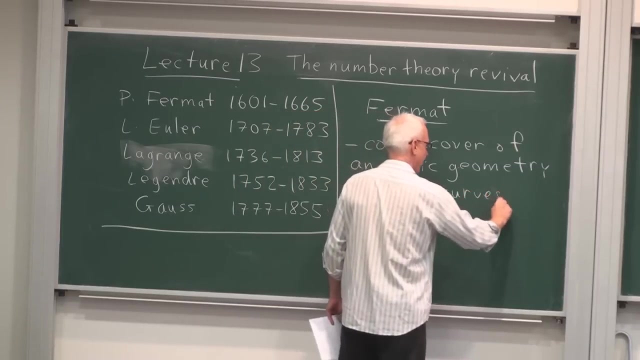 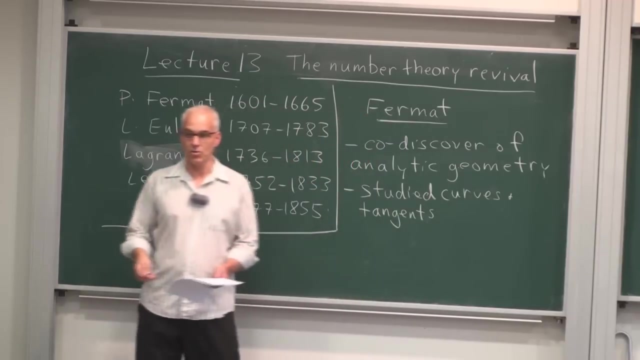 So Fermat worked in in a number of different areas and he contributed in an important way to analytic geometry. He was one of the co-discoverers of analytic geometry with, of course, Rene Descartes, And he investigated properties of curves and tangents and contributed in fact to some of the preliminary work before the calculus was discovered. 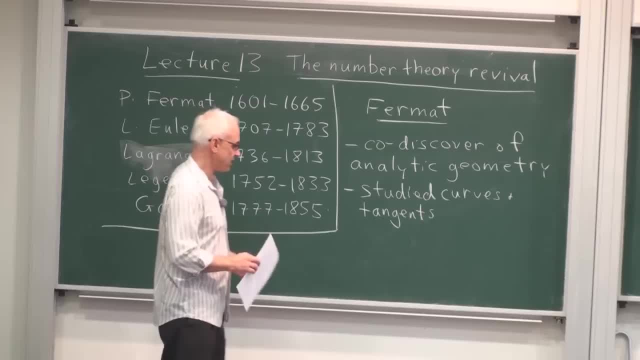 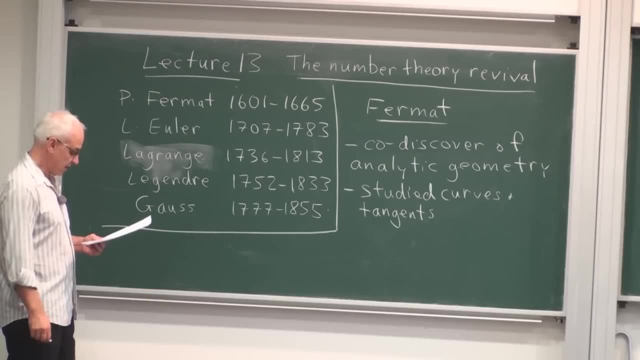 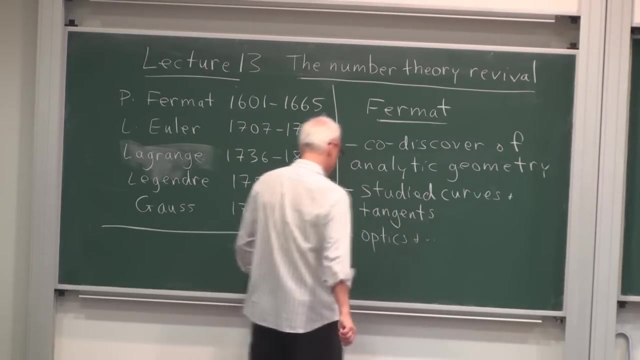 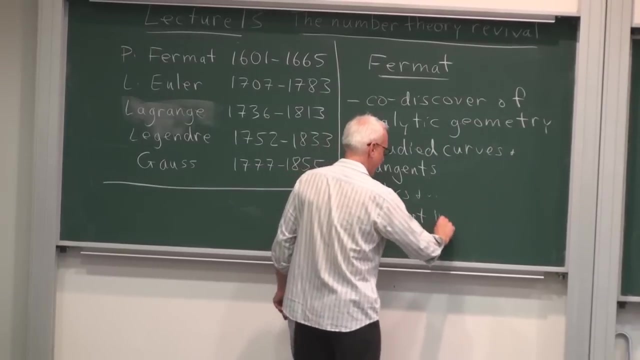 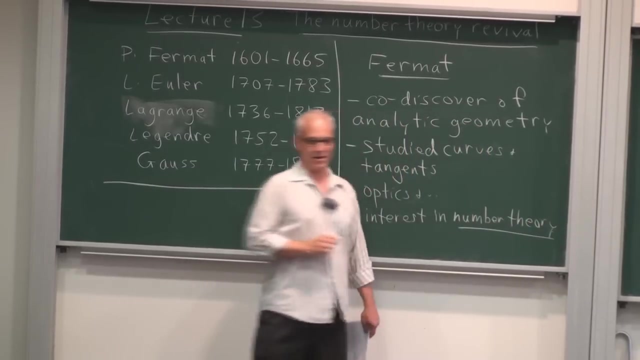 And some people give him credit for some of the discoveries in geometry. He also was interested in other things. He did some work in optics and other areas, but his main interest was in number theory, Which wasn't really a subject back in his day. 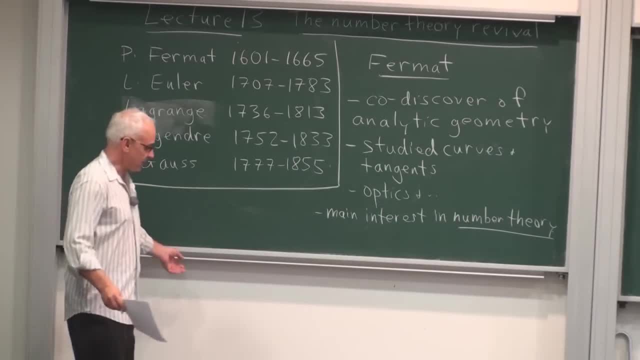 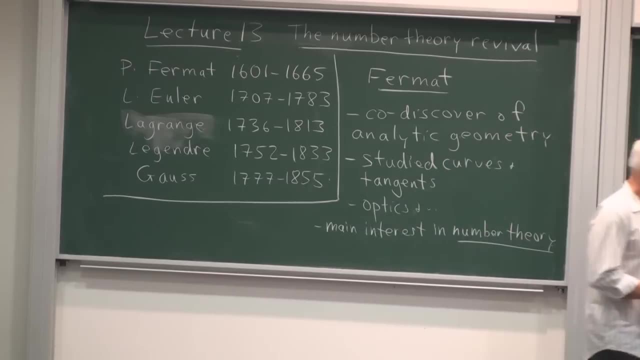 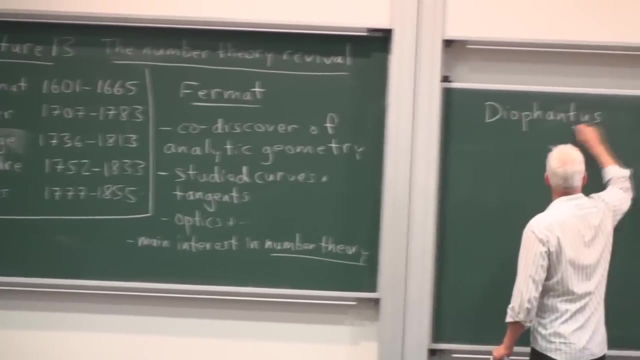 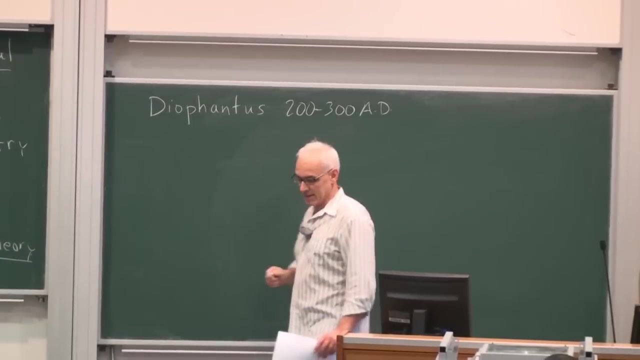 So what had happened in the number theoretical, in the pure number theoretical context before that? Well, we had basically Diophantus. So Diophantus of Alexandria lived around 200-300 AD And he, we've talked about him already. he was a fellow who 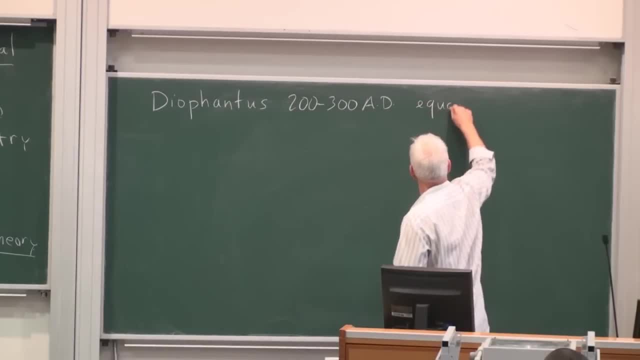 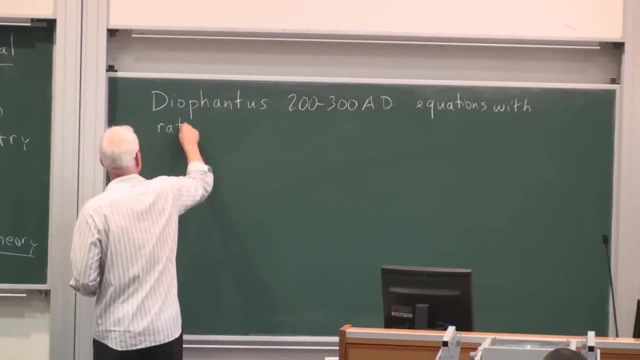 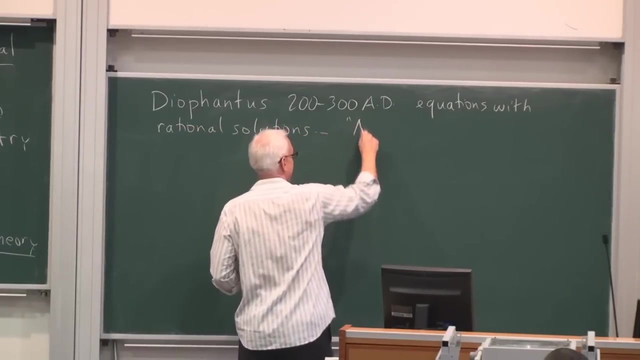 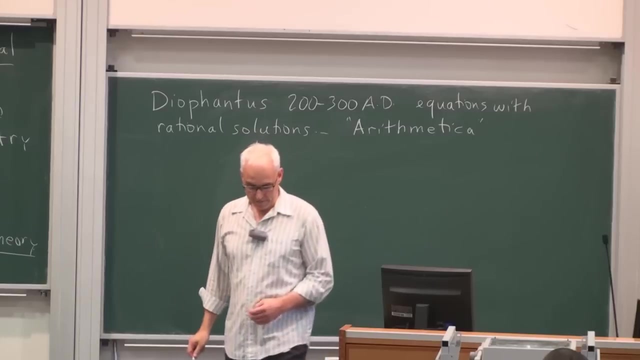 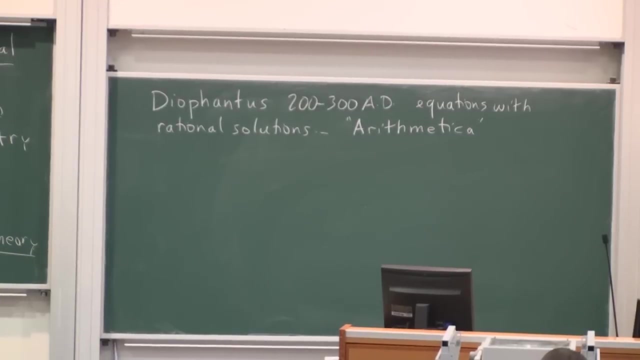 studied equations with rational solutions And he wrote a book called Arithmetica Which was recently translated, in Fermat's time, in the Greek, And that was one of the very influential drivers of Fermat's thinking. Of course we have the work of the Arabs and the Greeks and the Hindus after this period. 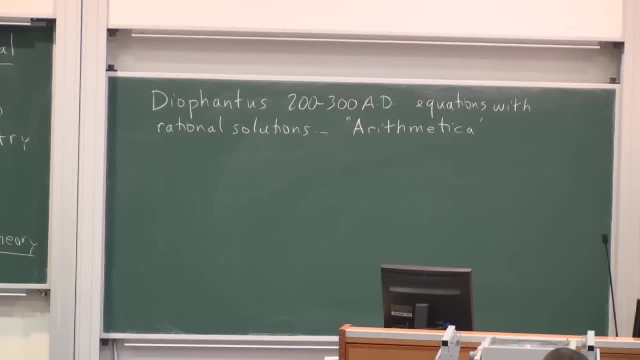 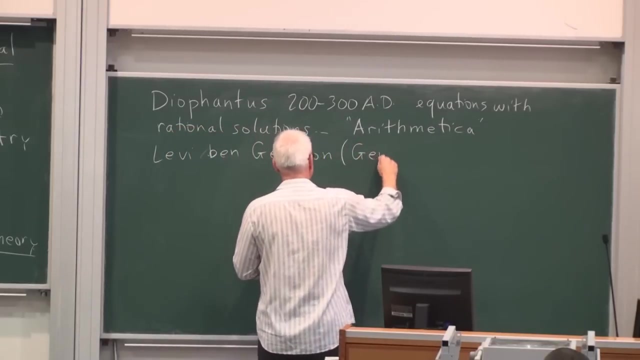 Who also contributed algebraic tools, But sort of in terms of purely arithmetical considerations. there wasn't a lot between the ancient Greeks and Fermat, With another notable exception, That of Levi Ben Gershon, Who's also referred to as Gersonides. 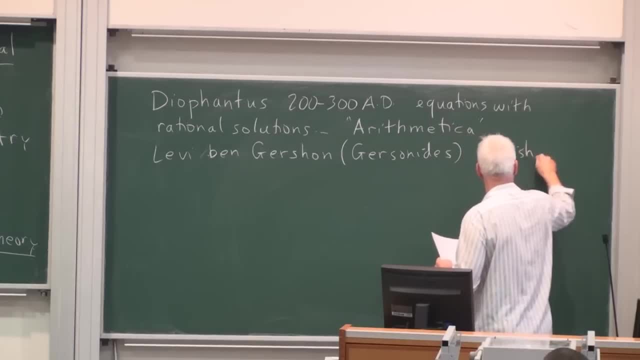 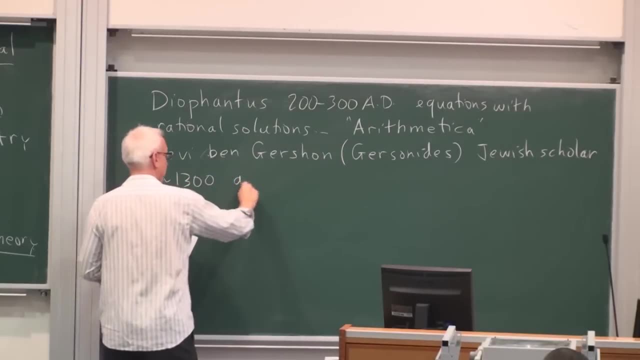 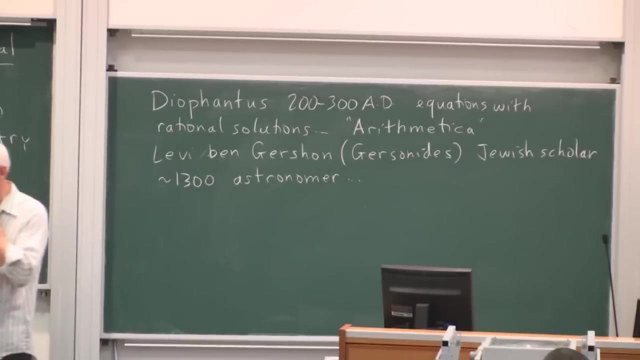 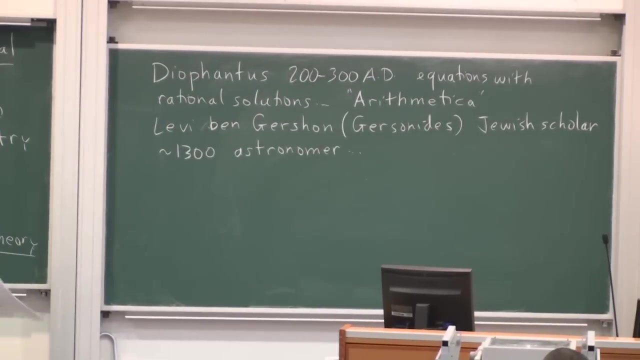 And he was a Jewish scholar Who lived around the time of 1300.. He was also an astronomer And he was very instrumental in discussing combinations and permutations. So of course the binomial theorem goes back long before that. We have Pascal's triangle going back to the Chinese, and so on. 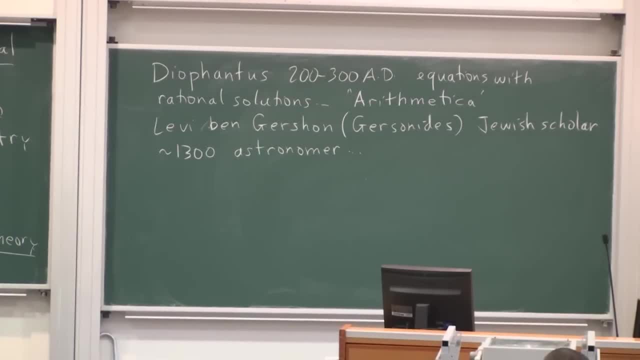 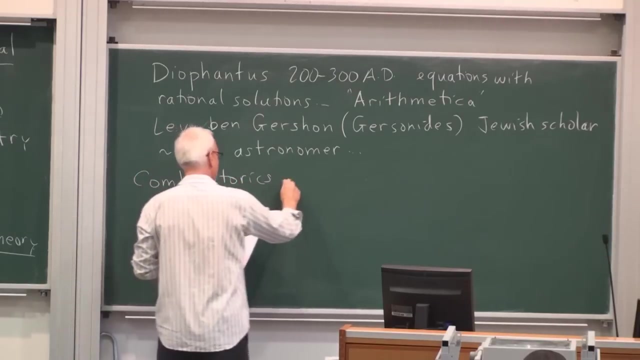 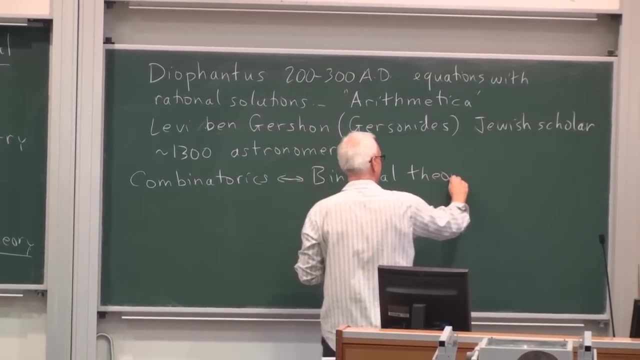 But Levi Ben Gershon was perhaps the first one to understand the combinatorial significance of Pascal's triangle and the binomial theorem. So he introduced the combinatorics associated to the binomial theorem. So let me remind you that if you have something like a plus b to the fifth, 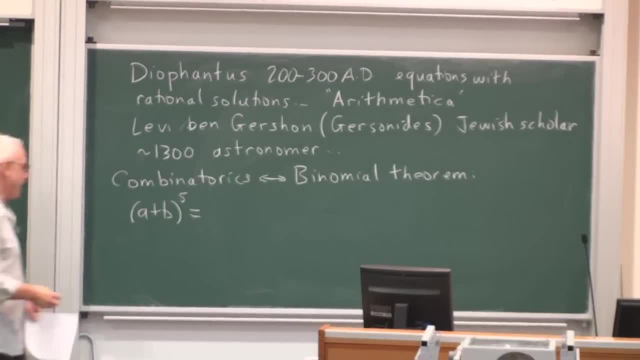 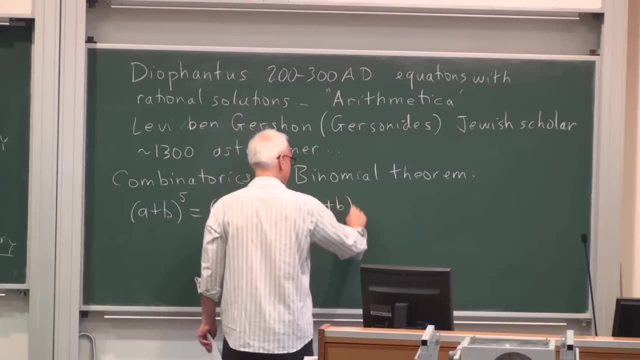 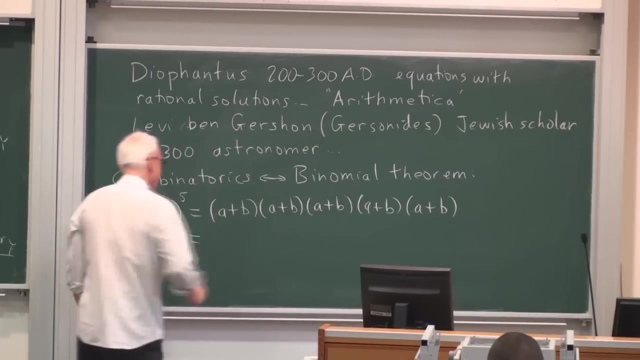 Then if you expand that out, you have basically five products: a plus b, times a plus b, times a plus b, times a plus b and one more a plus b- And the binomial expansion is just what you get when you expand all of that out using the distributive law and collecting terms. 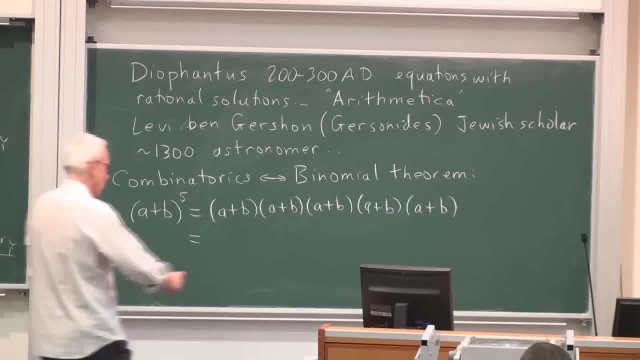 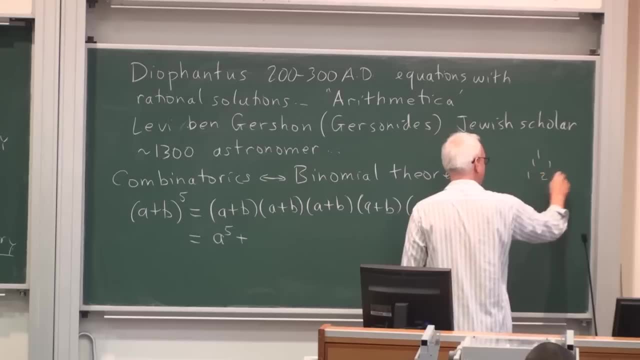 So nowadays all students know this is a to the fifth Plus. and then there's some numbers Which we get from Pascal's triangle. So there's the relevant fifth row. So the coefficients are a to the fifth And then five a to the fourth b. 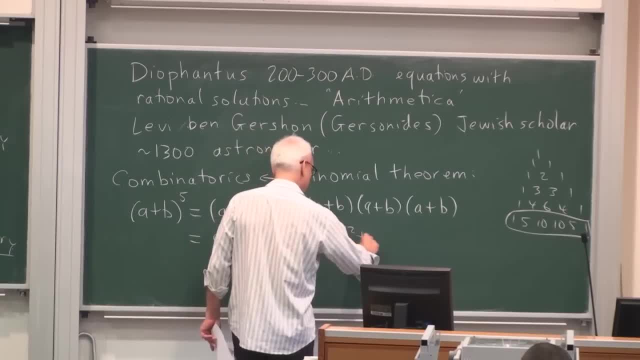 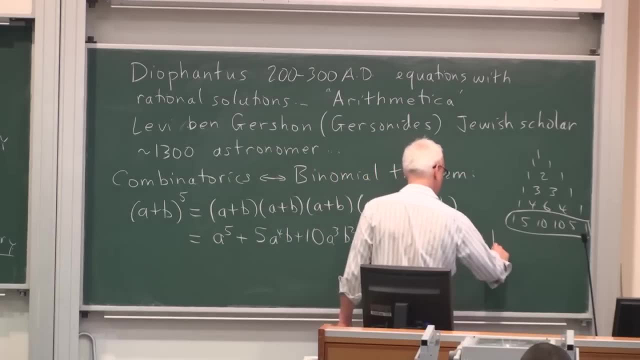 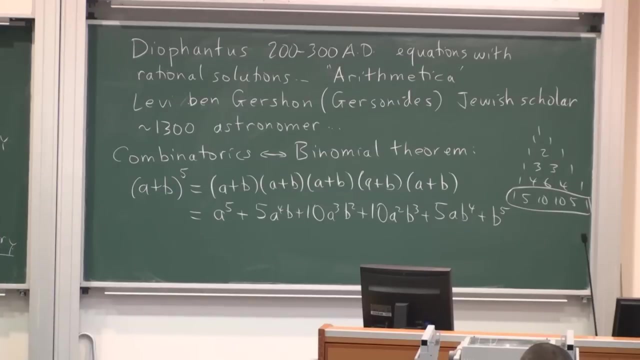 Plus ten a cubed, b squared. Plus ten a squared b cubed. Plus five a b to the fourth Plus b to the fifth. And Ben Gershon realized that there was some counting going on here, That if we look at one of these terms, 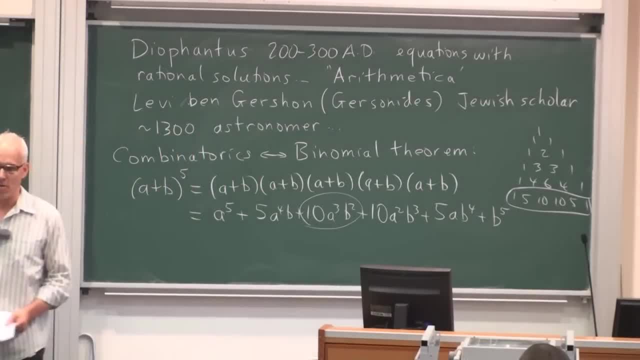 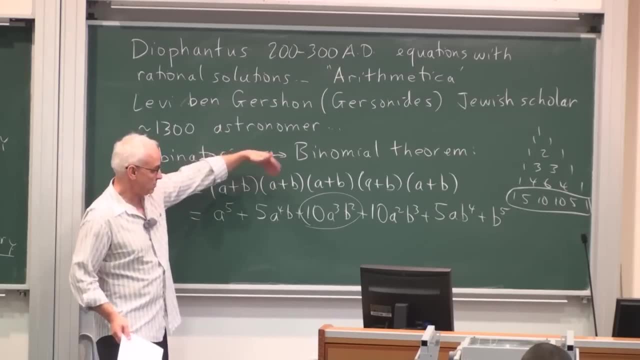 For example. say this one here: Where do we get the ten from? Where's that ten coming from? Well, we're looking at all the ways we can get a cubed times b squared When we multiply something from this one times something from this one. 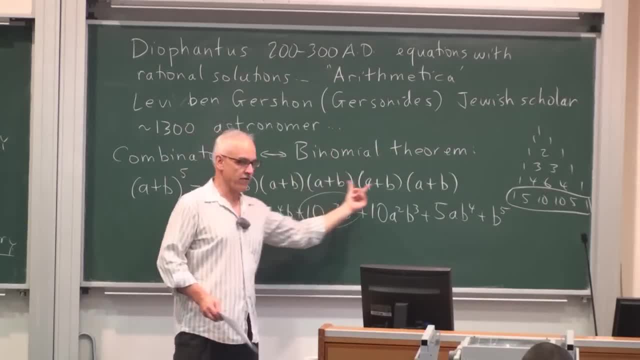 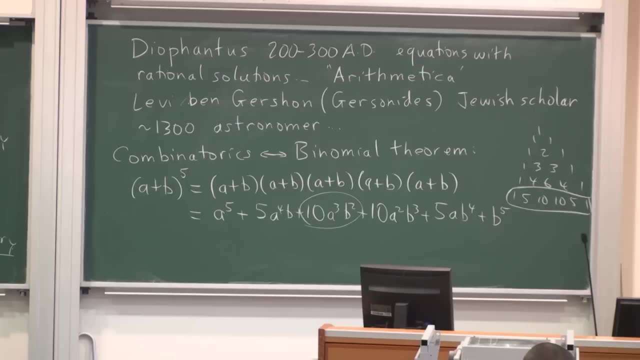 And so on times something from this one. So we have to choose one term from each one of these brackets And combine them And we're looking at how many ways can we get an a cubed times b squared. So this ten. 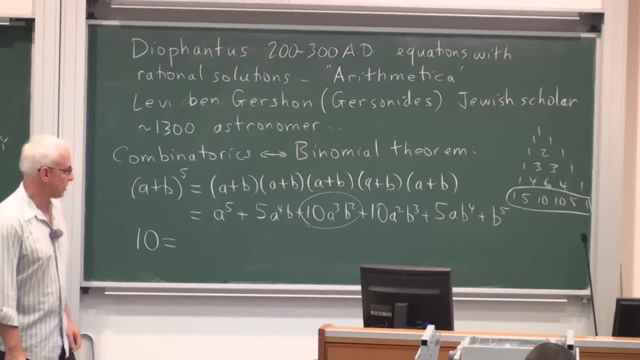 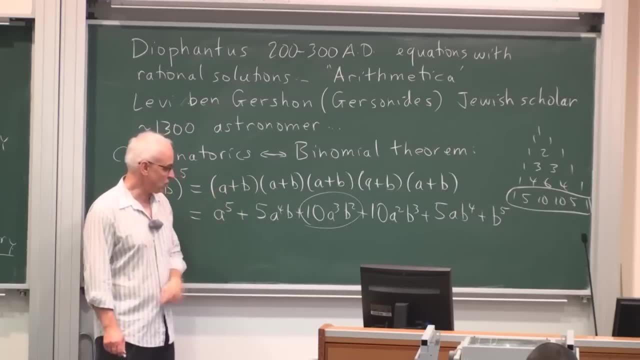 Was the number of ways that you can choose. Say, two b's out of the five brackets. All together, we're going to get three a's and two b's, And if we know where the b's are coming from, Then the a's are coming from the other ones. 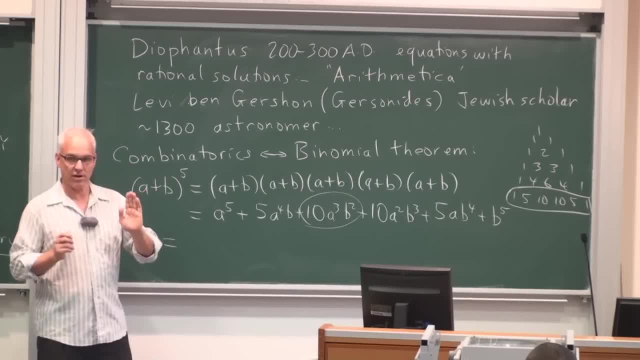 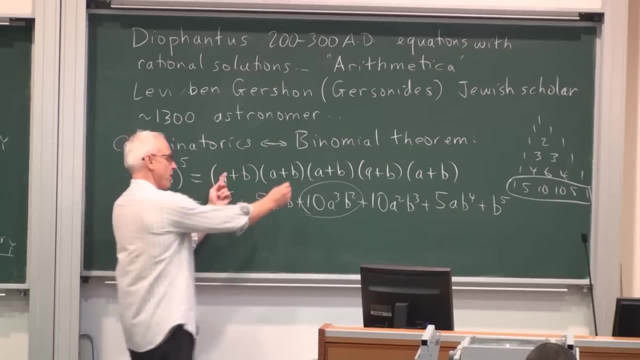 So it suffices just to worry about Which brackets are going to contribute the b's. Well, how many ways are there of choosing two brackets out of the five? That's one way: Two, Three, Four, Five, Six. 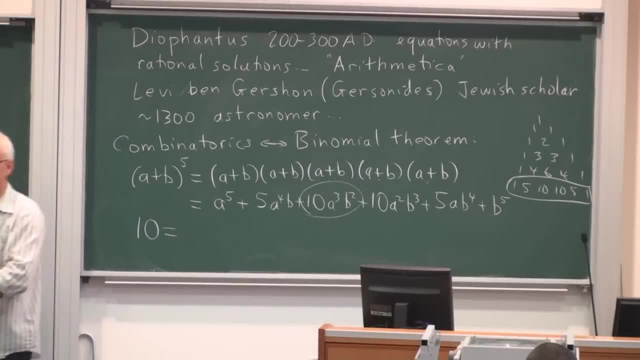 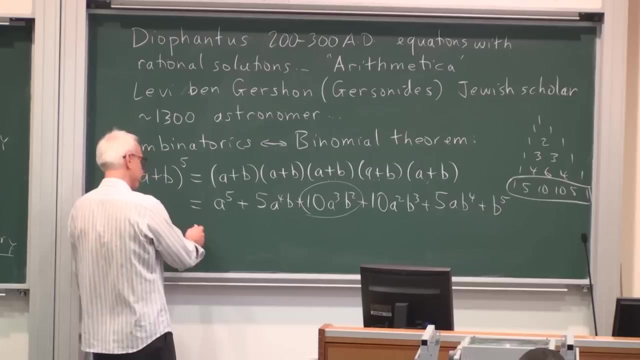 Seven, Eight, Nine, Ten, Those are the ten different ways of choosing two out of the five brackets, And those correspond to the various sums that contribute to this total here. So this ten, Which has nowadays the symbol five, choose two. 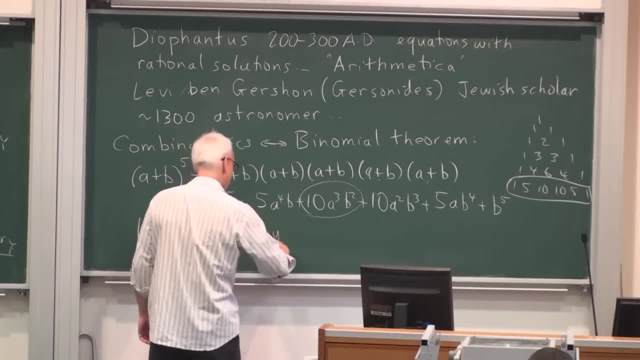 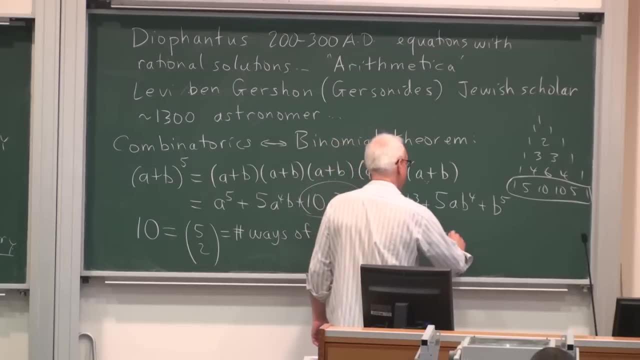 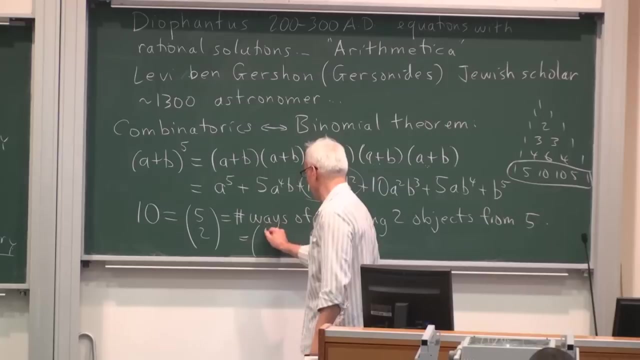 It's the number of ways of choosing two objects from a collection of five, And because it's symmetrical with respect to the a's and b's, We could also say it's the number of ways of choosing three a's. So it's the same thing as the number of ways of choosing three a's out of a total of five. 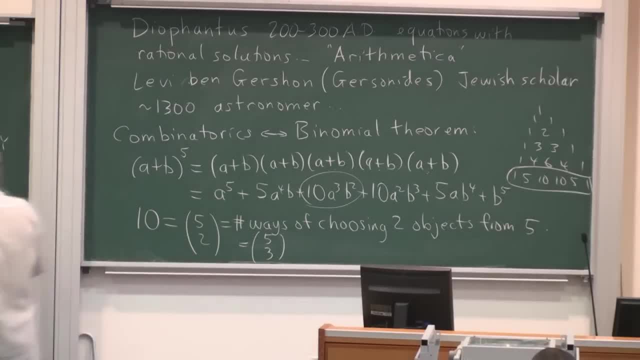 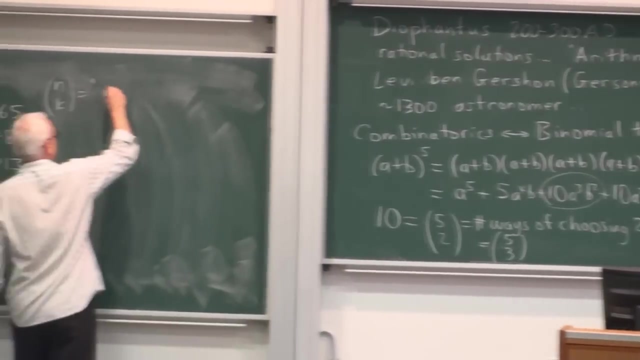 And in general, Bershon Ben Gershon also gave a formula for these numbers, And it's a formula that high school students learn these days. So the formula is that n choose k. It's often the way it's described with words. 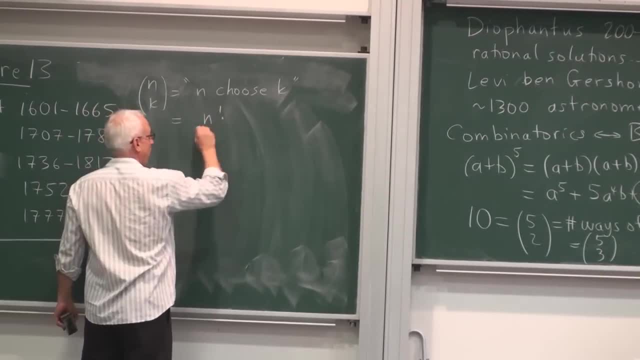 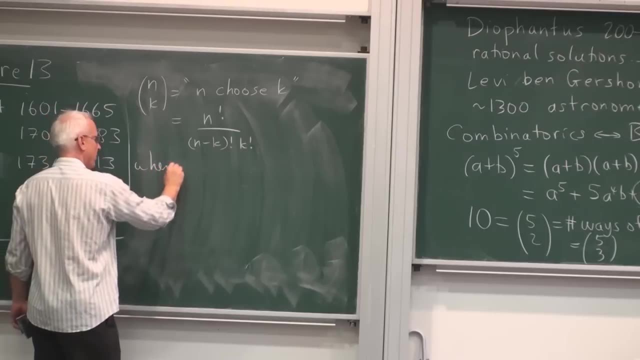 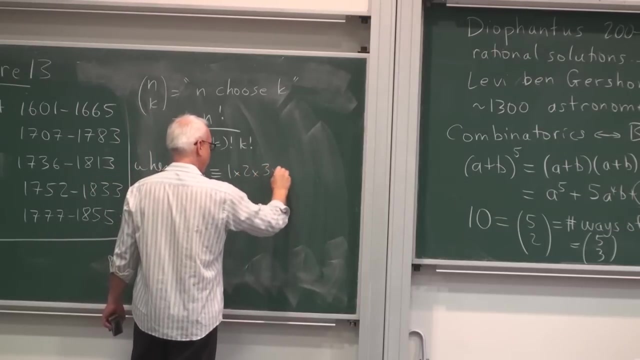 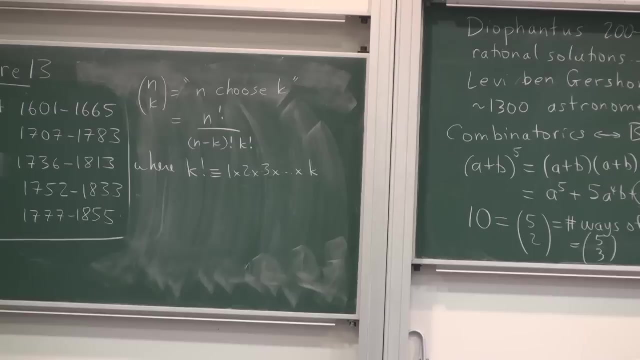 n choose k is equal to n factorial over n minus k factorial times k factorial, Where this symbol with the exclamation mark Say k factorial, means one times k Plus two times, three times, all the way up to k, The product of all the numbers from one to k. 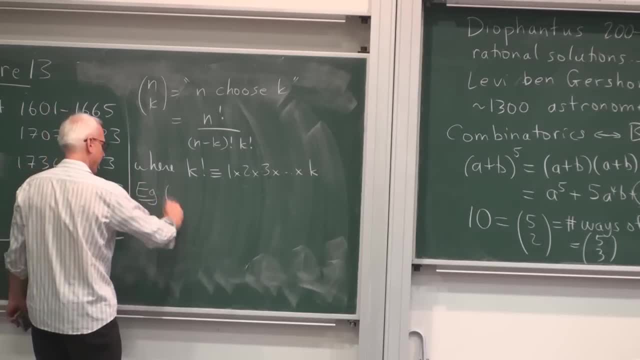 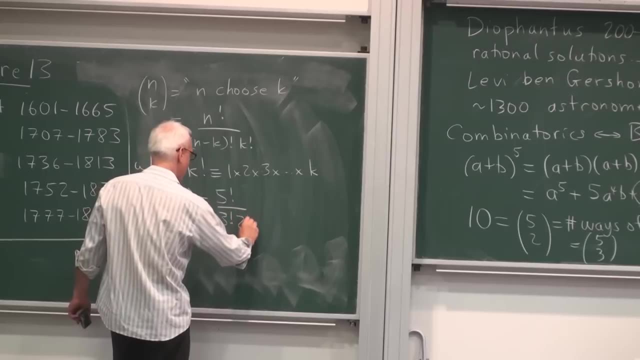 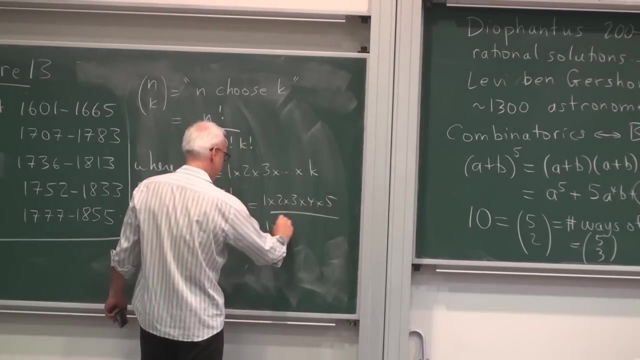 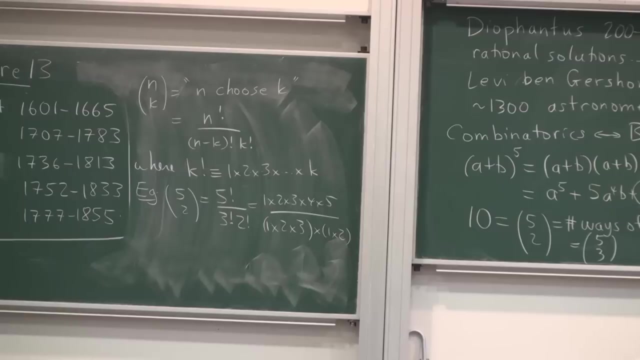 So, for example, five choose two Would be five factorial over three. factorial two factorial That's the same as one times two times three times four times five, Divided by one times two times three Times one times two. And so he explained why that formula arose. 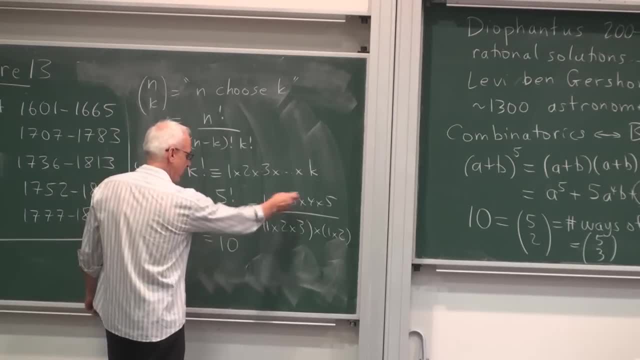 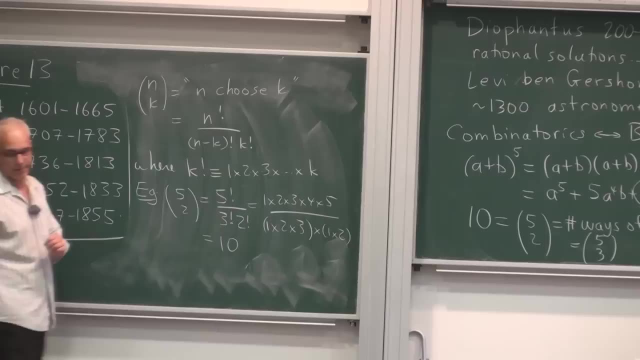 And of course we do get ten after we cancel various things. You can cancel that one, two, three with that one, two, three, And then you just get twenty divided by two, which is ten. So this is an arithmetical thing. 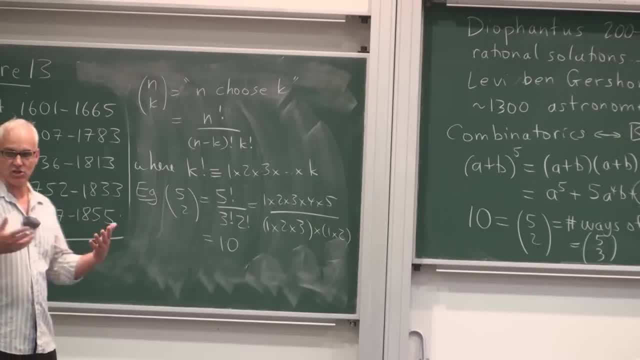 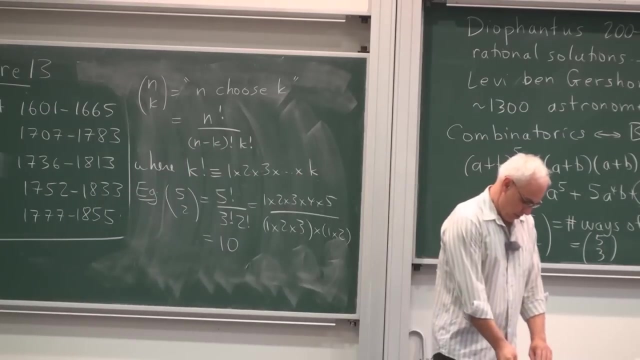 Because we're talking about numbers, We're interpreting numbers in terms of counting things, And the numbers are not exactly associated with geometry in the traditional sense. It's really numbers doing the job that numbers are supposed to do in terms of counting. Okay, so now let's come to Fermat's work. 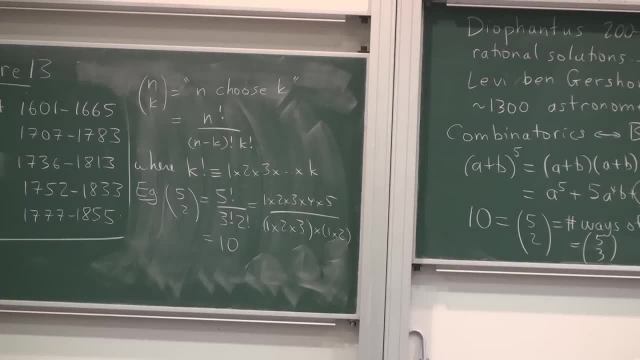 And some of the ideas that he introduced, Some of the problems he was working on, And in many cases he left things a little bit open-ended because he didn't provide proofs for some of his claims, In fact, for most of his claims. 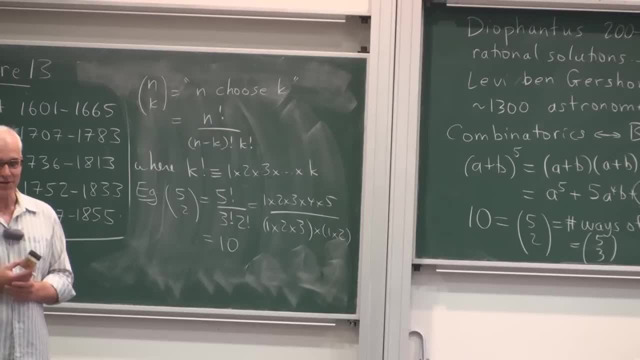 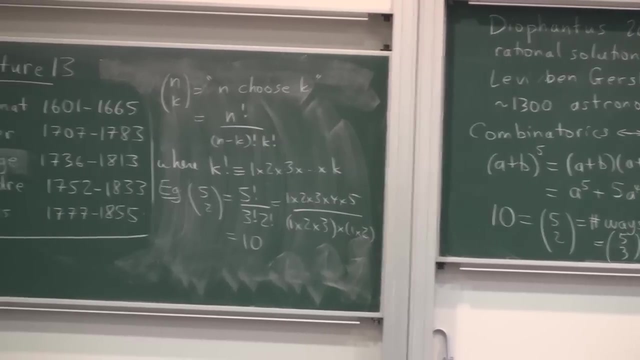 And so people didn't really know how he thought about things, And they didn't know, in fact, whether he actually entirely knew what he was claiming, And it took In many cases quite a long time after Fermat's dates for someone else to come along and prove the things that Fermat had claimed. 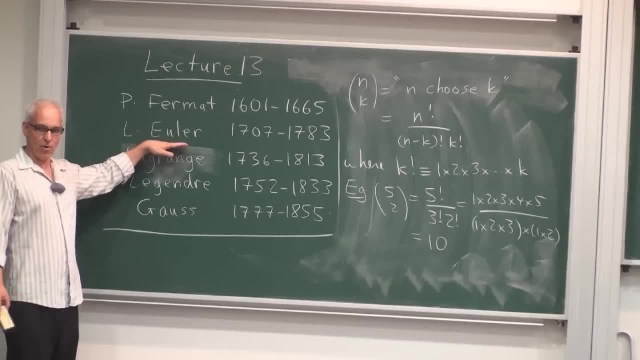 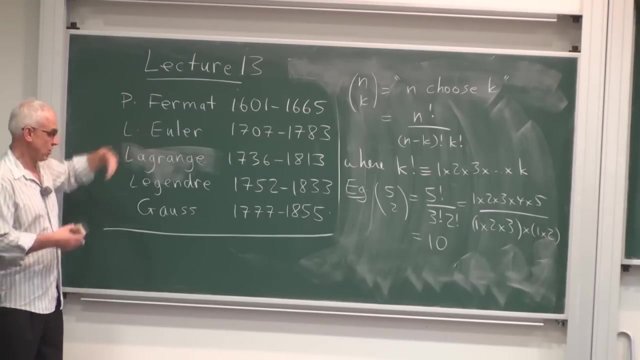 In particular Euler, who, I've stressed before, is the greatest mathematician of modern times. His interest in number theory was stimulated by getting a copy of Fermat's work And his friend Goldbach gave him a copy And he started investigating this stuff. 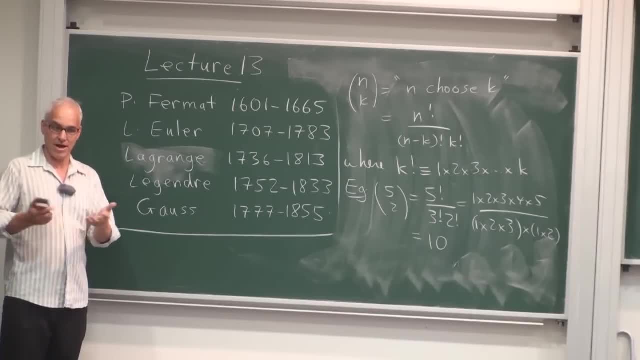 And he thought, well, this is great. And he ended up taking some of Fermat's ideas and sort of completing them or working hard to try to understand what Fermat had done, And he was able to make some progress, Quite a lot of progress, in fact. 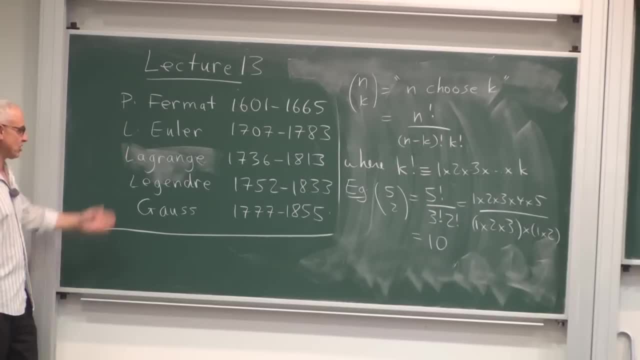 But then more progress had to wait for some later mathematicians, In particular Lagrange, And then other people who were very influenced by these developments were Legendre and Gauss. So these are amongst the great mathematicians of modern times. So let's have a look at what kinds of problems was Fermat interested in. 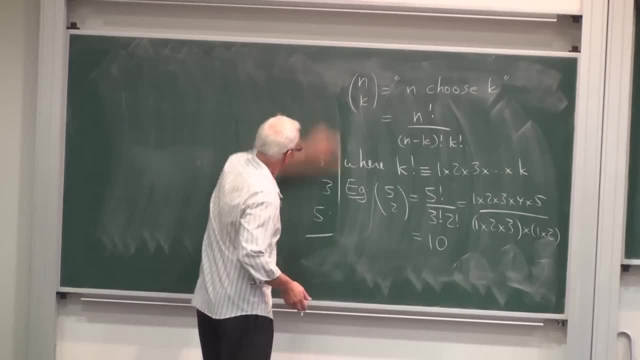 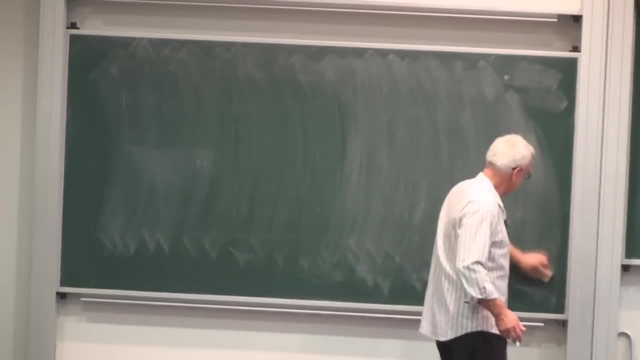 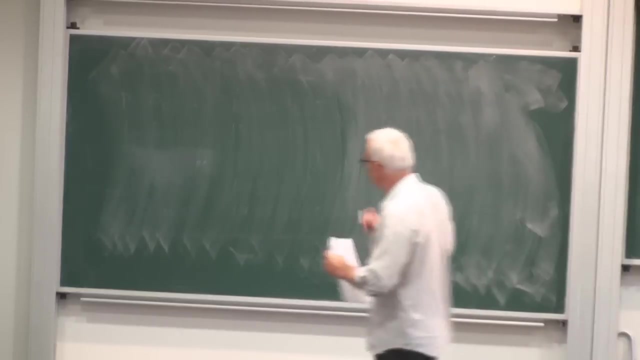 Well, he went back to the ancient Greeks and the kinds of problems that they were interested in With perfect numbers, Related things called amicable numbers, And he became interested in divisibility and related issues. But there were other A number of very specific things that he discovered. 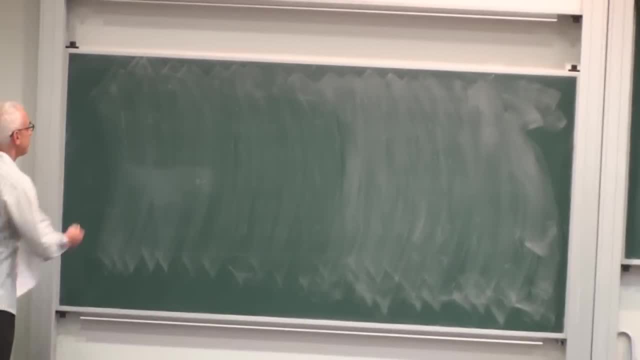 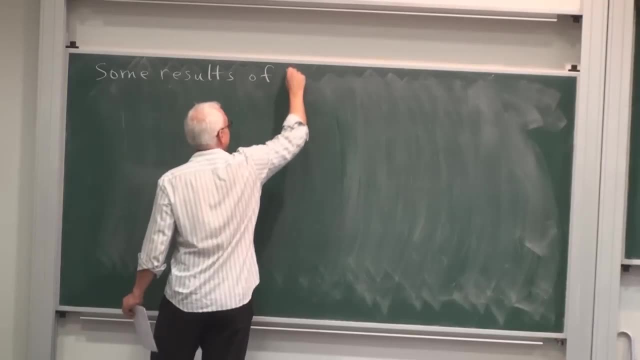 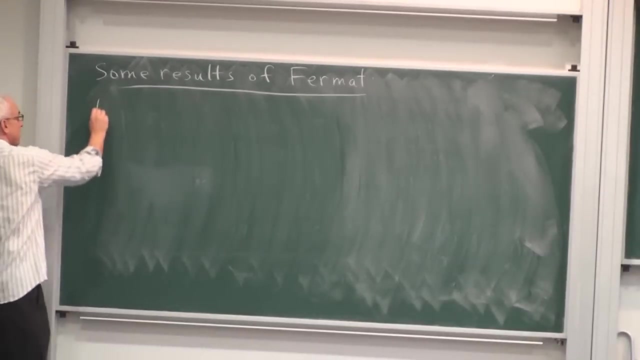 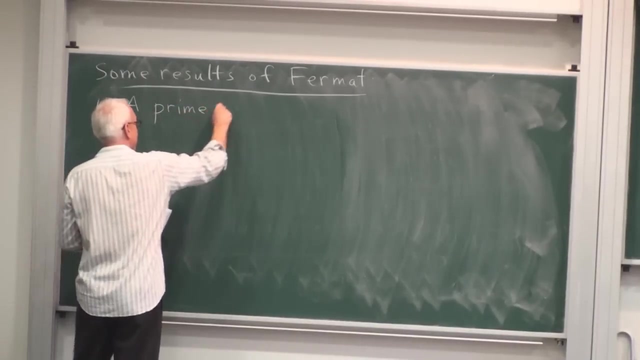 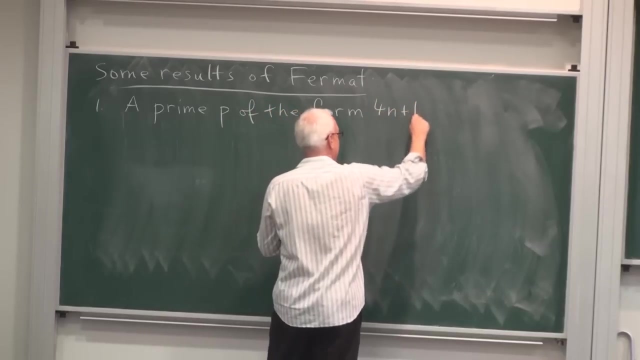 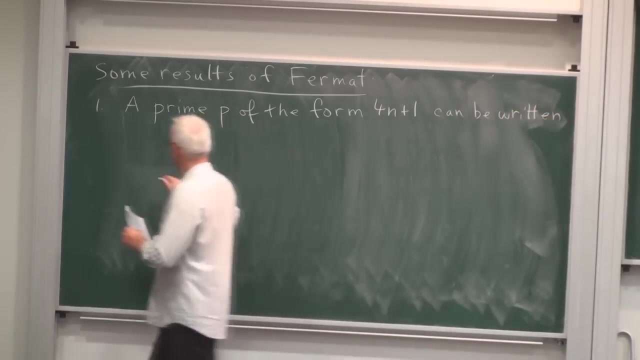 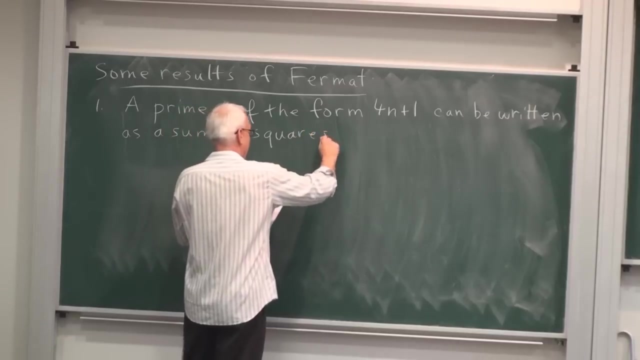 Quite beautiful and remarkable things. So some results of Fermat. Okay. so First we might say that a prime P Of the form 4n plus 1. Can be written As a sum of squares In exactly: 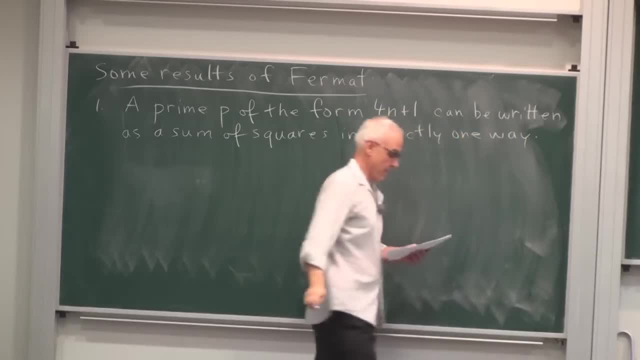 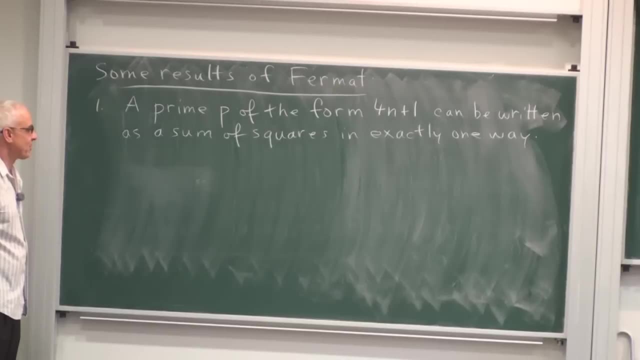 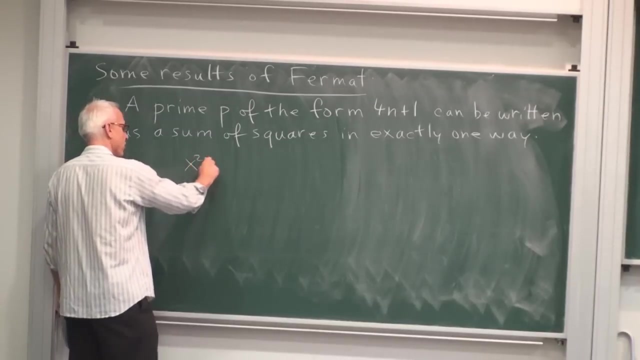 One way, And almost all of these, Almost all of these results Are concerned with natural numbers. We're thinking about equations with natural numbers, And here the motivating equation would have been the Pythagorean equation: x squared plus y squared equals z squared. 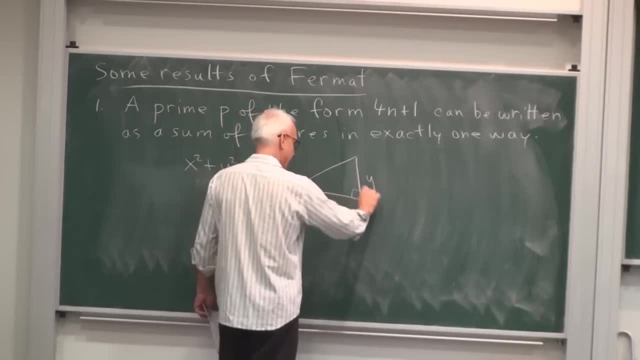 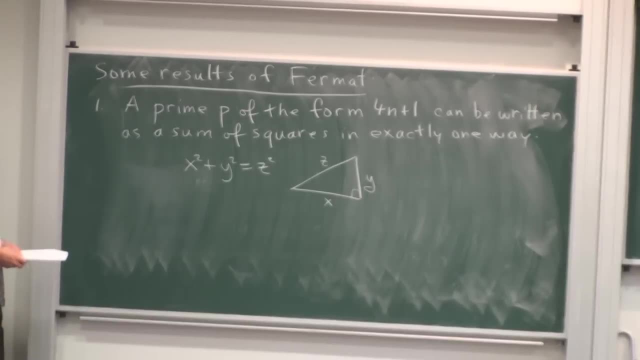 For a right triangle With sides x, y and z, Which, of course, had been studied by the ancient Greeks, And Diophantus knew a lot about this too, So the question is One way of interpreting What this is about. 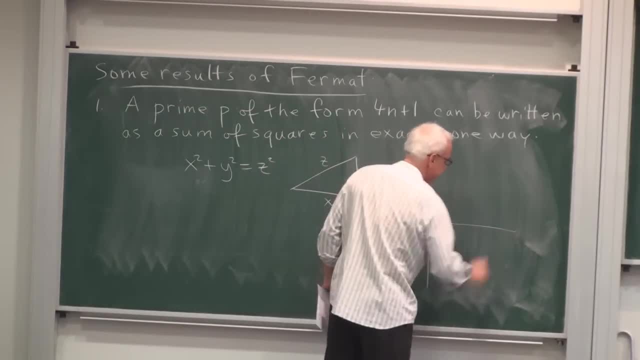 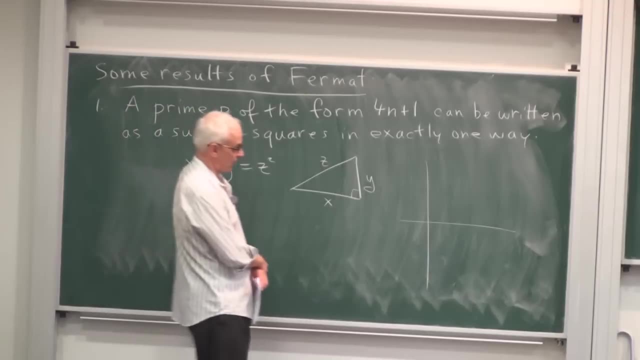 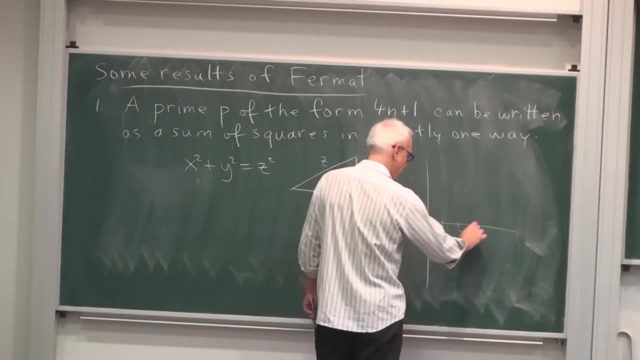 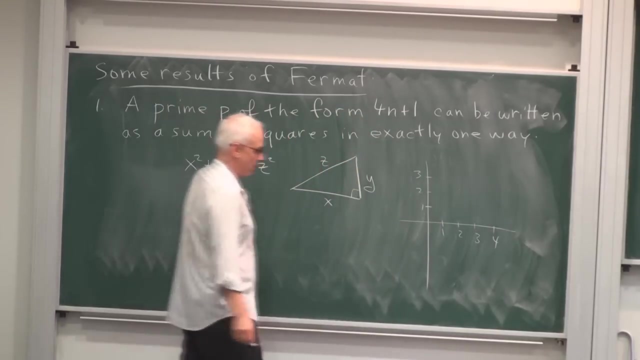 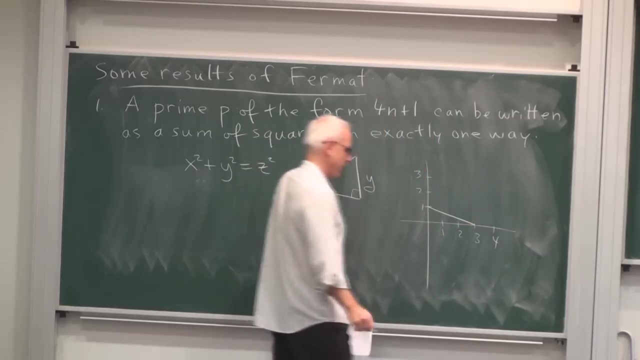 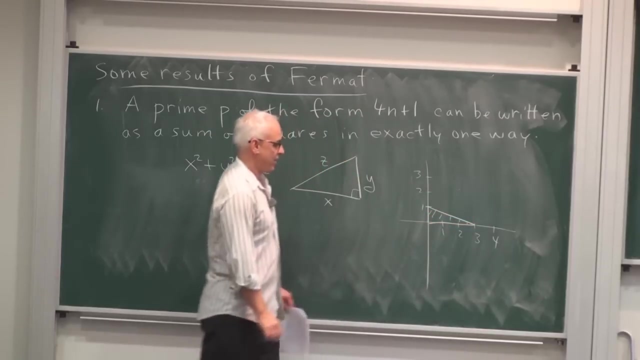 Is to ask Which primes Can be realized as Areas of squares In the integral plane. So if we restrict ourselves to just Integral values, Say positive integral values, And we Cook up A triangle, Say Say that one there. 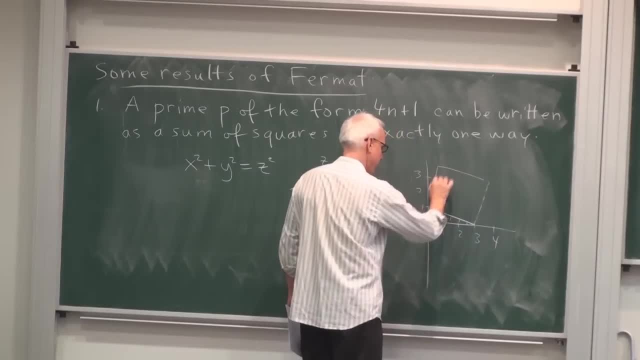 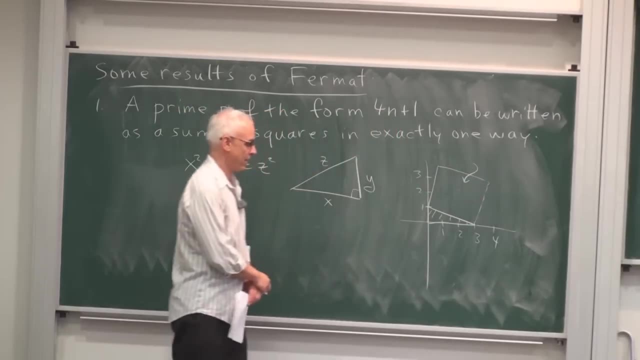 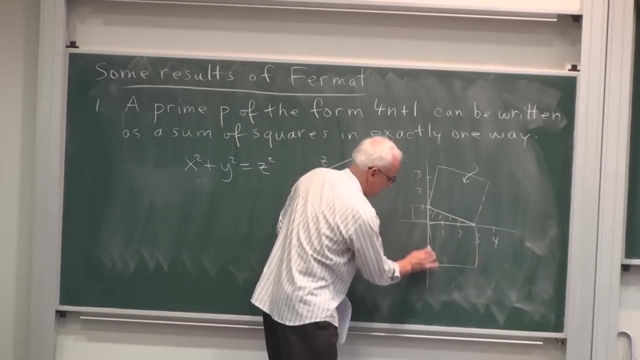 Then you can build On this hypotenuse, You can build a square, And the area of that square will be Well by Pythagoras. it's going to be the area of this square Plus the area of this square, And that's going to be. 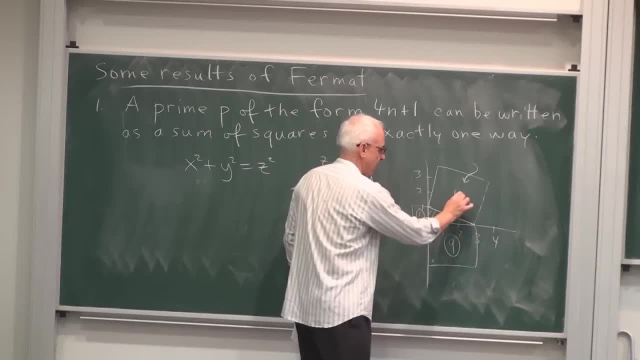 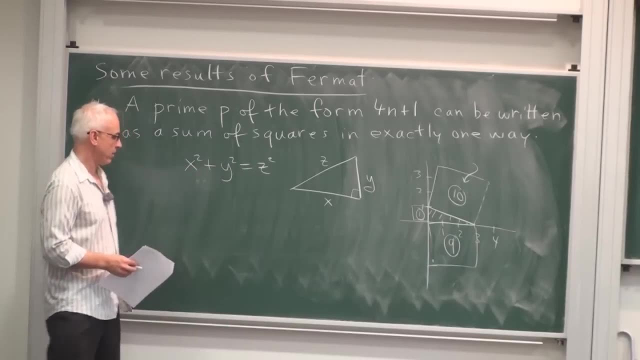 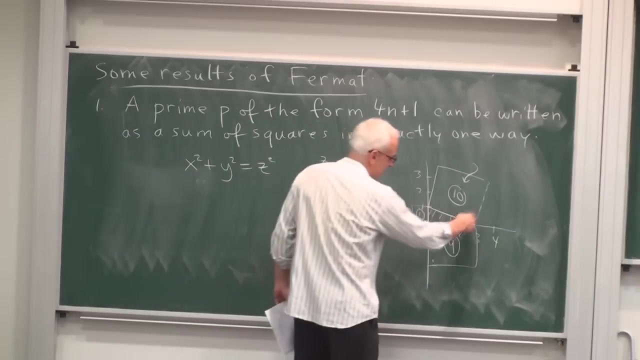 Have area nine And that's going to have area one. So this thing is going to have area Ten. It's a solution. One squared plus three squared Equals One squared plus three squared equals ten. So this is an. This is a. 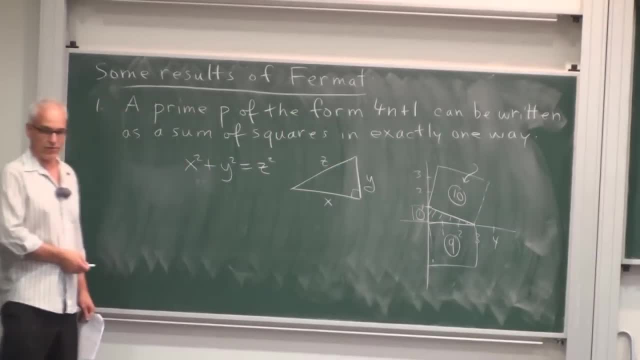 A number Ten can be written as A sum of two squares, And Fermat was interested. Okay, well, let's. Let's say we just restrict ourselves to primes. Which primes can be written As a sum of Two squares? And the answer is the. 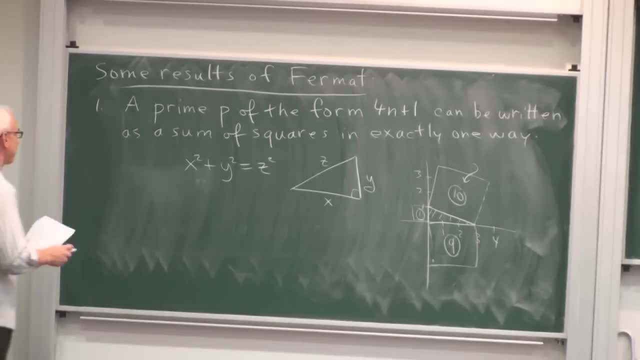 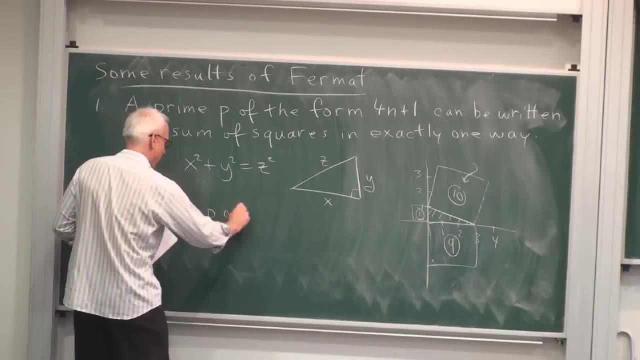 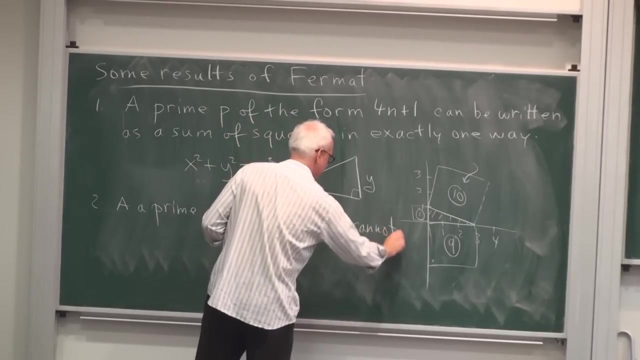 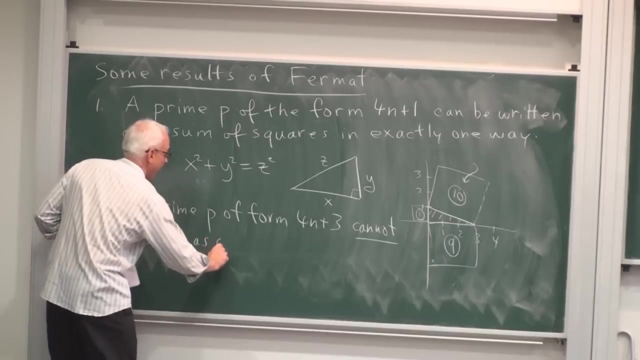 Primes of the form Four n plus one can be written In exactly one way, And our sister result Is that a prime P of the form Four, n plus three, Cannot Be written As A sum Of two. 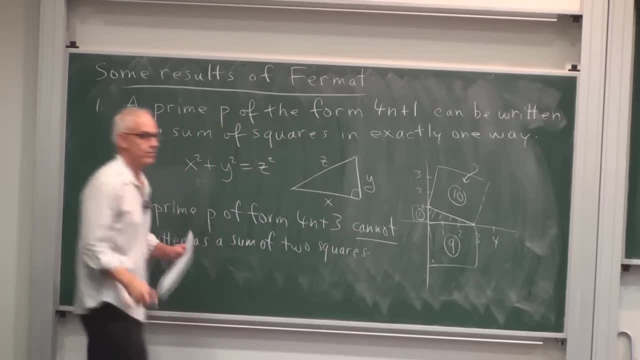 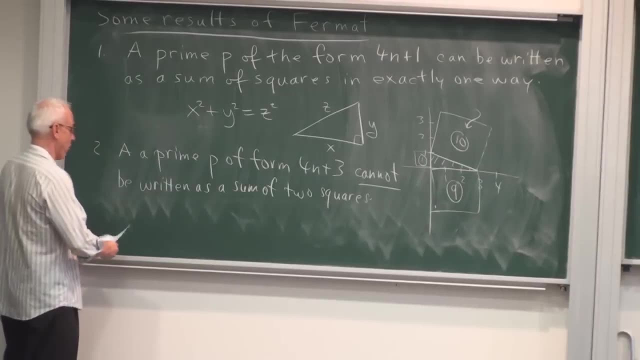 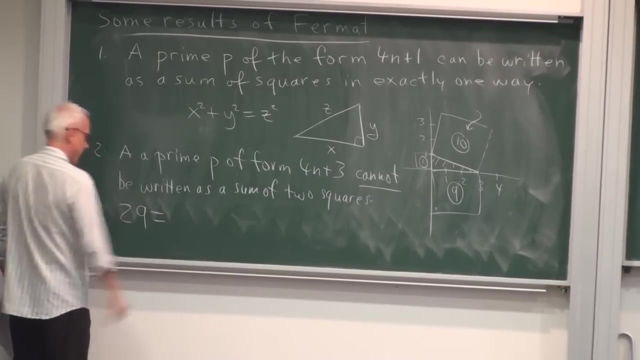 Squares. So, for example, If we take a prime of the form four n plus one, So that's one more than a multiple of four. For example, say twenty-nine, How would we write twenty-nine as a sum of two squares, Five squared plus two squared? 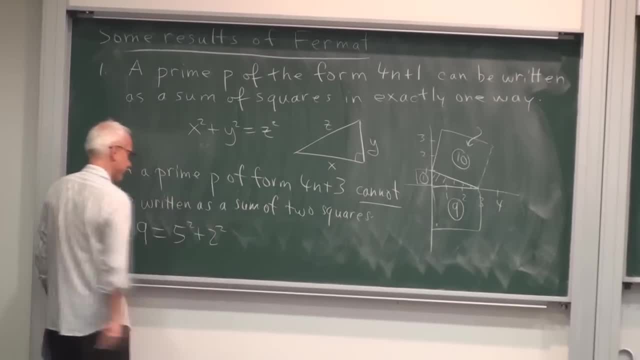 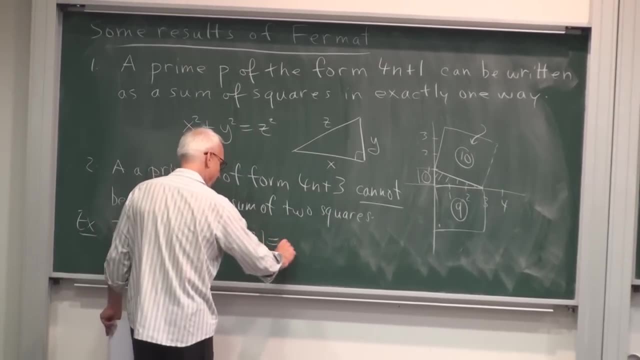 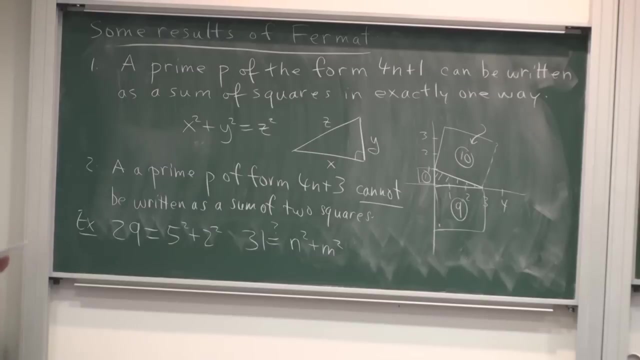 Well, it'd be five squared plus two squared. On the other hand, if we take a prime of the form four, n plus three, For example thirty-one, And we write it, Or try to write it, as n squared plus m squared, Then you can go through all the possibilities. 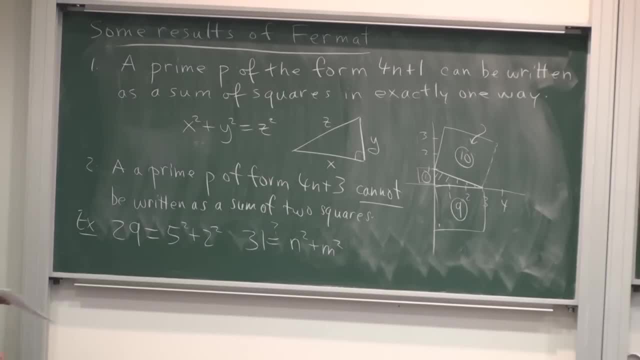 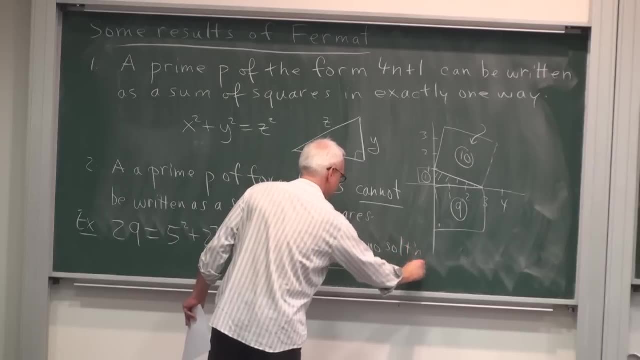 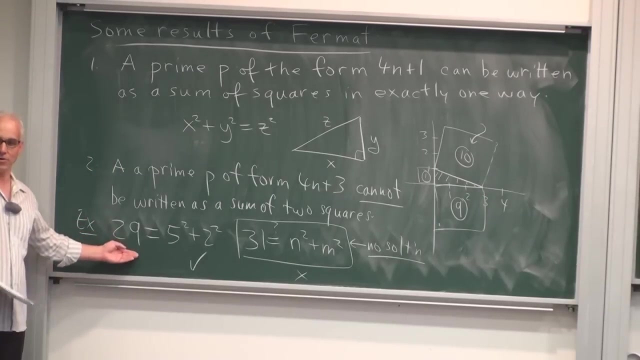 And none of them will work. Okay, So this one? No solution to this one. There is a solution to this one, Not this one, And, interestingly, there's exactly one solution, Even if the prime is very, very big. Yes, 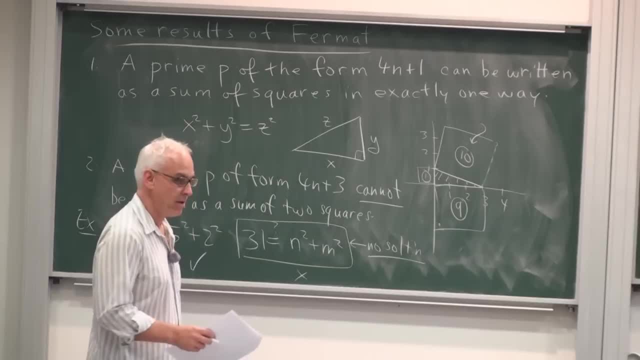 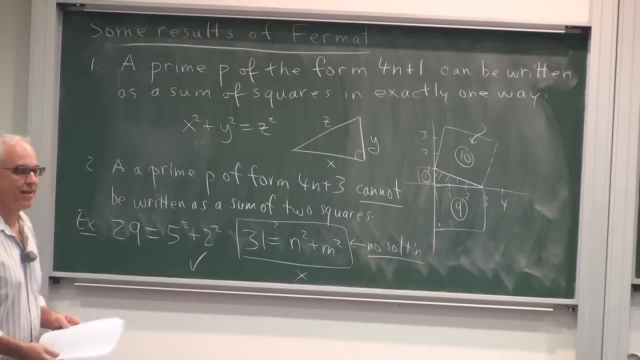 Is it assuming that n and m have to be integers? Yes, So all this discussion is with numbers which are integers. Yeah, Yes, But then the best one is to just use that as well. A sum of two squares. A sum of two squares. 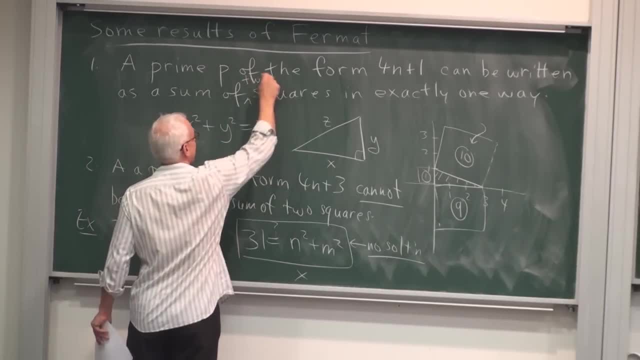 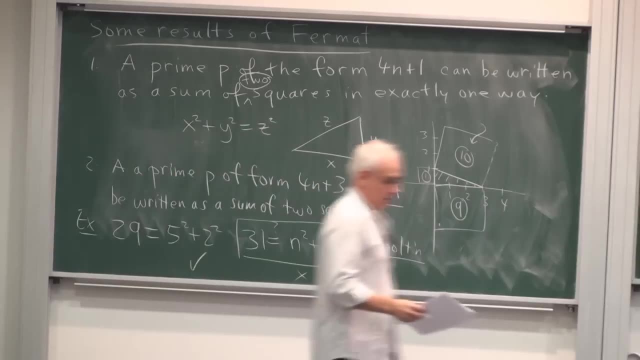 Yes, I didn't write that, Thanks. We're talking about a sum of two squares in exactly one way. Well, he discovered a little bit more in this direction. 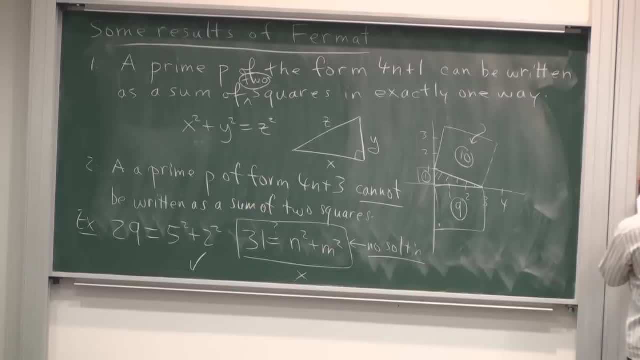 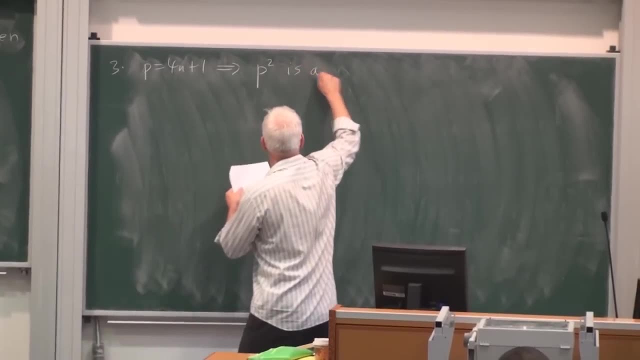 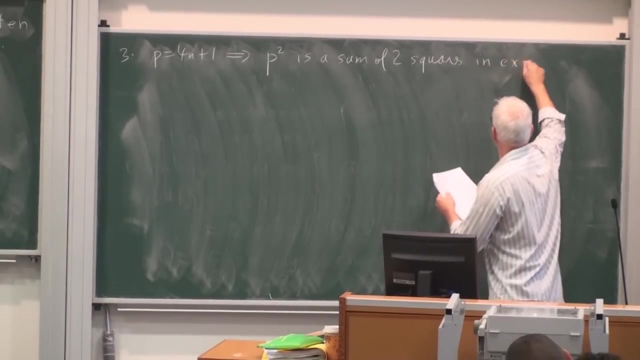 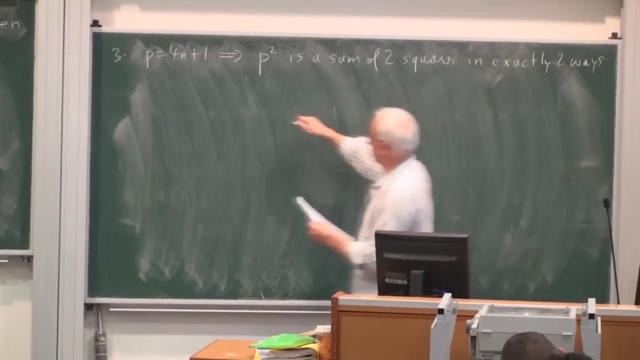 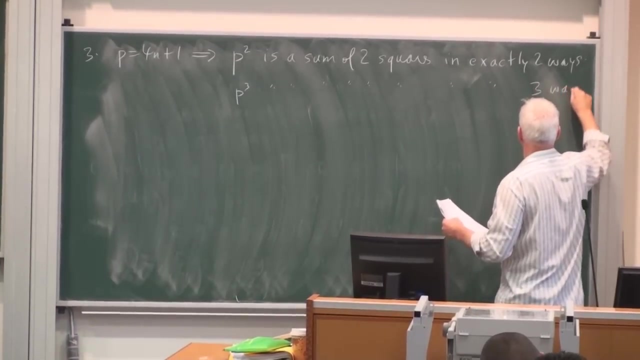 He investigated further and discovered that if p equals four n plus one, in that case p squared is also a sum of two squares in exactly two ways, and P cubed is a sum of two squares in exactly three ways, etc. 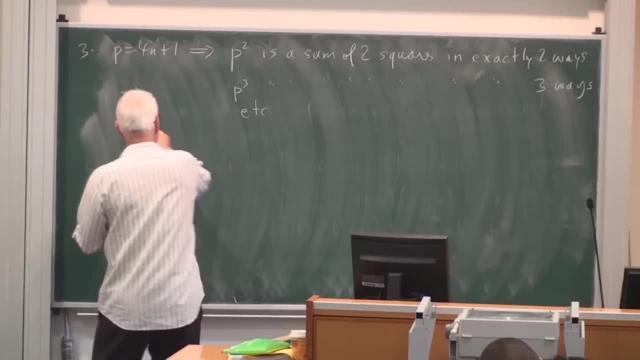 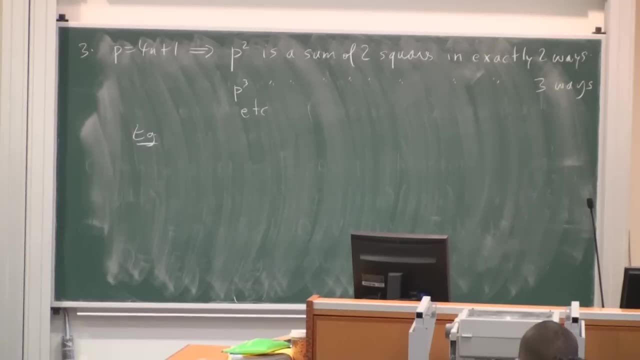 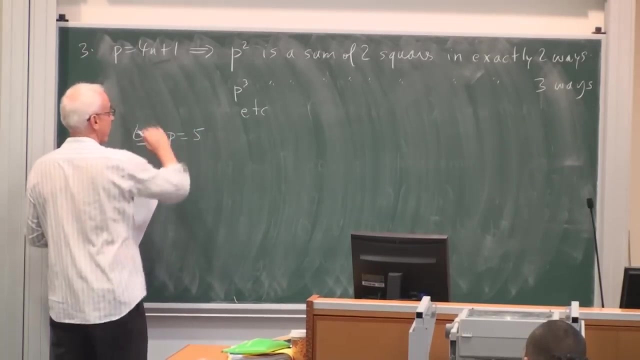 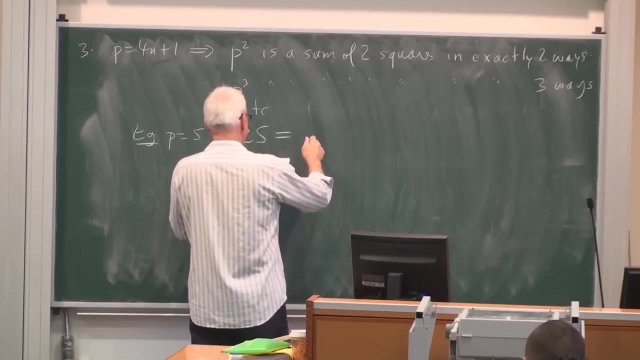 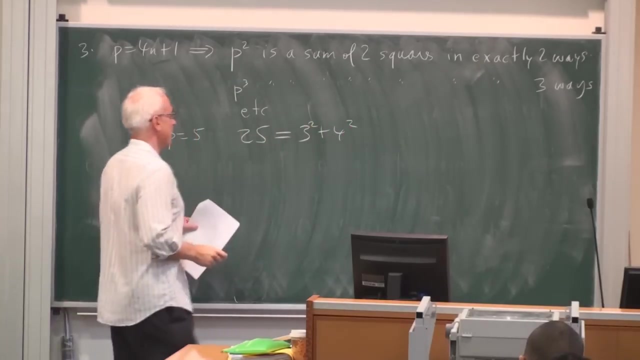 So, for example, the simplest such prime is P equals 5, which is of this form: Then 25 can be written as 3 squared plus 4 squared, So that's 4P squared is a sum of two squares in two ways. 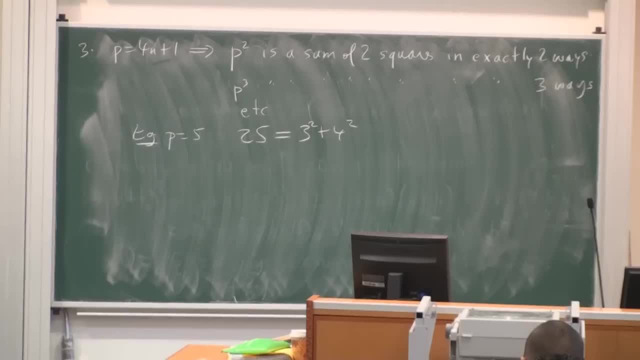 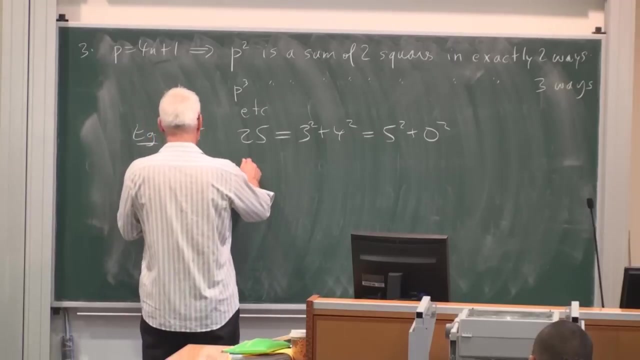 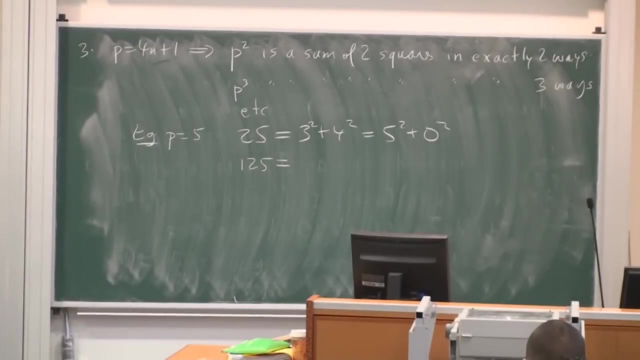 Okay, so What's the other way? 5 squared equals 0 squared. We're allowed to put 0.. And Okay, well, 125.. That's equal to 100 plus 25.. So it's 10 squared plus 5 squared. 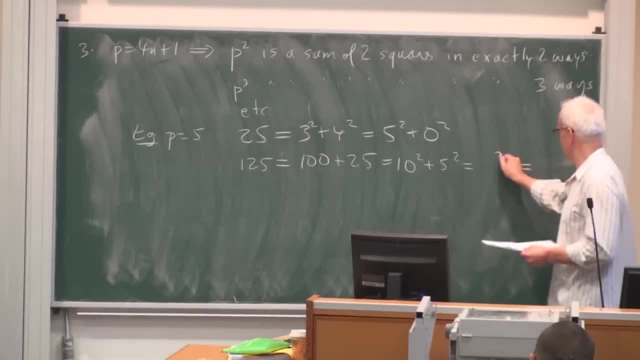 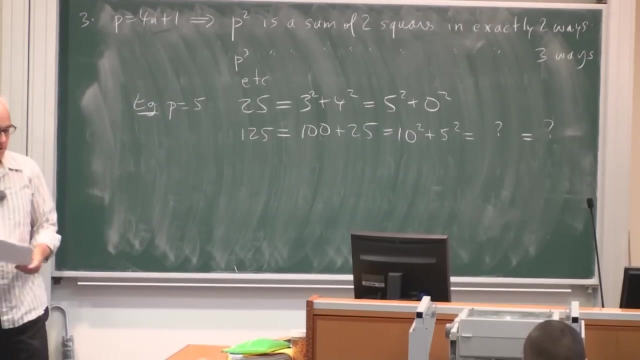 And there's also two other ways. Maybe I'll leave you to try to figure out what they might be. So this became part of a very big theory. just the start, Okay. so there's a very natural question here that the later mathematicians took up. 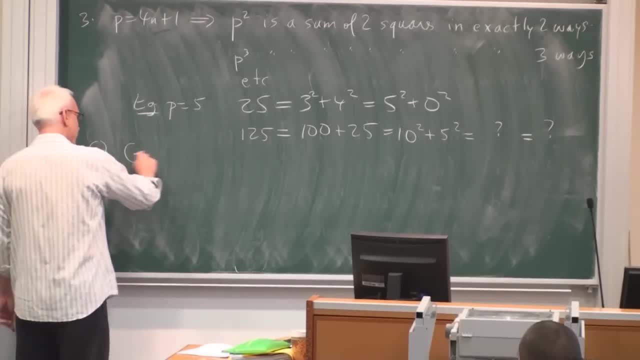 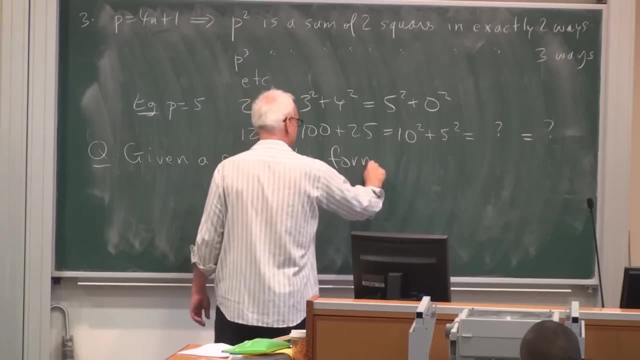 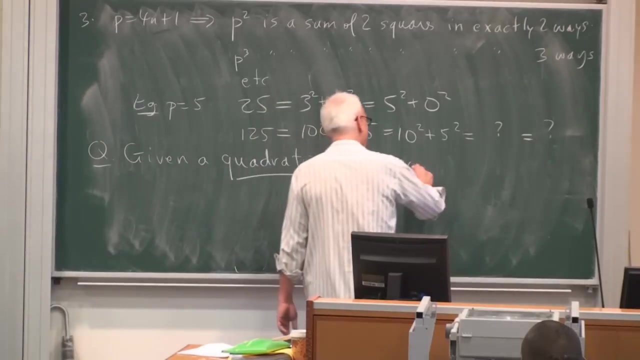 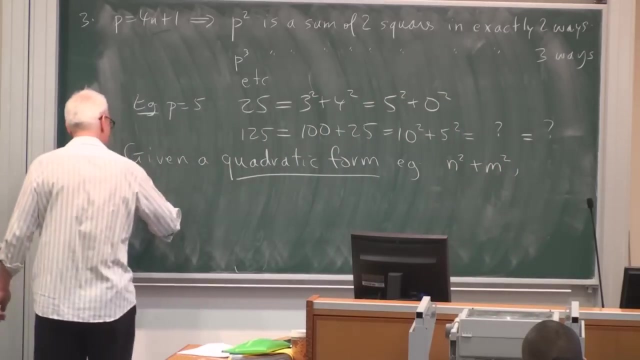 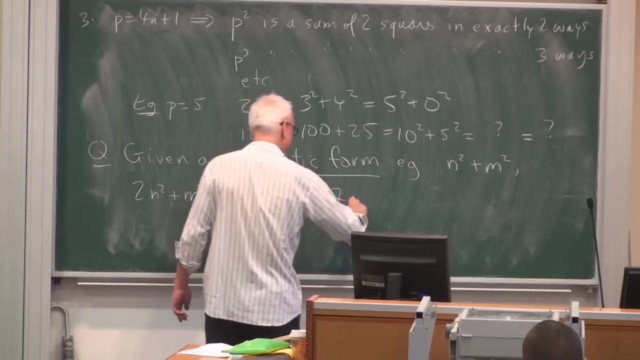 So the very natural question here is: given a quadratic form, Alright, so that's a quadratic expression in two variables. For example, it might be n squared plus m squared, Or it might be 2n squared plus m squared, Or it might be something like 3n squared minus 4nm plus 7m squared. 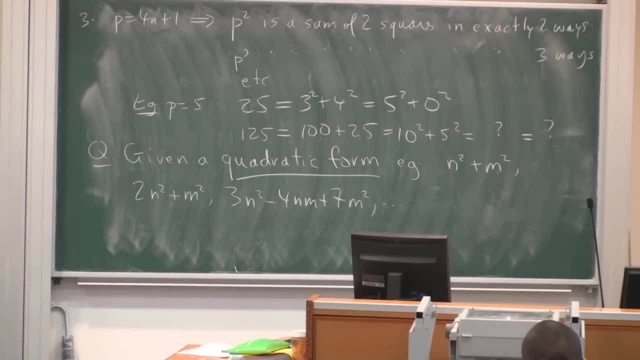 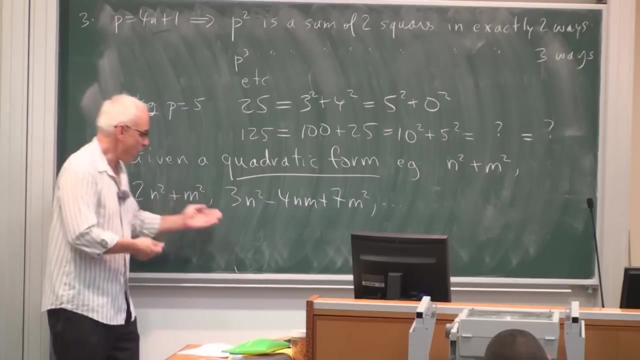 These are all examples of quadratic forms. They're quadratic expressions in two variables, n and m. So, given such a thing, the question is: how can we write a general integer by using this quadratic form in the form of such an expression? 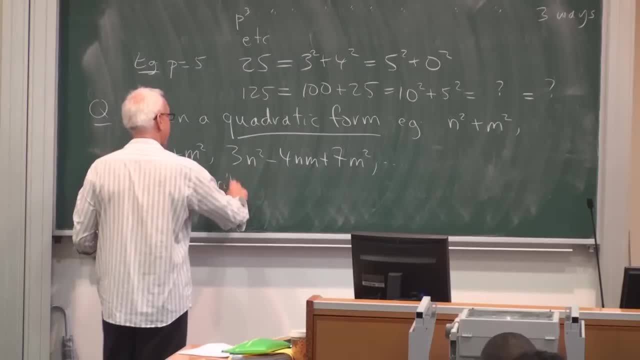 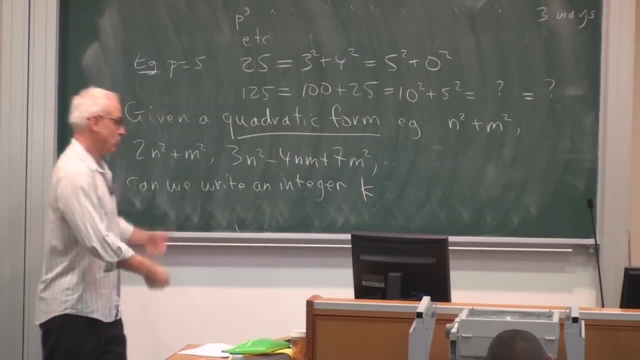 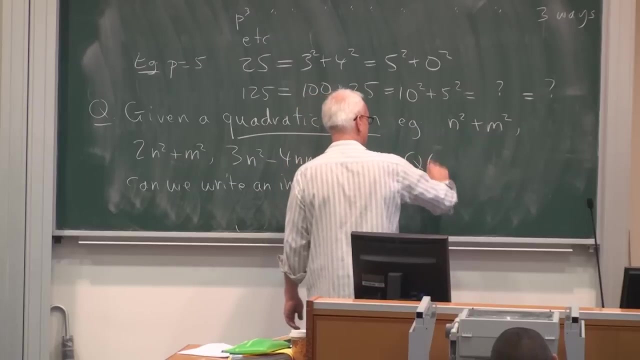 So can we write an integer k, let's say in terms of other integers- n and m- in this form? So let's say the quadratic form is in general qn of m. So the question is, can we write a general integer k? 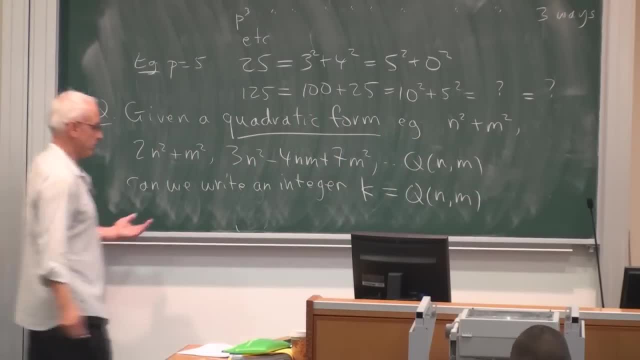 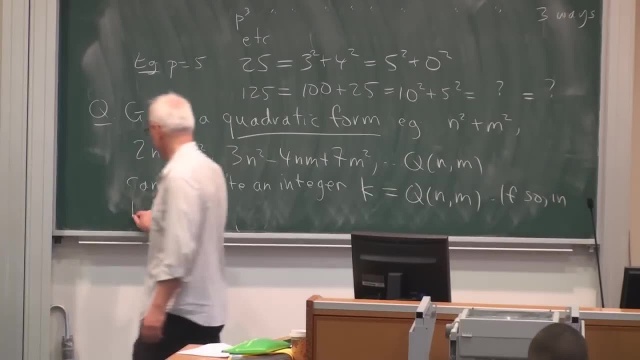 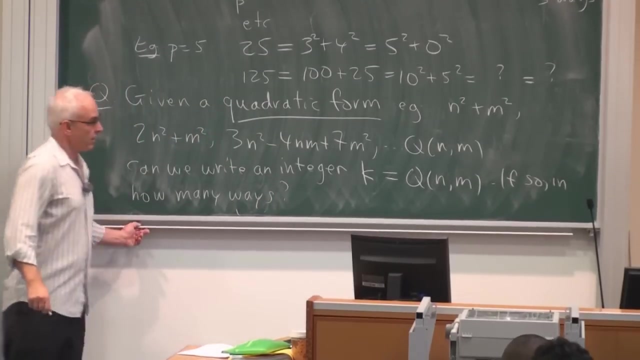 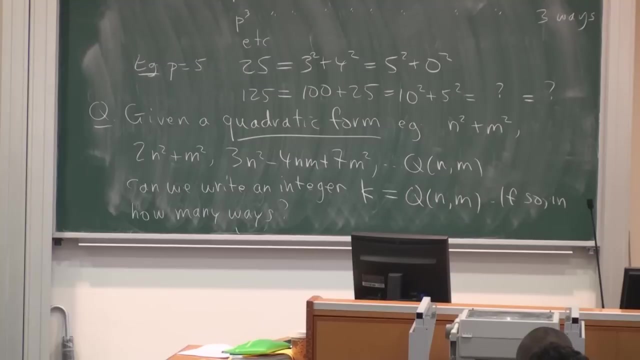 as q of nm, And if so, so that might be yes or no, but if so, in how many ways? So these are sort of very fundamental kinds of arithmetical problems. They're the sort of first hard problems that you get to when you go past the linear problems. 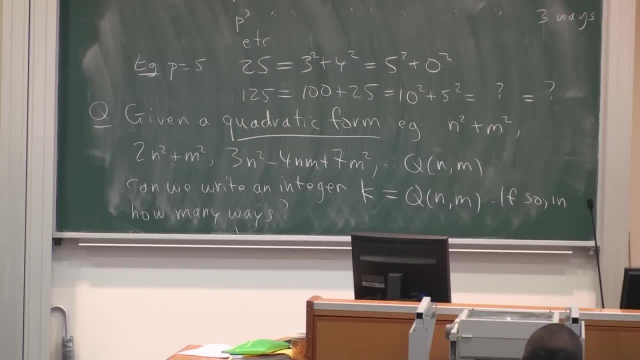 Because they're quadratic. They're essentially quadratic equations, in integers really, So you can write down the quadratic formula, of course. but the question is, when is the thing underneath the square root going to be a square? So it's a number theoretical question. 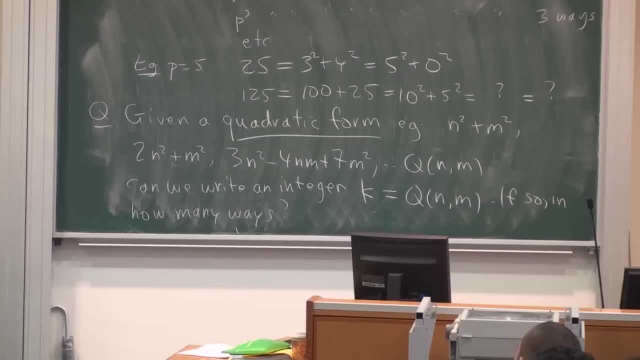 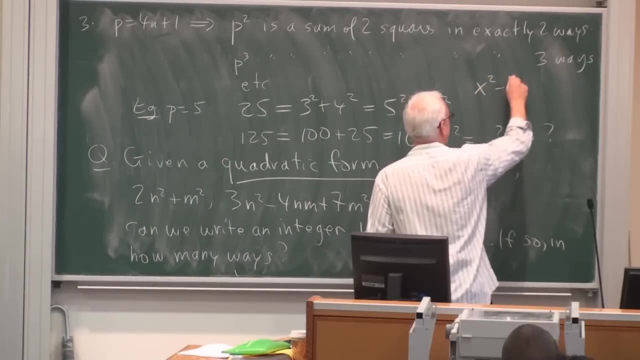 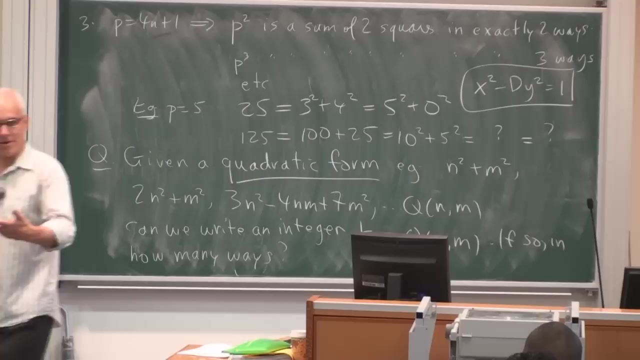 Of course, examples of this kind of thing had already been discussed in antiquity. We've already talked about Pell's equation, where you have x squared minus dy squared equals 1.. Where d is some number that's chosen in advance which is not square. 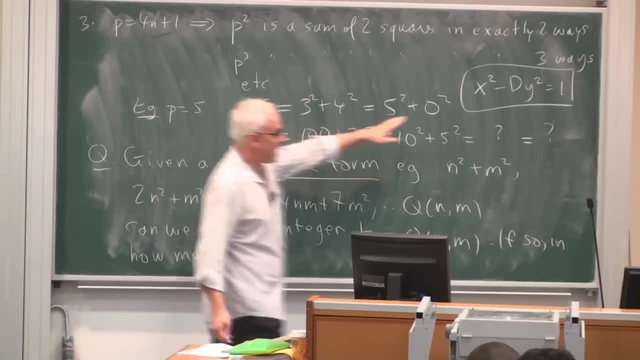 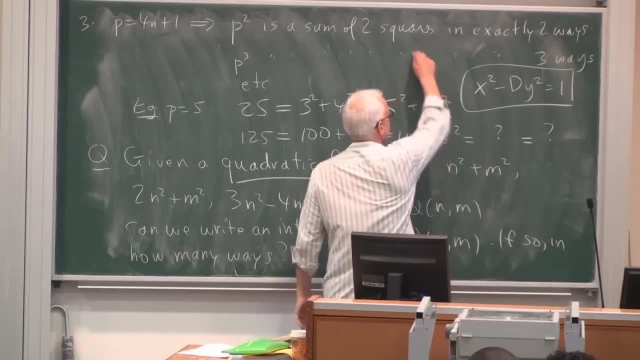 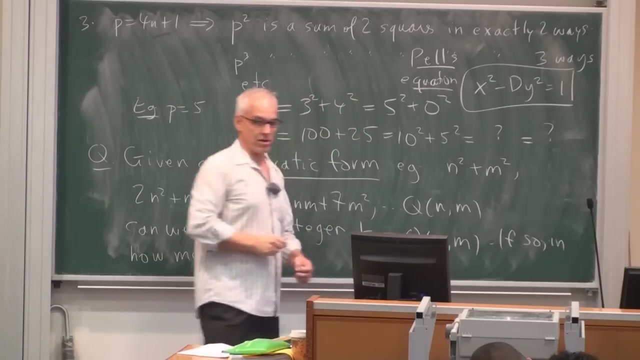 That's an example also of such a kind of thing. We're asking in this case: how does one write 1 as an expression involving this quadratic form? So this kind of equation had been around for quite a long while in terms of Pell's equation. 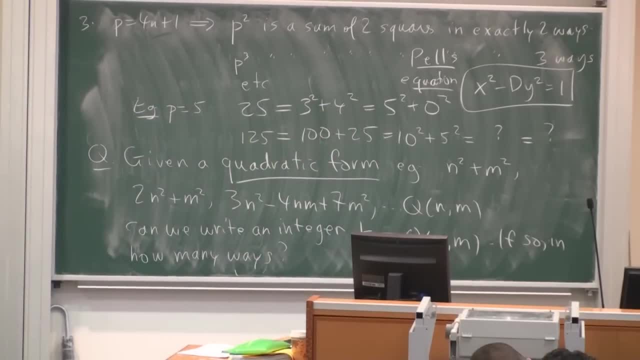 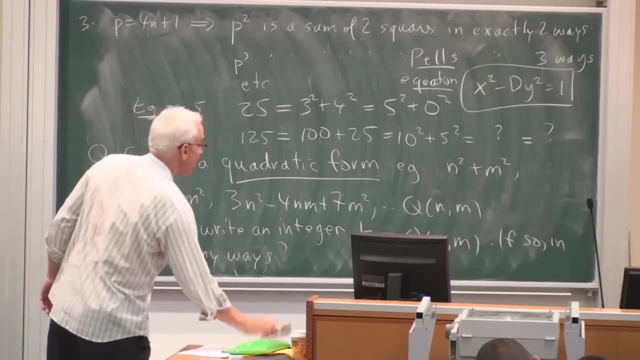 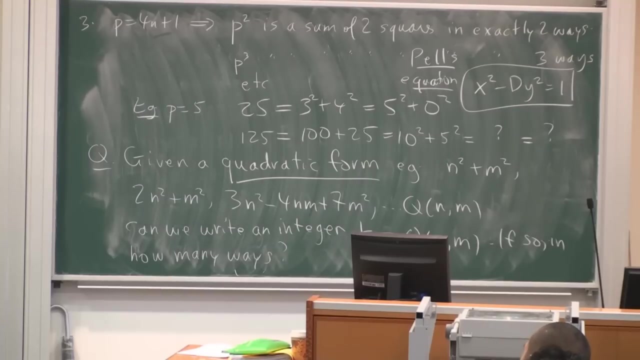 But Fermat realized that there was actually a much more general set of questions, Questions that one could ask. In fact, Fermat was quite interested in Pell's equation and did some work in that, And one of his claims was that if d was not a square, 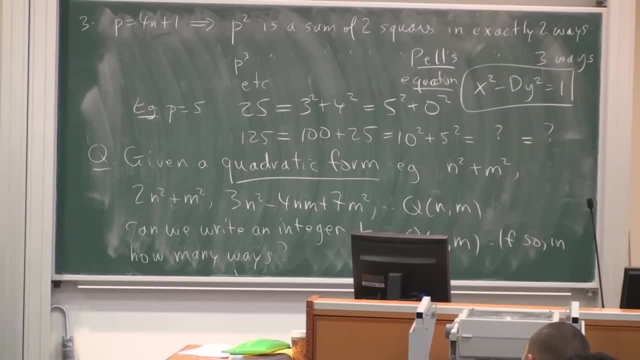 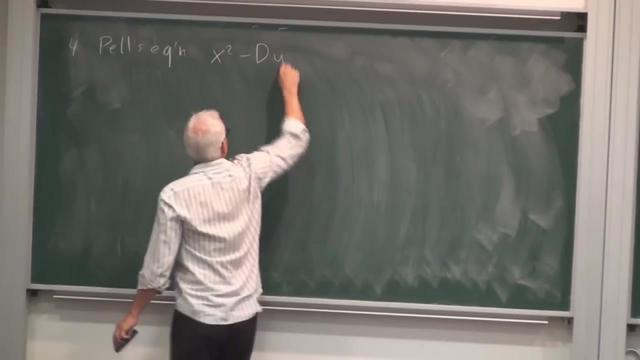 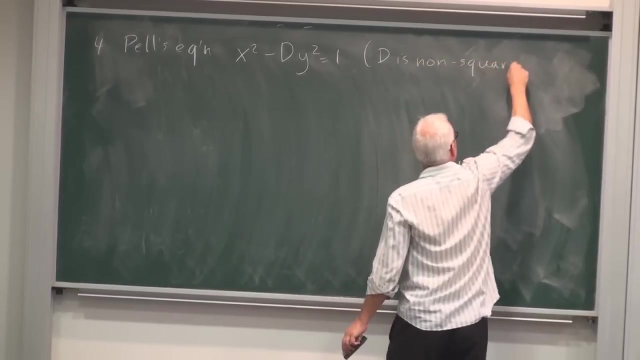 that such an equation always had an infinite number of solutions. So I suppose maybe this is the fourth thing. Fermat claimed that the Pell's equation, x squared minus dy squared, equals 1,, where d is a non-square, has an infinite number. 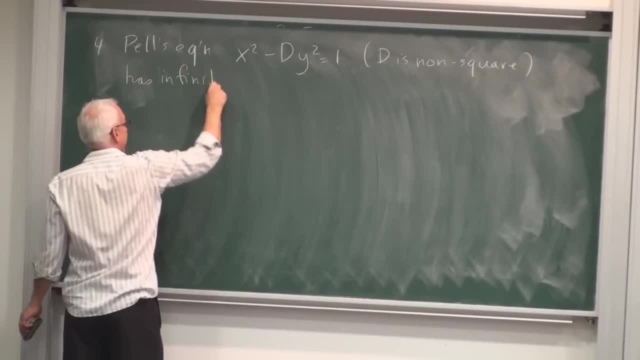 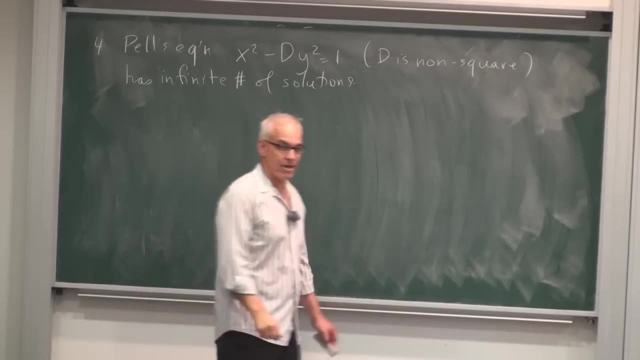 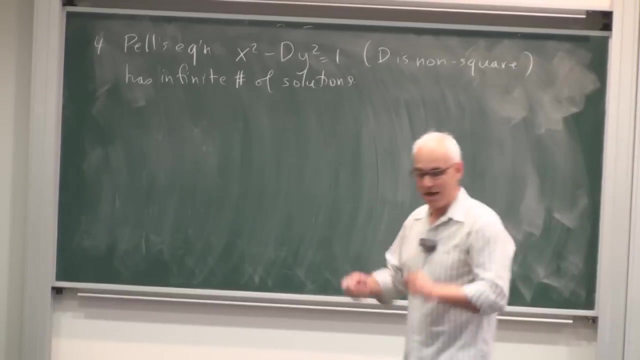 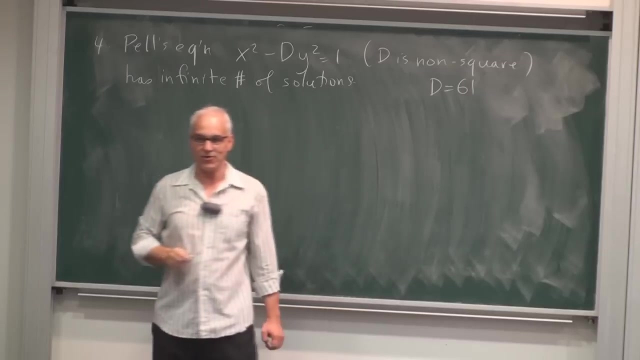 of solutions. He claimed this in letters and he posed this as a problem to fellow mathematicians, to English mathematicians, And he was well aware that there were certain values of d that were particularly hard. For example, d equals 61,. 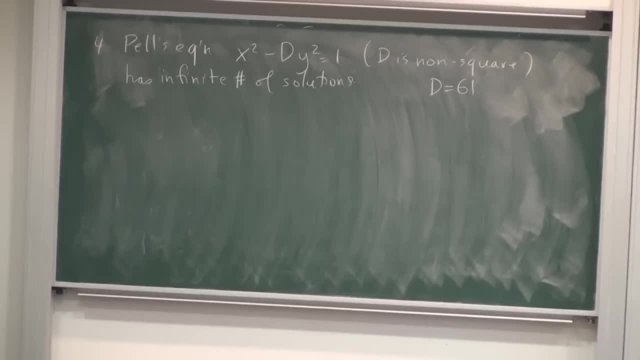 where the solutions, the smallest solutions, are already pretty big and not likely to get to it via trial and error. So he made this claim that there was an infinite number of solutions, but in fact the proof of that was that there was always a solution. 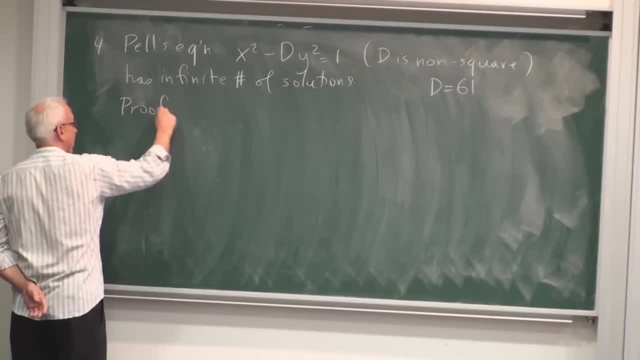 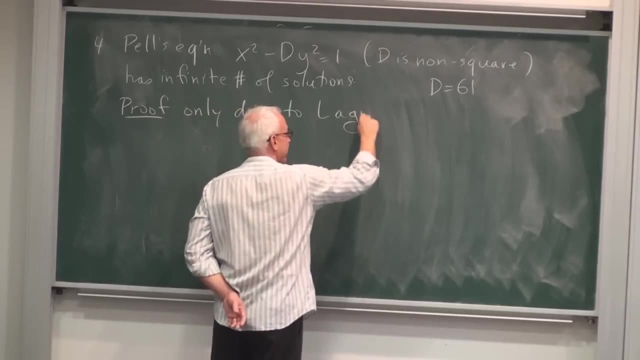 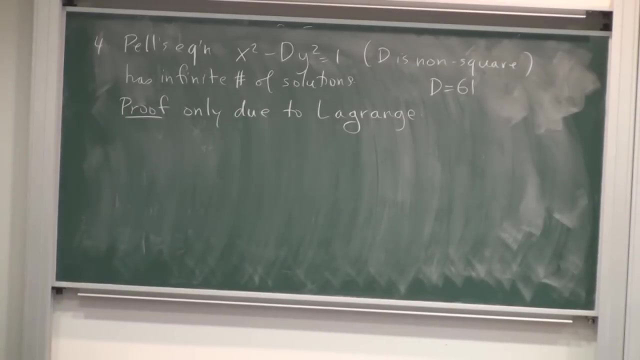 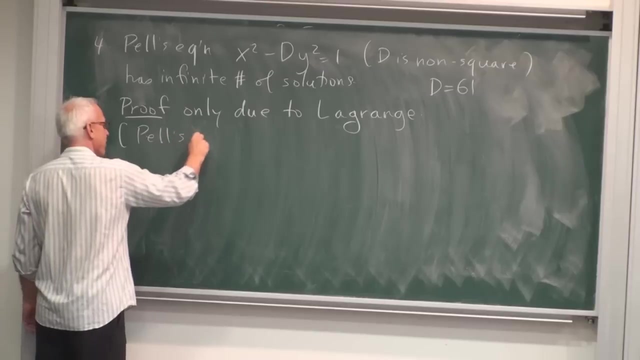 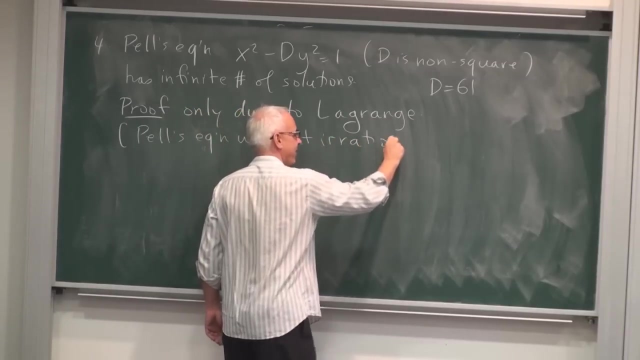 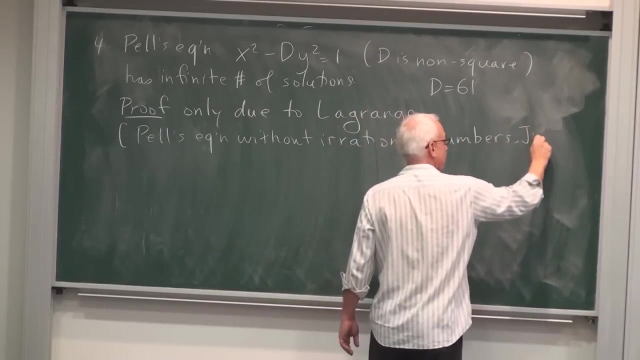 But if there was an infinite number of solutions that had to wait for Lagrange Proof, only due more than 100 years later to Lagrange? This is a subject that has interested me on occasion and I've written a little paper called Pell's Equation Without Irrational Numbers, which appeared in the Journal of 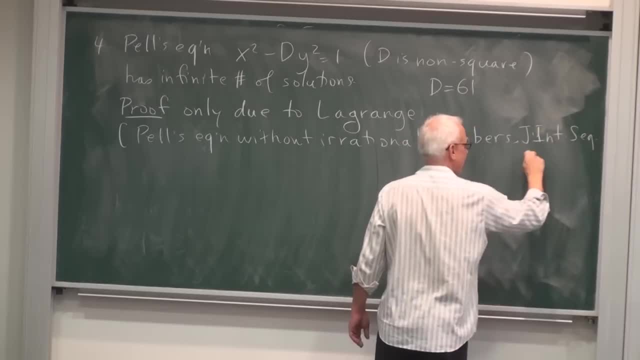 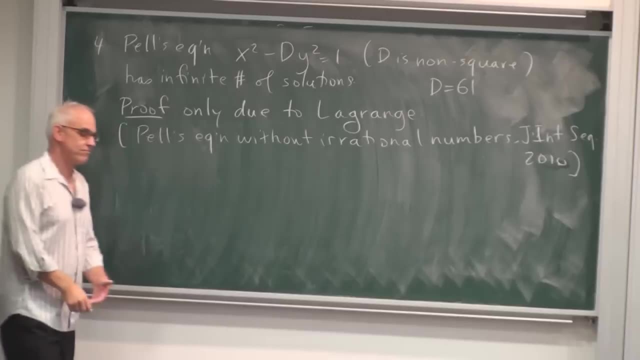 Integer Sequences just in 2010.. And in this paper I give what I think is probably the simplest proof of this fact: that there's an infinite number of solutions to Pell's Equation. So it's very elementary proof that you can have a look at. It just requires some first-year understanding. 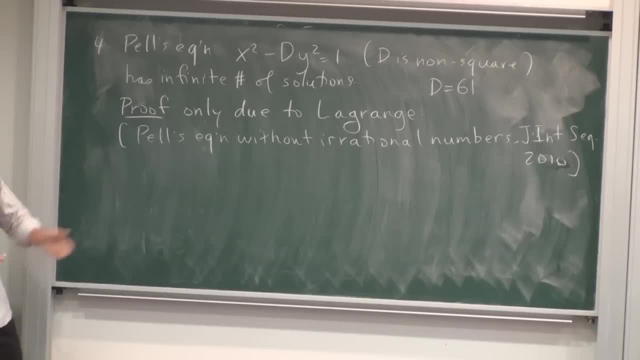 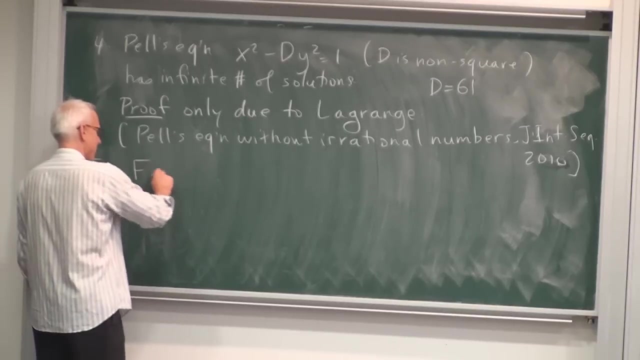 of linear algebra. You can find it on the internet if you like. What other kinds of things was Fermat interested in? He was interested in prime numbers and he investigated the question of: is there some formula for prime numbers? Many people have. 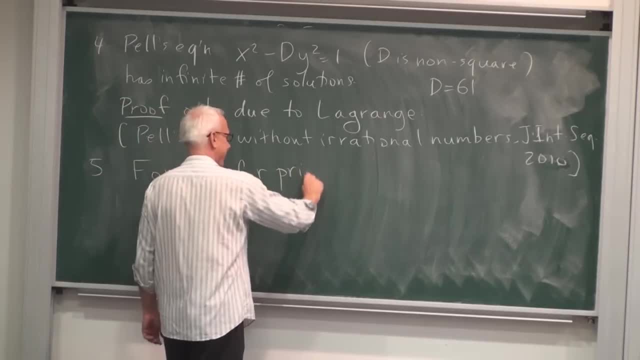 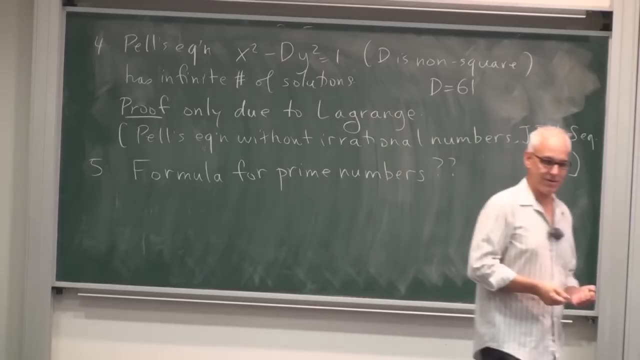 searched for a formula for prime numbers, and there probably are lots of people today who are looking for a formula for prime numbers, some formula that will guarantee you a prime number, But no such formula is known. There's a maximum prime that's known and that's a. 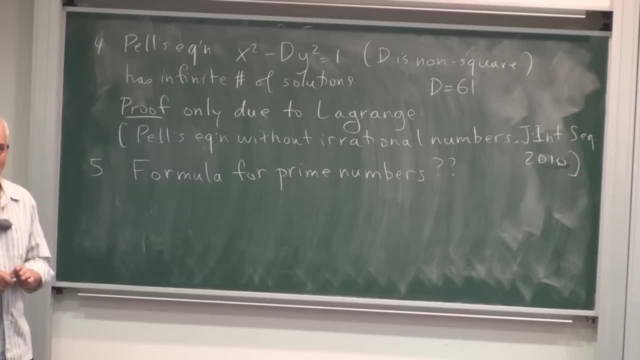 record that has stood for a long time. So I'm going to give you a little bit of information. So I'm going to give you a little bit of information. So if you've been looking for a prime number for three or four years now, it's hard to come up with bigger and bigger primes. But 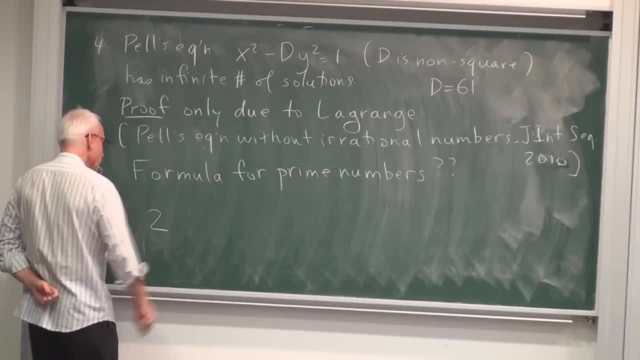 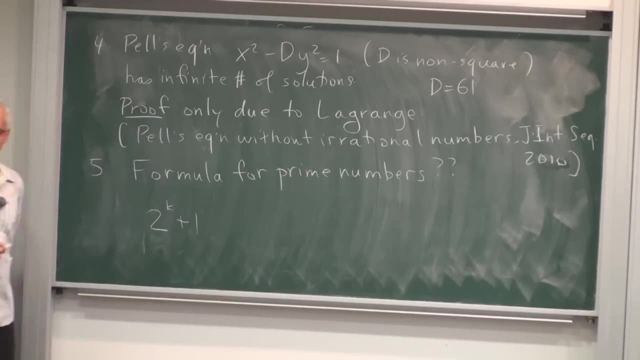 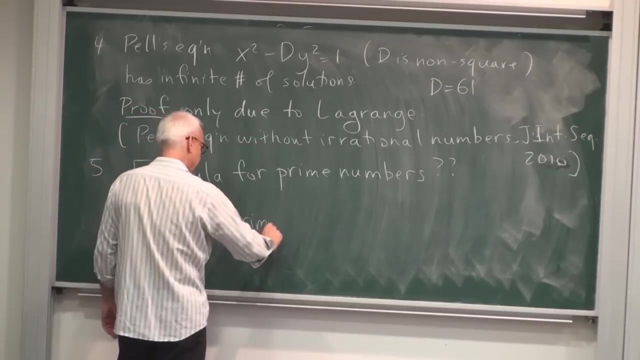 Fermat's idea was that we should look for a prime of the form 2 to the k plus 1.. We've talked about 2 to the k minus 1.. 2 to the k plus 1 is prime. It's not too hard to see. 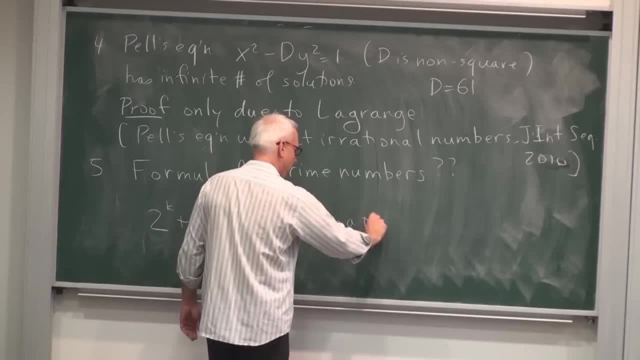 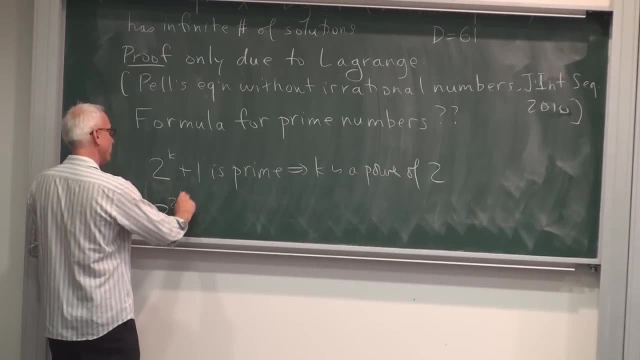 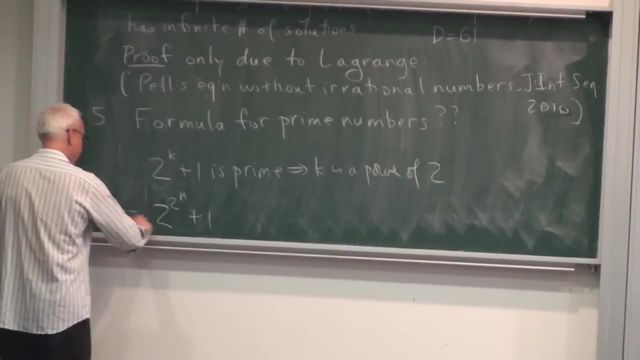 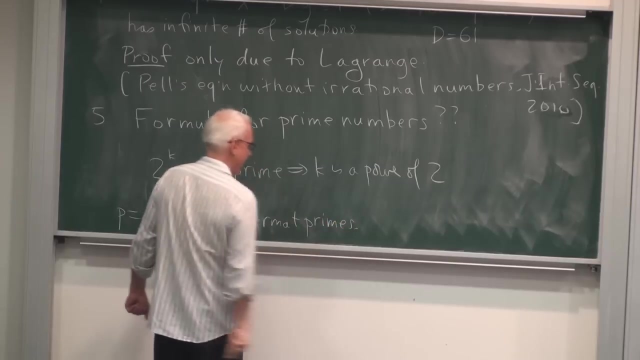 if it is prime, It means k is a power of 2.. So, in other words, we're actually talking about something in the form 2 to the 2 to the n plus 1.. Primes of this form are called Fermat primes, And it's known that they are. 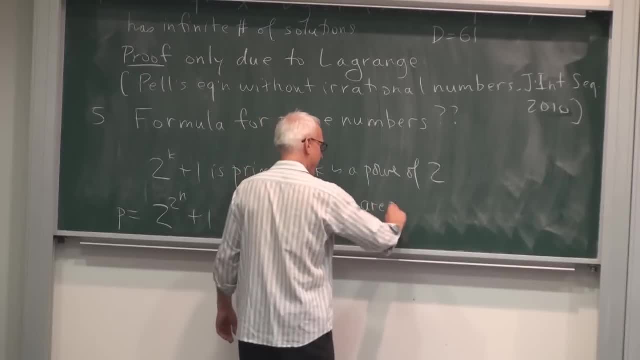 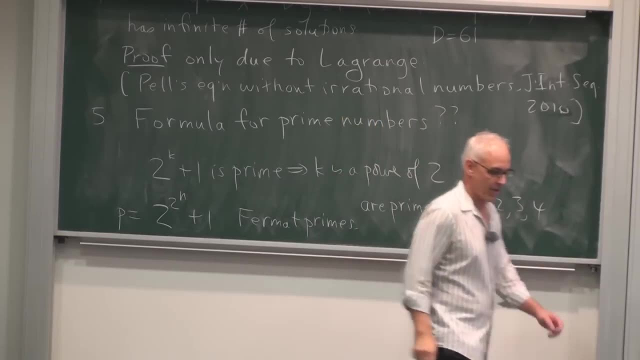 prime. They are prime for the first five When n is equal to 0,, 1,, 2,, 3, and 4.. And when n is equal to 0,, 1,, 2,, 3, and 4.. And those primes are: 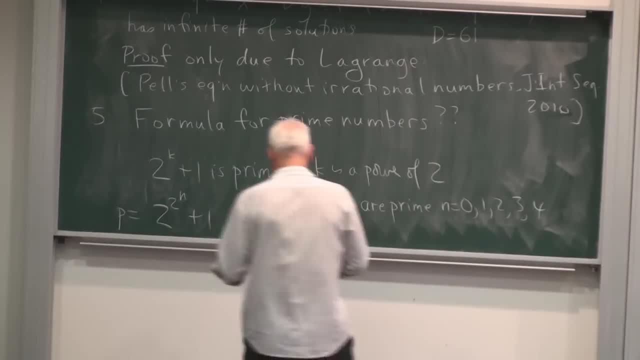 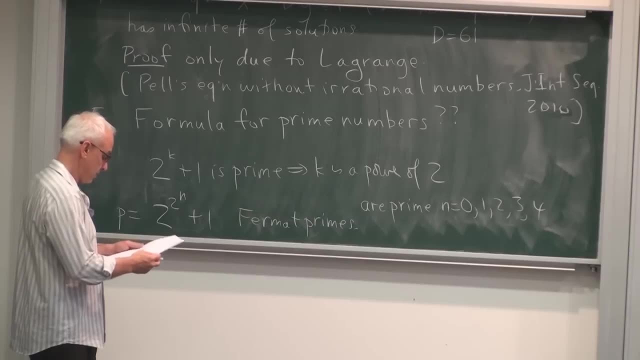 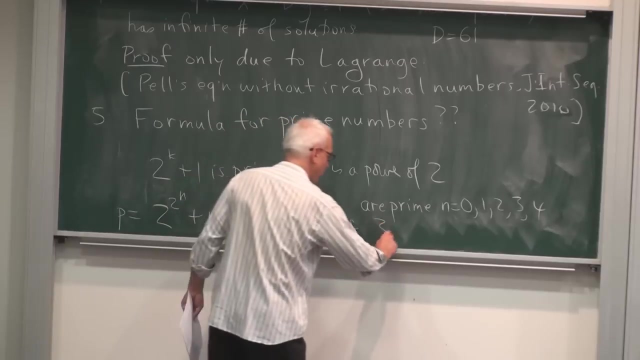 I thought I had it. I guess I don't. Well, the first one: when n is 0,, we get 2 to the 1 plus 1.. So that's 3.. That's one of them, And then the next one is 5.. And the next one: is 6. And the next one is 7., And the next one is 8. And the next one is 9. And the next one is 10. And the next one is 11. And the next one is 12. And the next one is 12.. And. 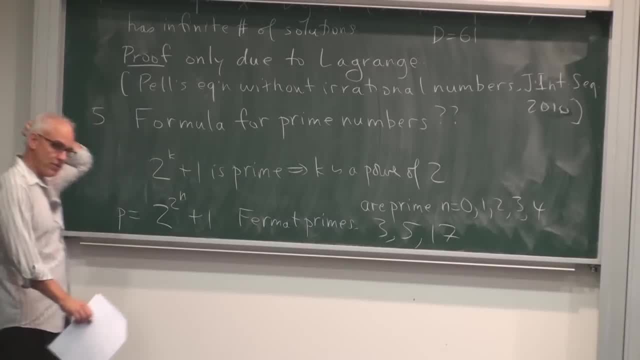 the next one is 17.. And then there's two more which I don't know offhand, When n equals 3 and when n equals 4.. And they are in fact prime. And so Fermat claimed that in fact this formula works for any n. You stick any n in and you get a prime number. 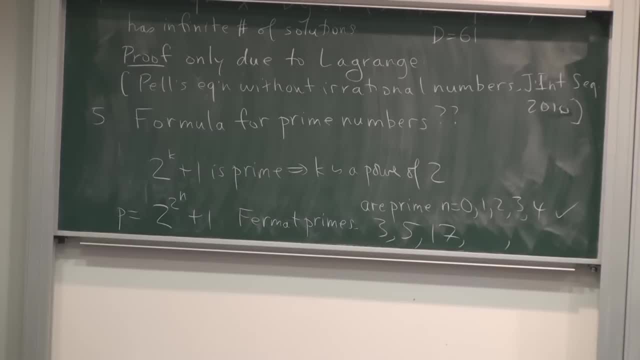 But there's reason to believe that he was doubtful about this later on. Okay, In fact, that claim is false. The next one in the list is, in fact, not prime, But it's not so easy to figure that out. Thank you. 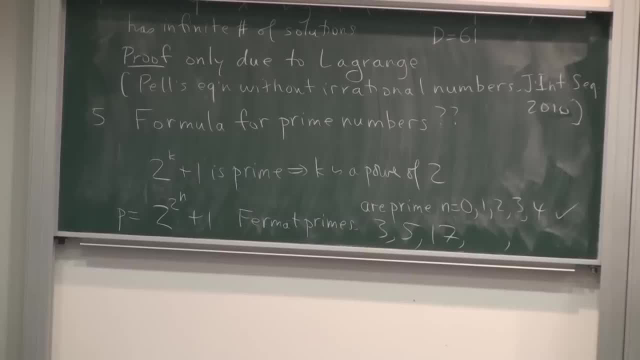 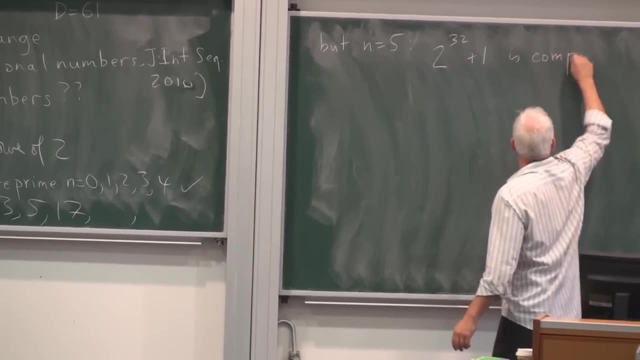 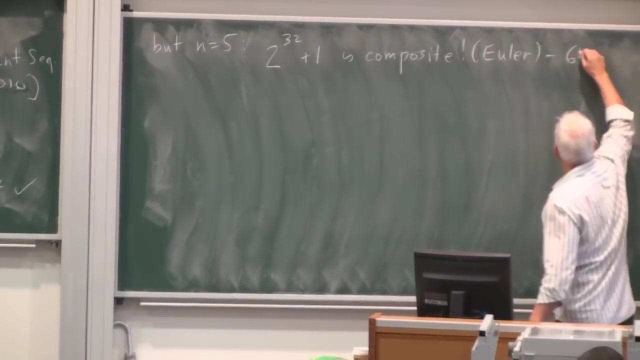 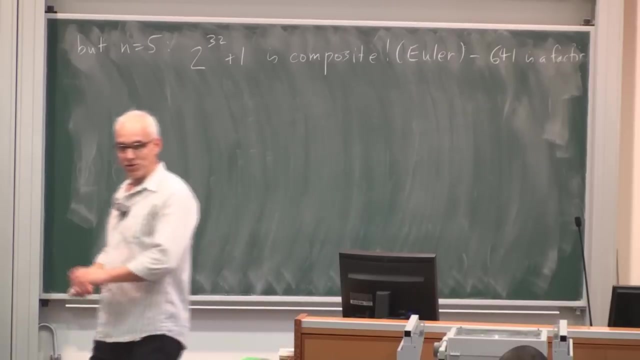 So those numbers are prime, But n equals 5, we're talking about 2 to the 32 plus 1, is composite, And that was discovered by Euler, who discovered that 641 is a factor. Now you can be certain that Euler did not use his calculator to figure that out. 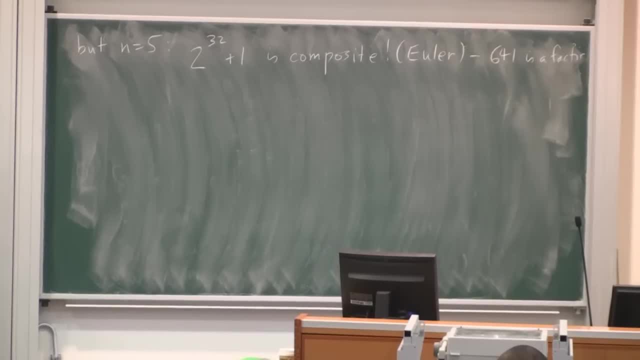 So Euler would have calculated that. He would have calculated 2 to the 32 plus 1. And he would have set about trying to see whether it was composite. And pretty well, the only way he would have done that is to start dividing it by primes. 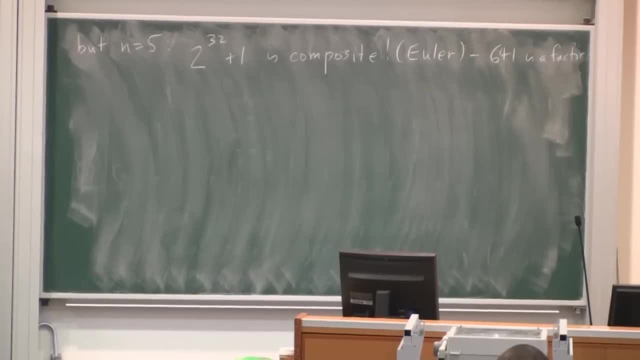 Divide it by 5, or it's not obvious if it's not 7.. Go through all the primes and divide it each time and see if you get something where it divides. And once you get to 641, you find that it does actually divide. 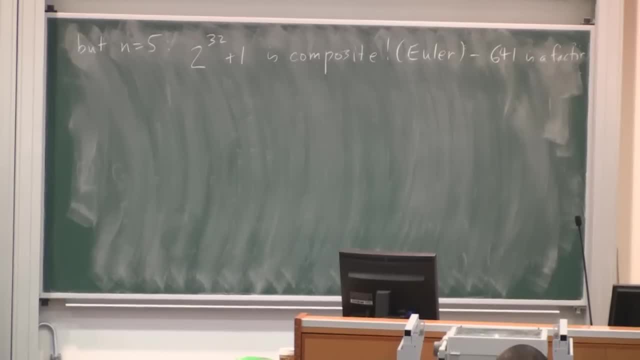 That tells us a lot about Euler Right. This is the greatest. This is the greatest mathematician of modern times, And he's not averse to spending his time this way. He does not mind making a calculation, saying: OK, it's early morning, I'm going to compute this thing all day. 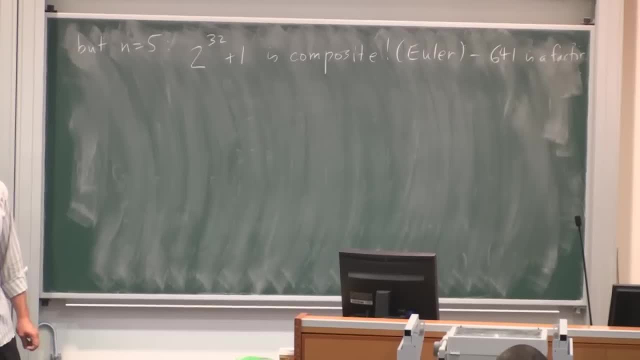 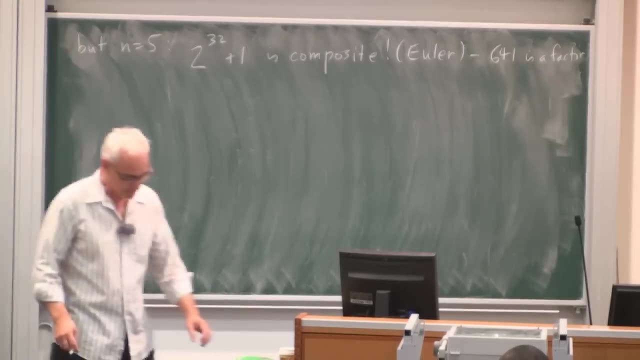 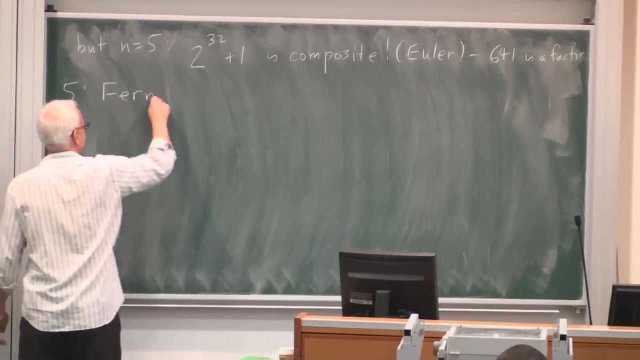 See how far I get. Maybe that's one of the reasons why he's the greatest mathematician of modern times. Thank you, Fermat's most famous result. No doubt you all know about Number 5.. It used to be called Fermat's Last Theorem. 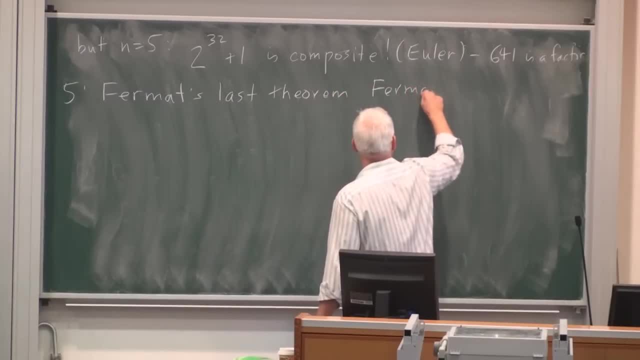 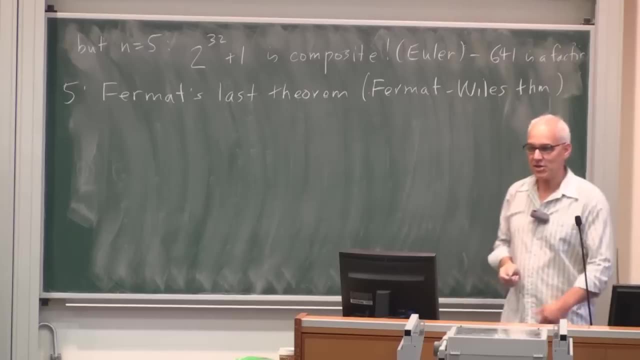 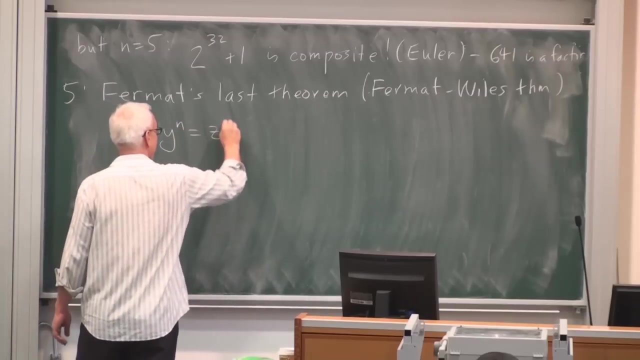 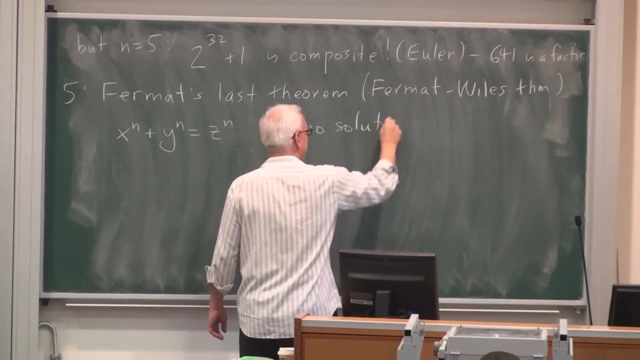 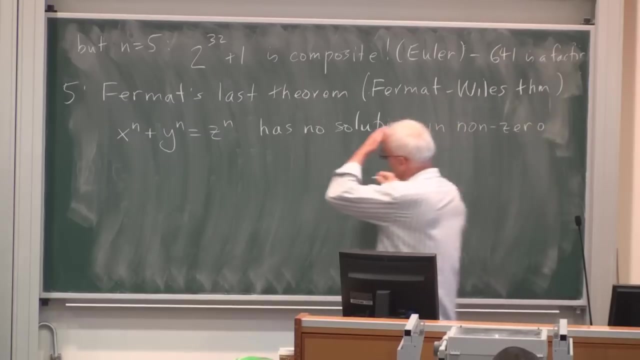 But now it's often called Fermat-Weil's Theorem, And this is a famous result that says that the equation x to the n plus y to the n is the same. N equals z to the n- has no solutions in non-zero integers if n is bigger than 2.. 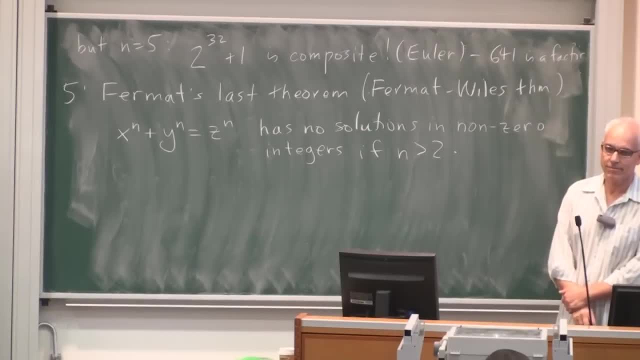 Number 5.. It used to be called Fermat's Last Theorem, But now it's called Fermat's Last Theorem And this is the greatest mathematician of modern times. It used to be called Fermat's Last Theorem. But now it's also called Fermat's Last Theorem And we get the answer, Of course, with n equals 2, there are many solutions And in this equation we have n equals 2.. And we have n equals z to the n has no solutions. 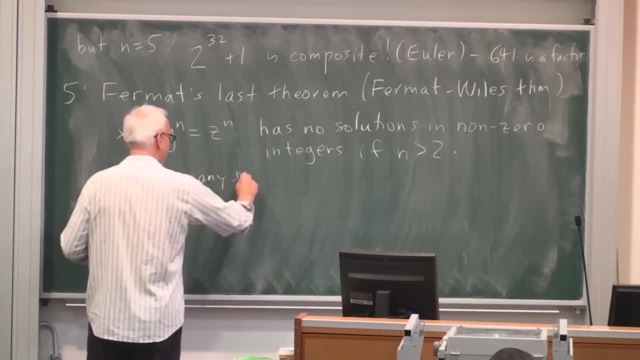 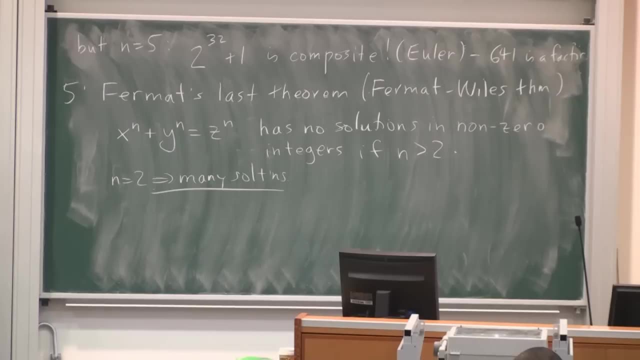 all the Pythagorean triples, but for n equals 3 or n equals 4 or n equals 5 or, in fact, any larger integer, n natural number n, there are no solutions, and the famous story that you've no doubt heard is that Fermat 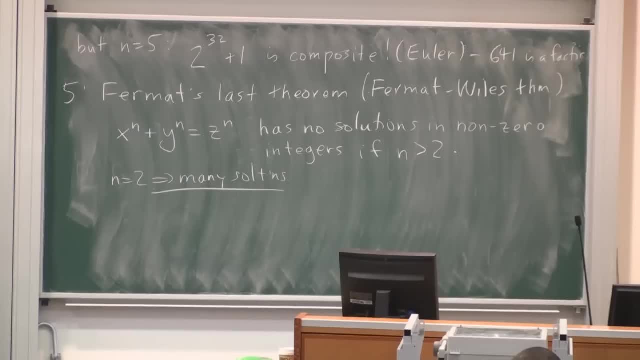 who was reading Diophantus' book. in the margin of that book, in the section in which Diophantus was talking about this kind of problem or something related, Fermat wrote: I have discovered the fact that this thing has no solutions, and I have a marvelous proof of this result, which. 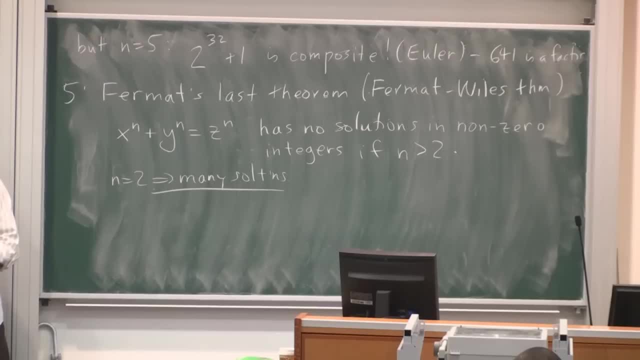 this margin is too narrow to contain and that little comment has sparked huge amount of work, as all important subsequent mathematicians tried hard to prove this result, to discover the proof that Fermat supposedly had. so Euler tried, Lagrange tried. almost everyone would have tried at some point, whether they admitted it or not. 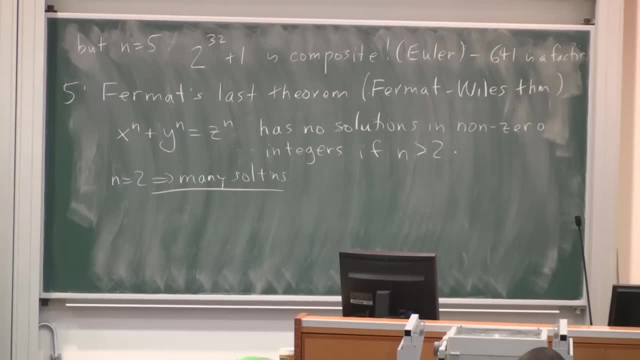 and it was only in fact proven in 1994. Andrew Wiles, after a seven-year-long heroic study of this equation, found a proof using very advanced techniques and many ideas that Fermat would have had no idea about. so the jury claims that Fermat was probably wrong. 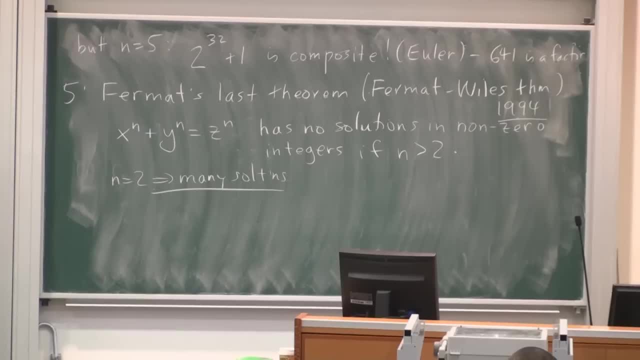 that he didn't have a proof, and most mathematicians believe that, but we're not 100 percent sure. there's always some slight chance that maybe there's some miraculous, simple proof that none of us have found, although it is very unlikely. but this, this problem, in fact, it's not very. 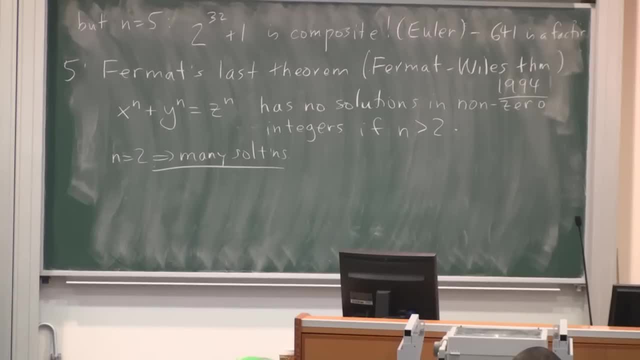 very important problem. really. it doesn't lead to a lot of interesting developments on its own. the mathematics that has come out of this has been very interesting, but the problem itself has a bit of a dead end. but nevertheless it's generated a lot of interesting mathematics and 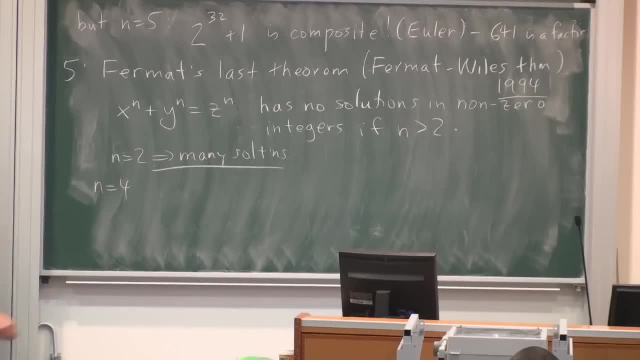 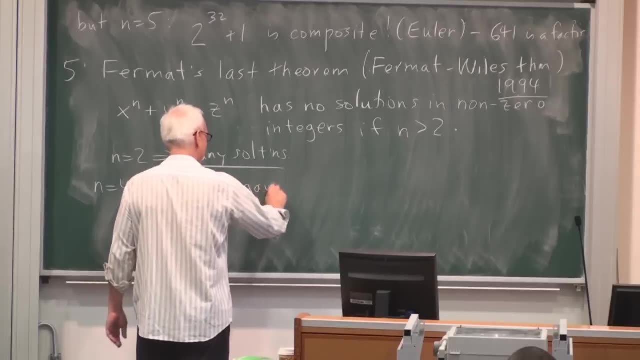 special cases were proven by individuals. so in Euler's four- actually, Fermat actually did write down a proof of this and it's in the Very important- or I can use it based on the bread outer shape- is that humans are always afraid of a building too northeast of home roads, all night long along the road. andボдаppt sich ihrem nicht in den Eunphalischen Lücken, but nevertheless It's generated a lot of interesting mathematics and special cases were proven by individuals. so in n equals four. actually, Fermat actually did write down a proof of this and in the In Order of the Word lt quest Hard to check. 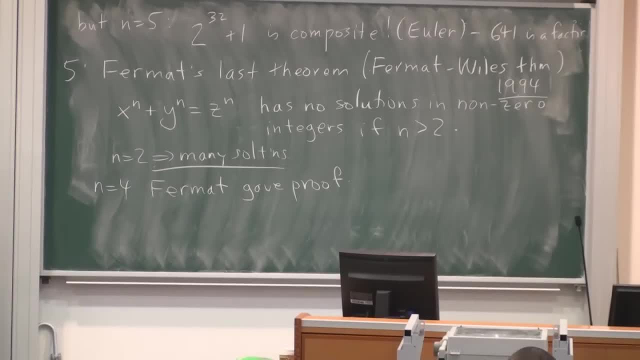 involves an important idea that he called infinite descent, And the idea is a little bit too complicated perhaps to describe at length in a history of mathematics course, But roughly the idea is that Fermat said: all right, let's suppose that we have integers x, y and n, that 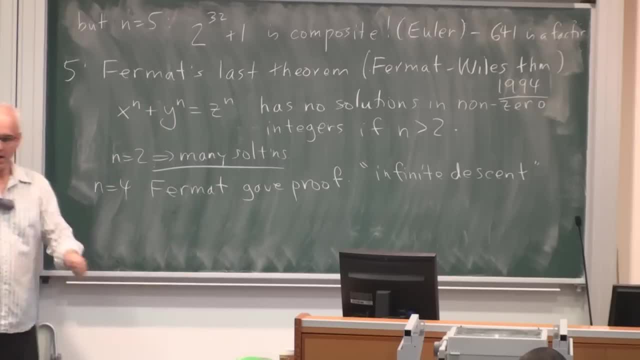 satisfy x to the fourth plus y to the fourth equals z to the fourth. And then he made various deductions and calculations and reductions and so on, And eventually he ended up with a new set of numbers that also satisfied the equation, which were smaller than the ones he'd started with. 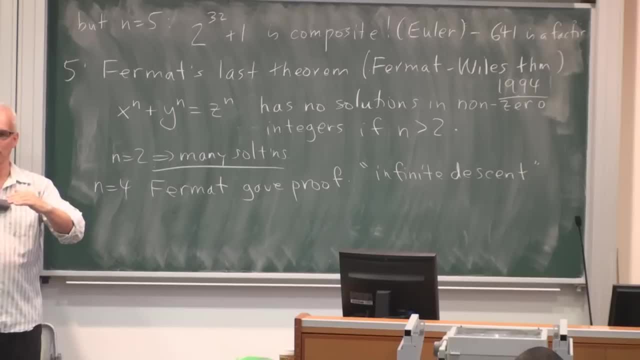 He could prove that if you have one solution, then you can get a smaller solution, And then that was enough for him to say: well then it must be impossible, because we can't keep getting smaller and smaller solutions, because the natural numbers have a bottom. 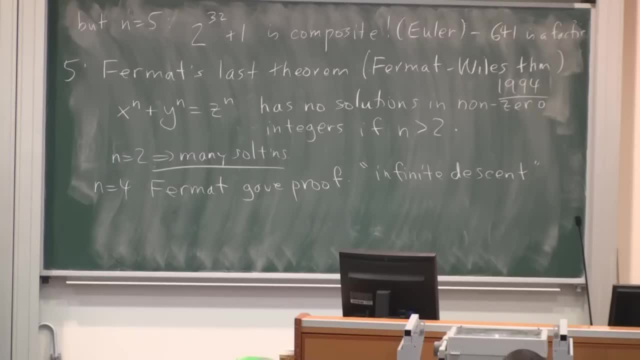 Once you get to zero you can't keep going further. So that was kind of a general technique of proof that he recognized that it was a very important idea of his proof, this infinite descent, And he used it very successfully in other situations. 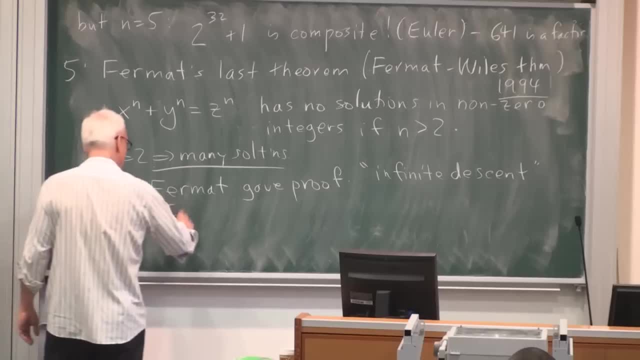 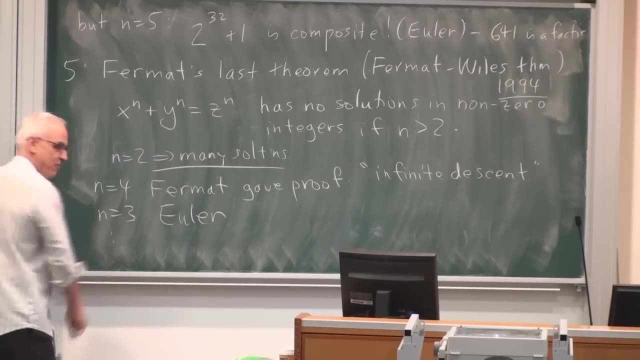 n equals 3 is harder And that had to wait Euler. Euler gave a proof for n equals 3. And many other mathematicians then gave proofs n equals 5,, n equals 6. And typically the proofs are the same. 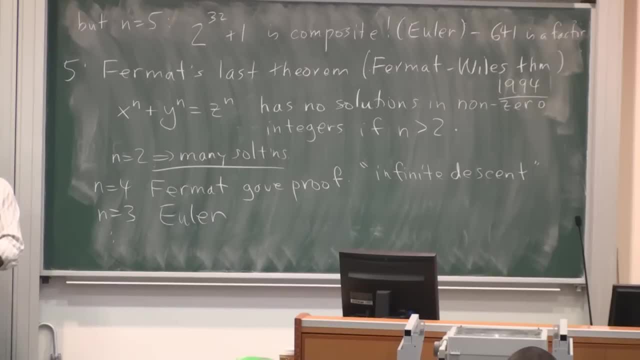 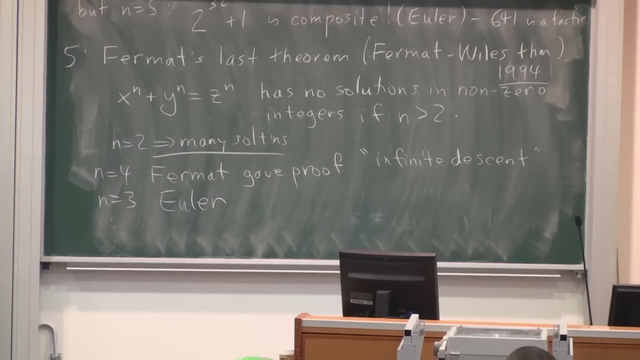 The proof for n equals 5 is quite different for the proof n equals 7 and so on. So a lot of work went into this problem And the problem became famous just because no one could solve it, because it seemed so hard. Thank you. 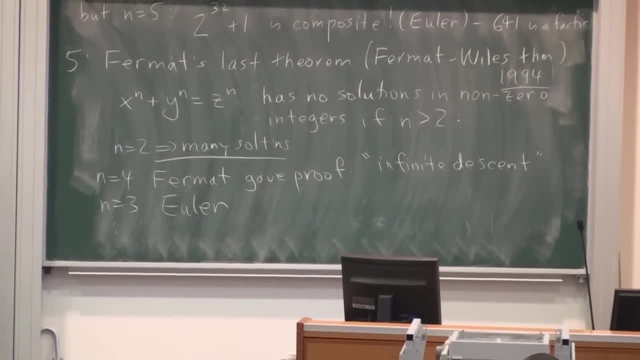 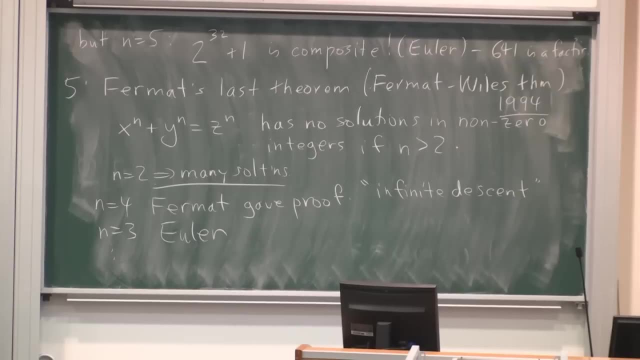 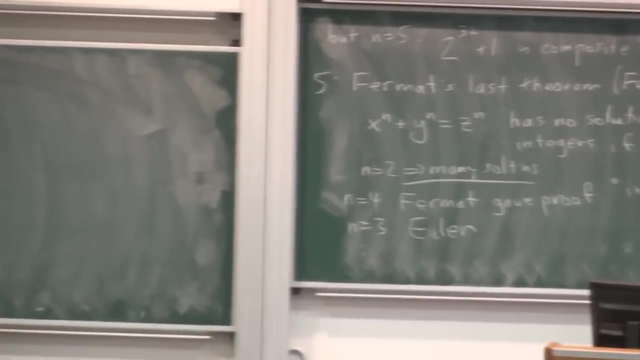 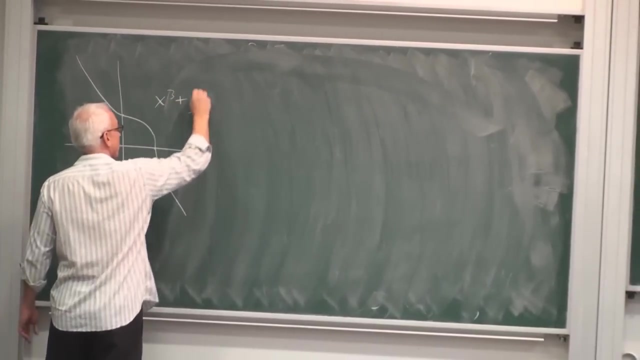 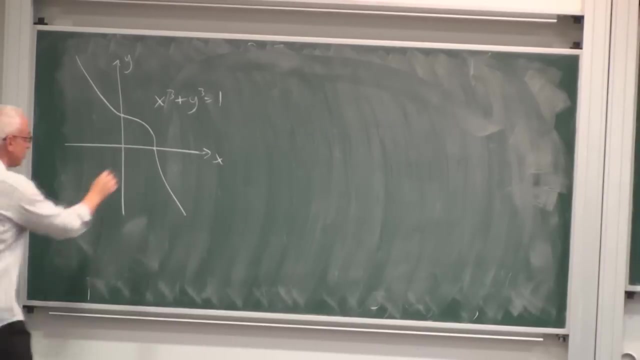 The n equals 3 case has an interesting application to cubic equations. So The cubic equation x cubed plus y cubed equals 1,, just in the ordinary xy plane. It does have two obvious solutions, because it goes through the point 1, 0, and it goes through the point 0, 1.. 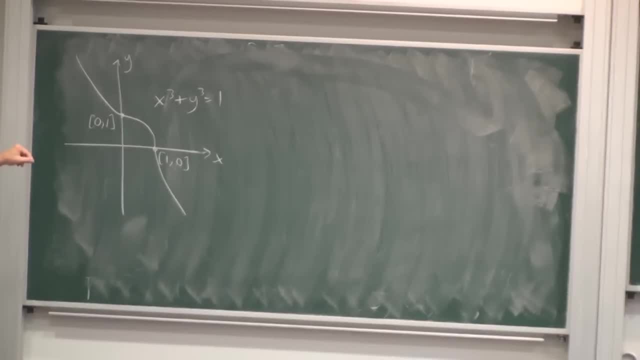 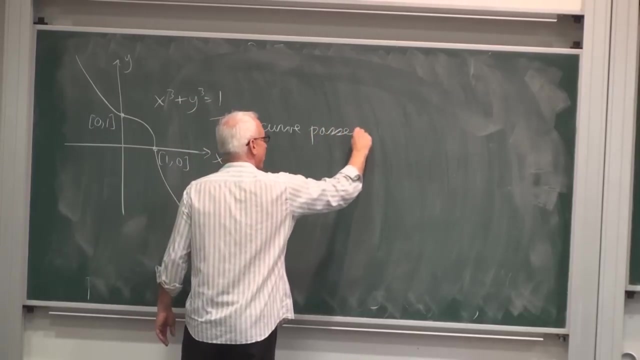 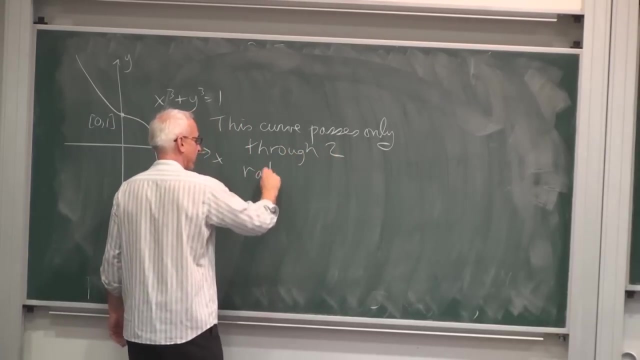 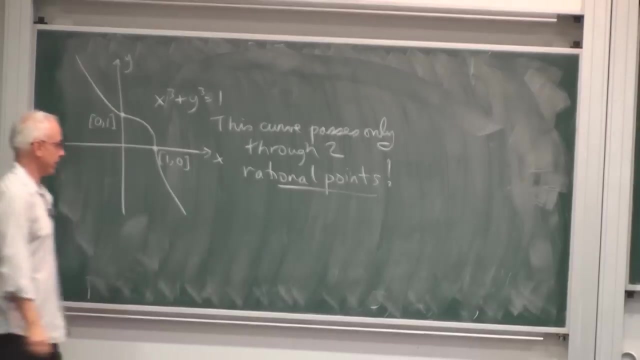 But aside from that there are no other rational solutions. So it's pretty closely connected with the n equals 3 case for the Die-Fonten equation. is the result that this curve passes only through two rational points, Which of course is very difficult to do. 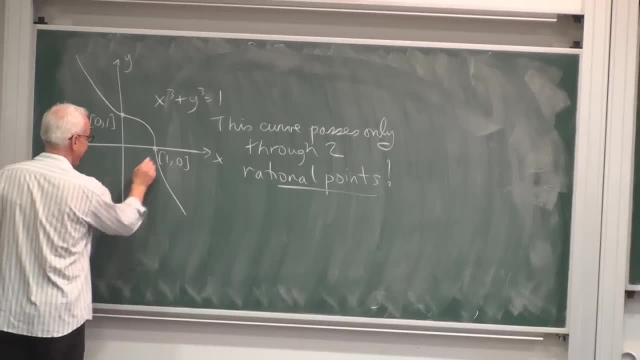 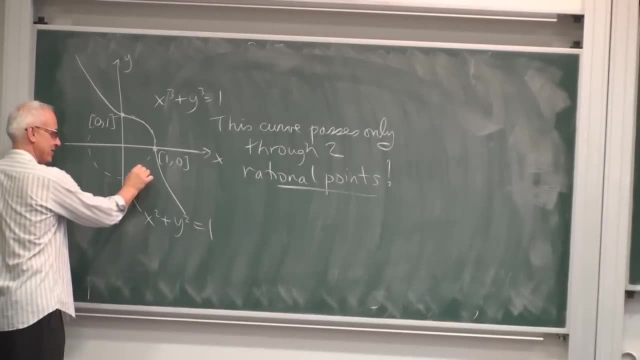 It's very different from the case of the circle- x squared plus y squared equals 1, which passes through an infinite number of rational points. So you might say: well, what am I graphing here? Well, there are lots of points, rational points, which are pretty close to satisfying this equation. 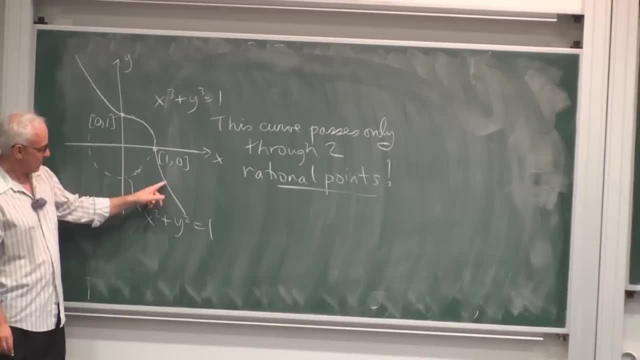 And you can think that that's what we're graphing here. This is a plot of a point for which x cubed plus y cubed is pretty close to 1, but not exactly equal to 1.. So Fermat realized also that this whole problem of asking the question 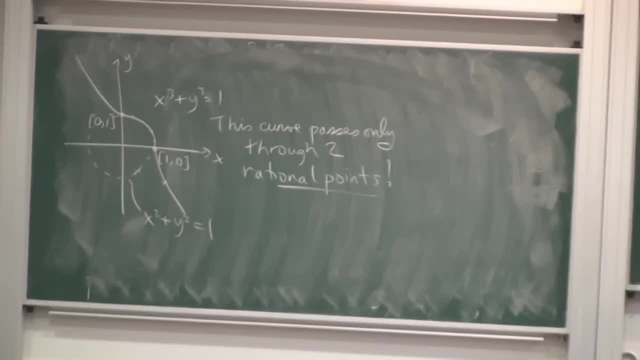 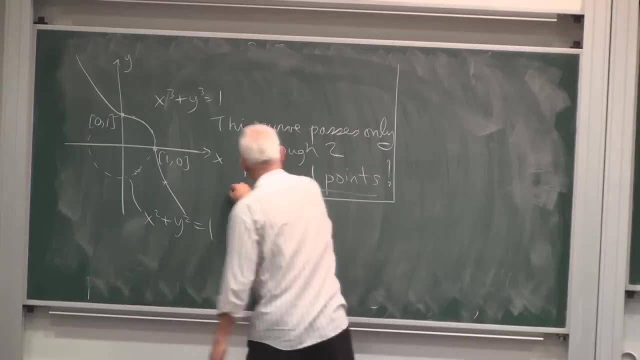 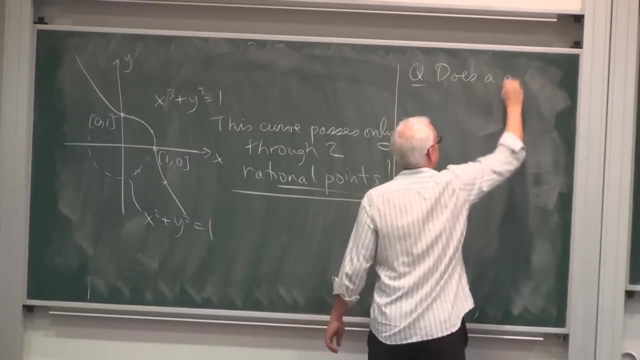 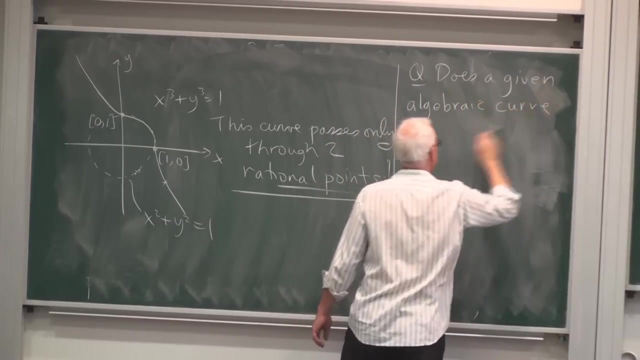 given a curve in the plane, does it have rational points was a pretty interesting and important question And that turned out to be a very, very important line of thought. So the question is: does a given algebraic curve, say given by an equation of the form p, x, y, equals 0, where p is a polynomial? 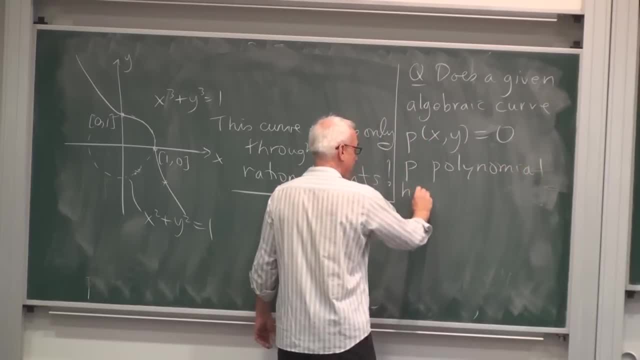 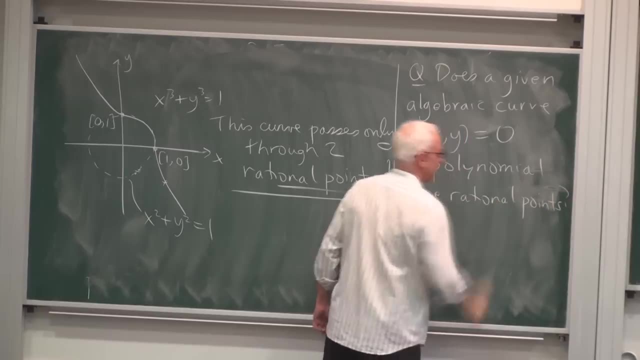 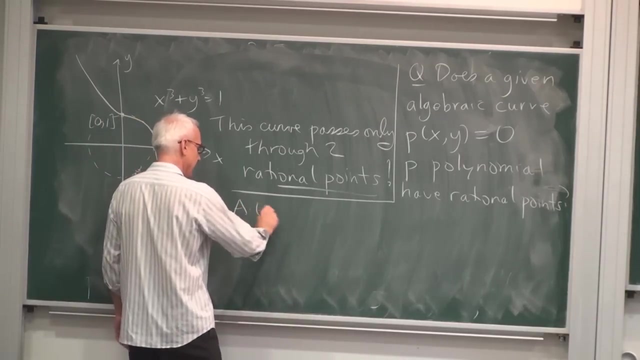 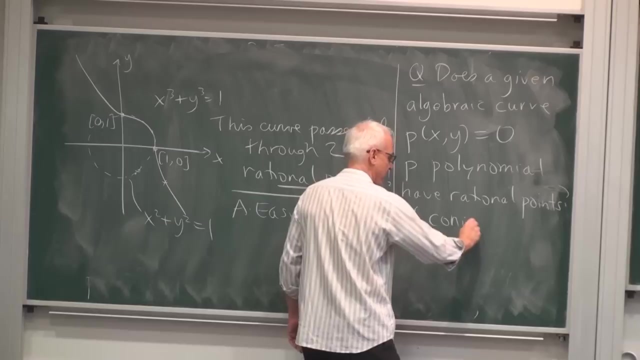 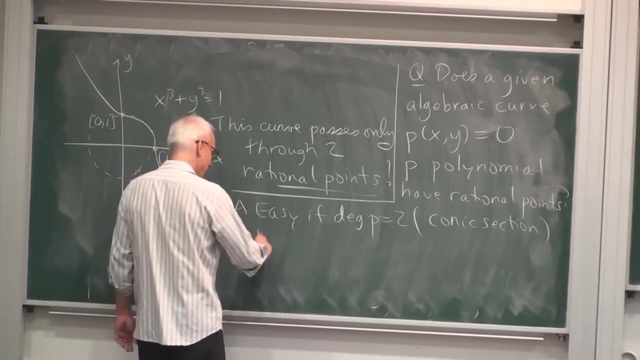 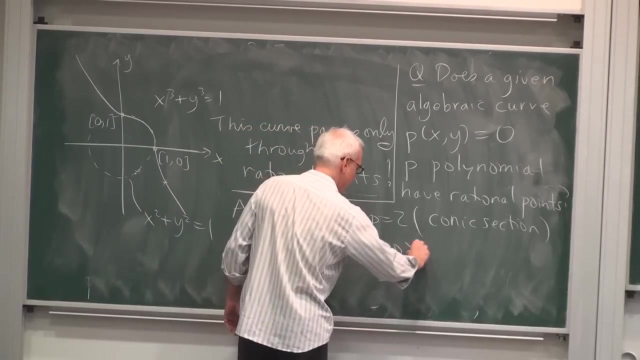 have rational points on it, And it turns out that question is pretty simple. The answer is easy if the degree of p equals 2. In other words, when we're talking about a conic or a conic section. But not so easy if the degree of p is bigger than 2.. 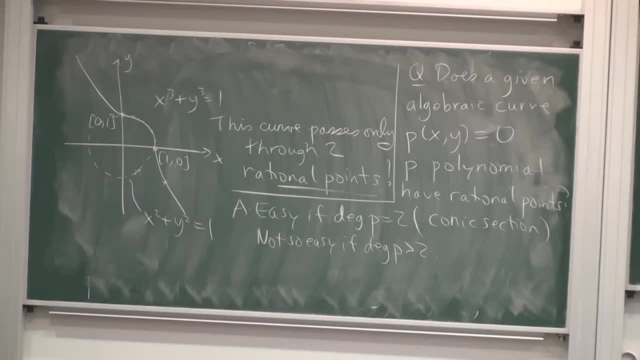 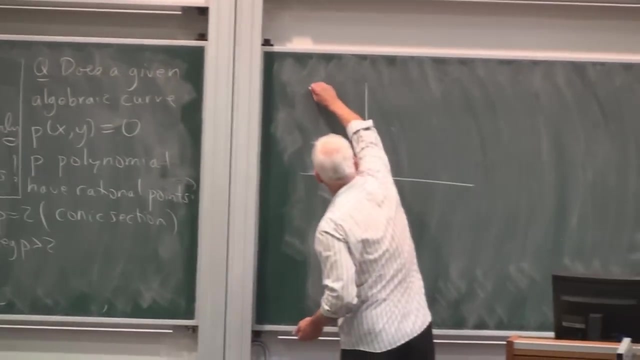 In particular for cubics. it's already rather a subtle issue, And Fermat introduced an important technique for well investigating some of these things, which again in some sense goes back to Diophantus, but he extended this idea. 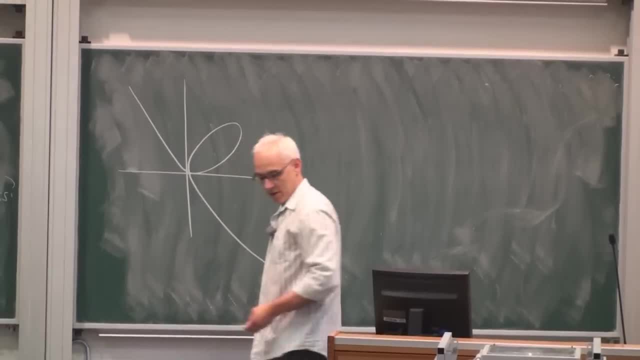 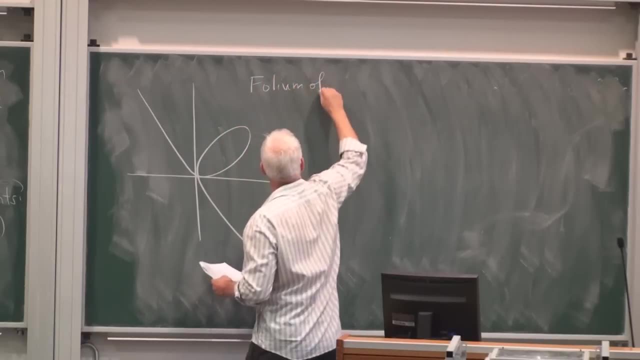 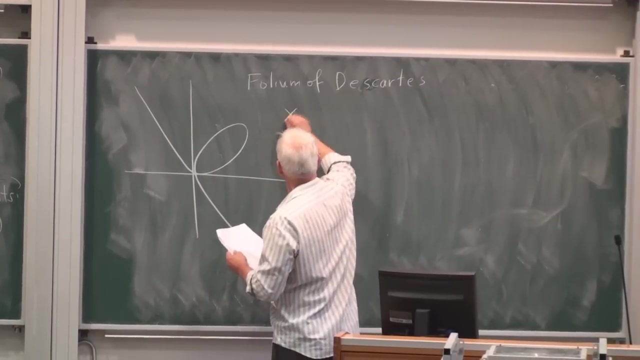 So let's look at a curve. Let's look at this curve here, which is well a folium of Descartes. It's a cubic and it has the equation x cubed plus y cubed equals 3xy. 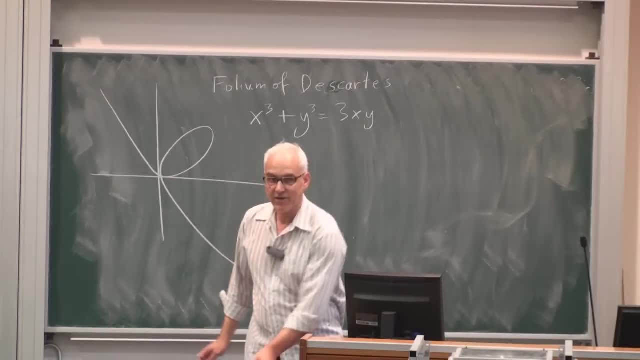 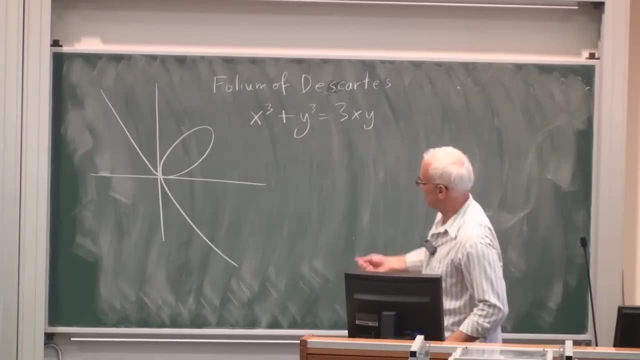 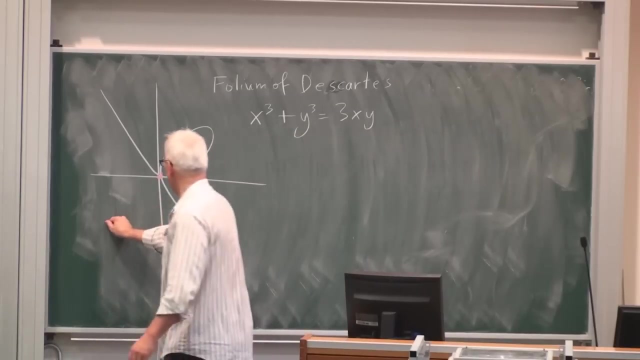 So Fermat realized that Diophantus' idea of thinking about tangents could be extended to thinking about secants. So he said: all right, there's something special happening about the point 0, 0 here. Let's look at a line through that point. 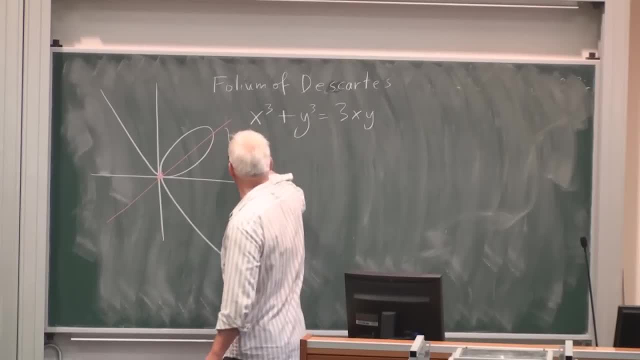 Such a line has equation y equals tx, where t is just the slope of that line. So let's see if we can find this point. We know two of the places where this line meets the cube, Namely this point right here. 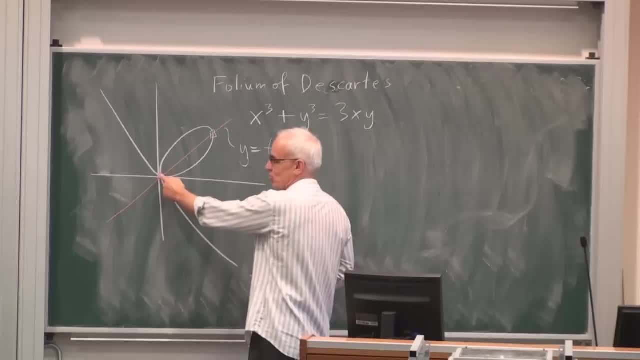 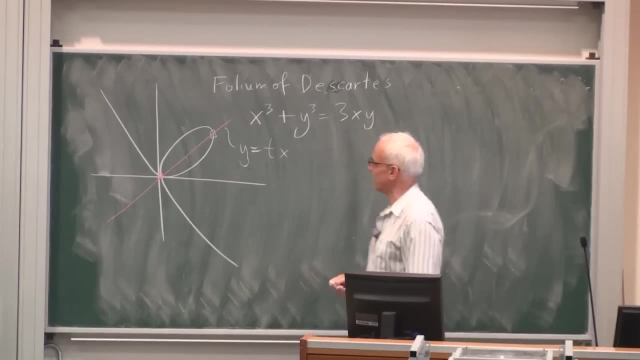 This is really a double meet. The line meets the cubic twice at that point. So there's one more place where the line meets the cubic and we should be able to find that out. So if you substitute y equals tx into here. sub in. 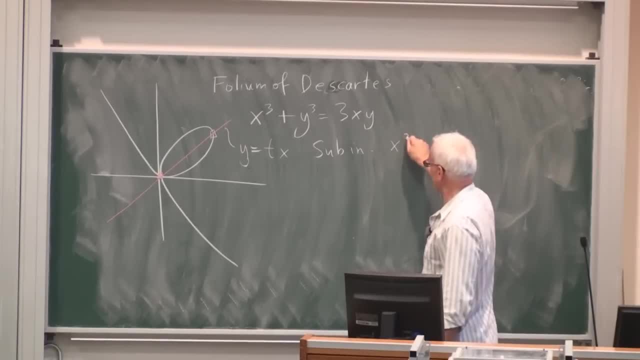 then what do we get? We get x cubed plus. then we put this in here: so t cubed, x cubed equals and here 3x times tx, so tx squared, And then conveniently the solution x equals 0,. 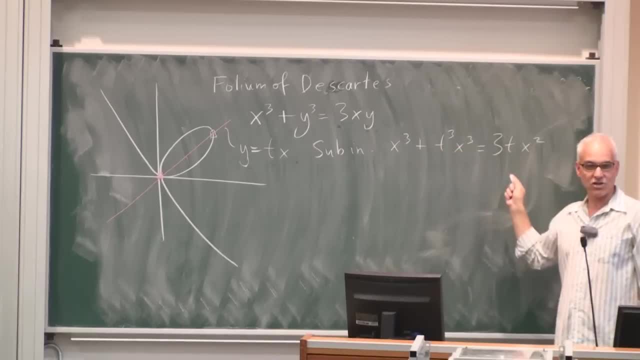 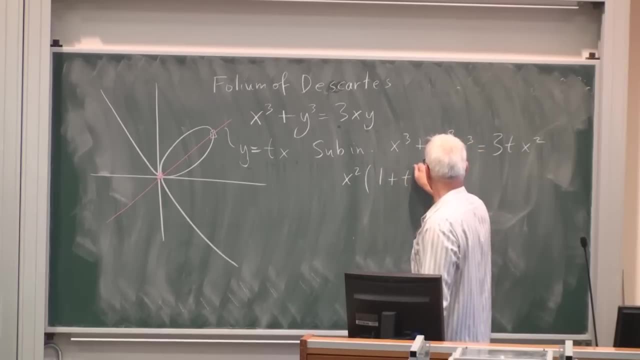 which we already know about, is appearing as a common factor of x squared here. So in other words, if I factor the things out, I get x squared times 1 plus t, cubed minus 3, I guess there's an x. 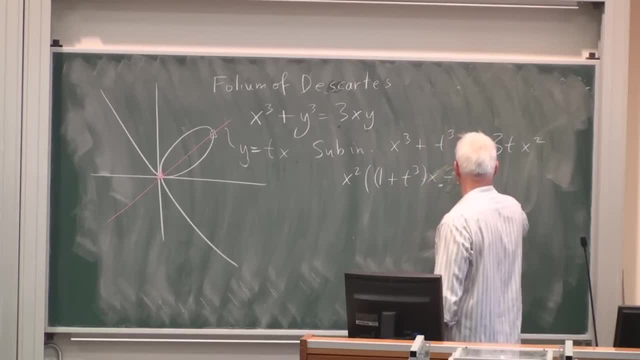 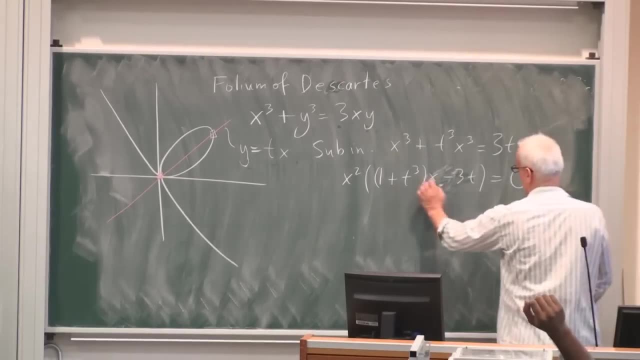 All right, like this, x minus 3t equals 0.. So I brought everything to one side and factored out an x squared and I have 1 plus t cubed times, x still remaining and minus 3t. So we know that x equals 0 is a solution. 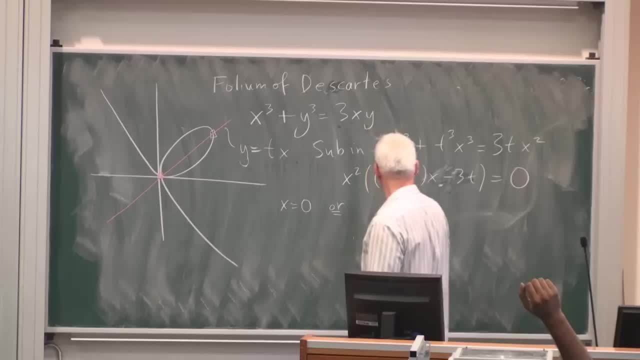 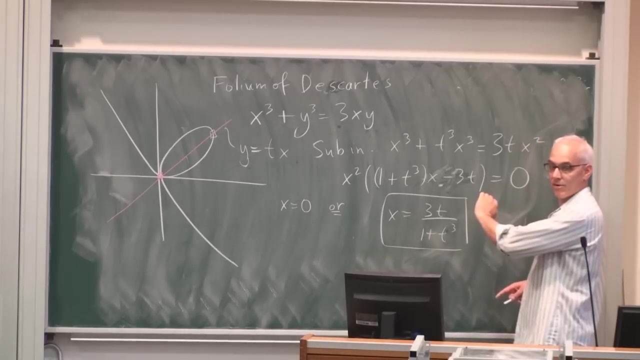 Fine, that corresponds to here. The other solution is: x equals 3t over 1 plus t cubed. All right, this one here. well, I've got in the bracket here, so this bracket is multiplying that times X, and so if we found X, then if we go back to the line, 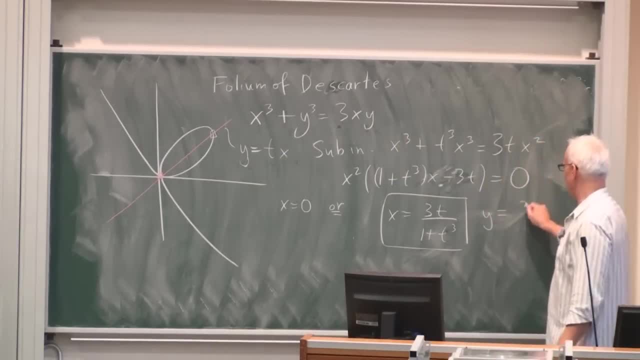 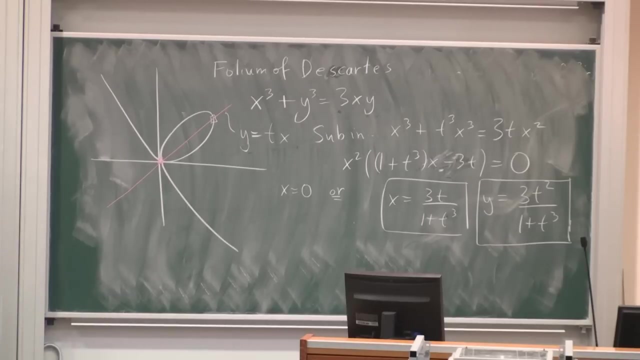 then Y is just T times that. so Y will be 3 times T squared over 1 plus T cubed. so that's actually a, now a parameterization of the cubic. that means for every value of T, if you replace T with a particular value, you get an X. 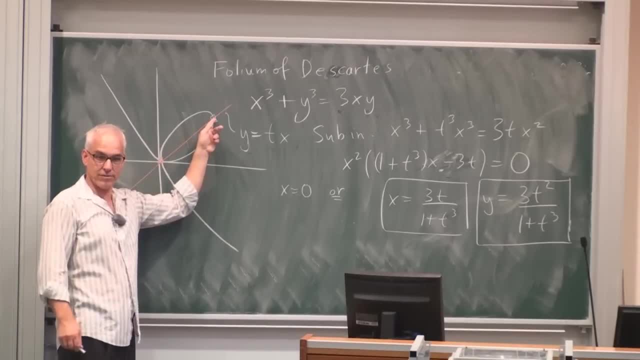 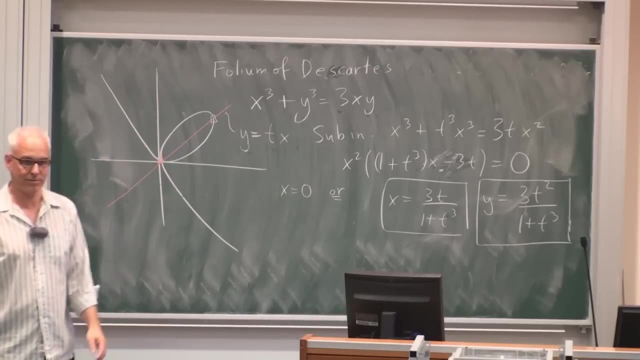 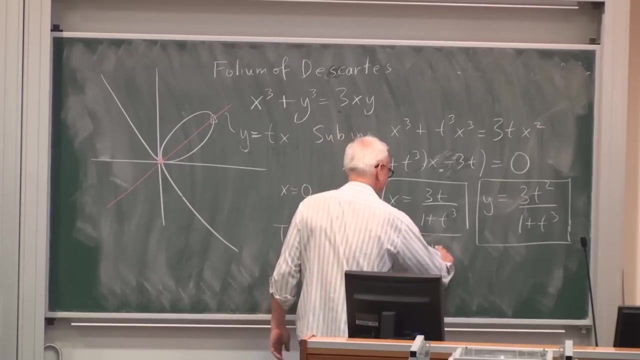 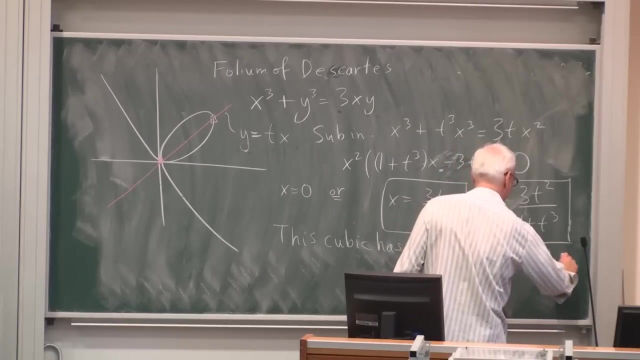 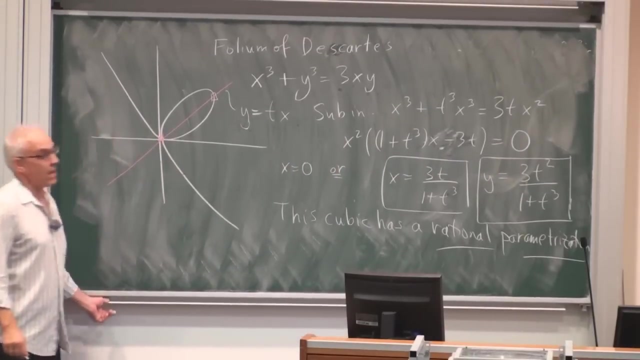 value and a Y value that give you a point on the curve. so you can generate the points on the curve in this very simple way, with this parameterization. so this cubic has a parameterization fact has a rational parameterization, which is even better. there's a rational parametrization now in the modern theory of curves. 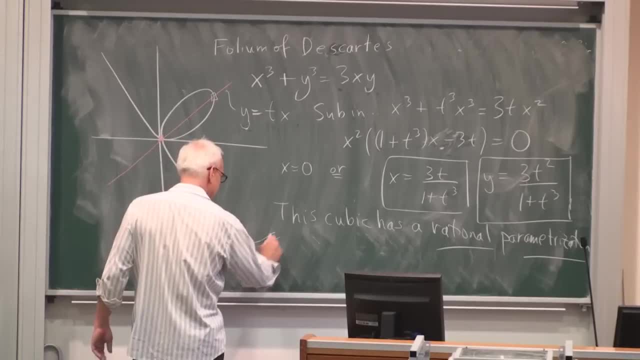 hey, that means that sort of saying that this is a genus 0. that was a genius, a we need a jury to eliminate as soon as you're out and you work really well together. you got to do it, you got to do. next, your X is: admit, but don't forget to click like I'm not doing it. 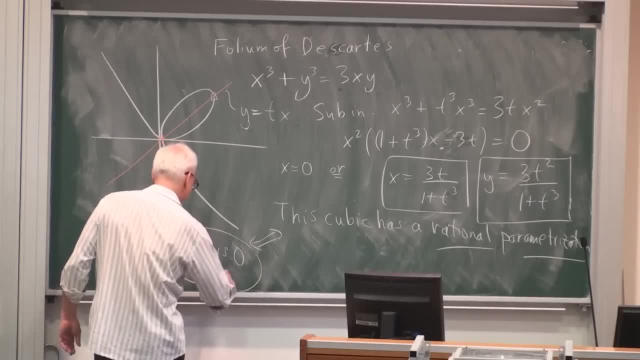 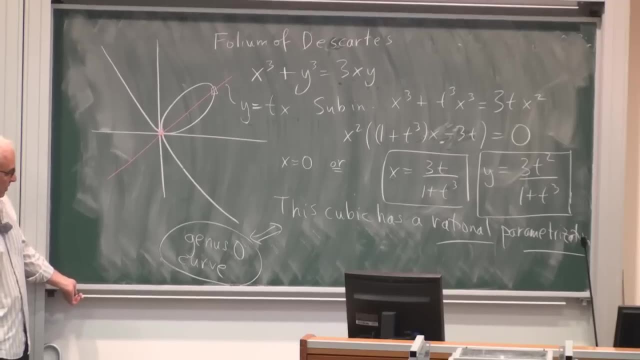 This is a genus zero curve. Let me just put that terminology out there. A little bit later in the course we might have a better understanding of what that might mean once we learn a little bit more about complex numbers and a bit of topology. 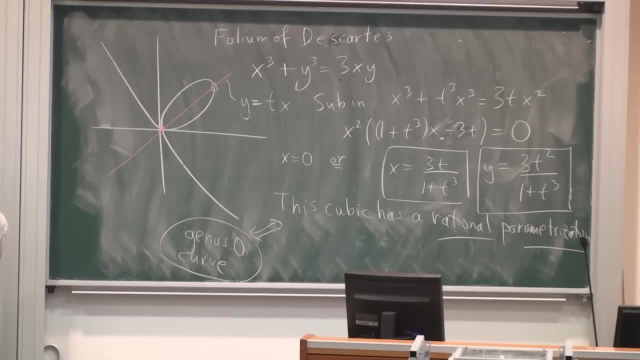 That's a genus zero curve. but not all cubics are genus zero curves. because, for example, this cubic is not a genus zero curve because it does not have a rational parameterization. If it had a rational parameterization then there would be lots of rational points on it. 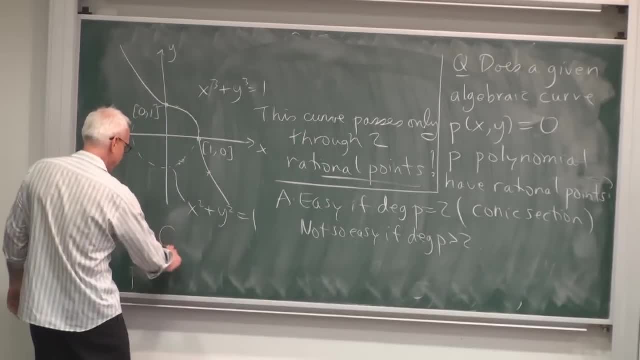 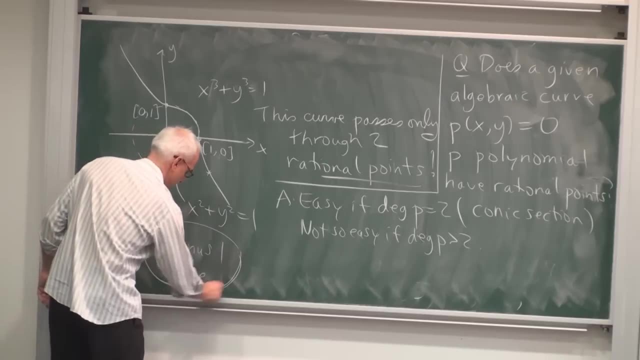 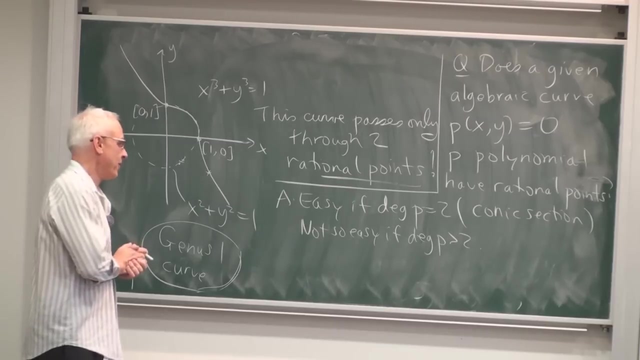 but we've said that there are no rational points on it. So this thing here is of- well, it's not of- genus zero, It turns out to be genus one. So we're getting close to this idea that in the world of cubic curves, 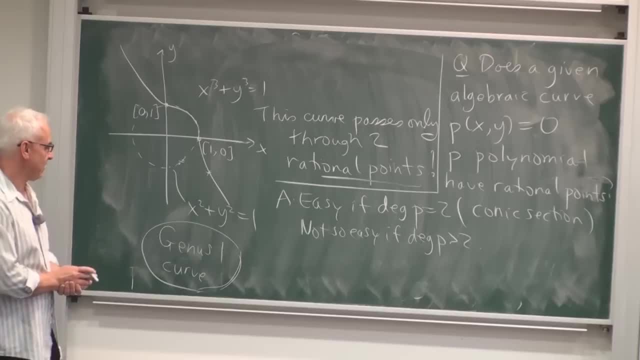 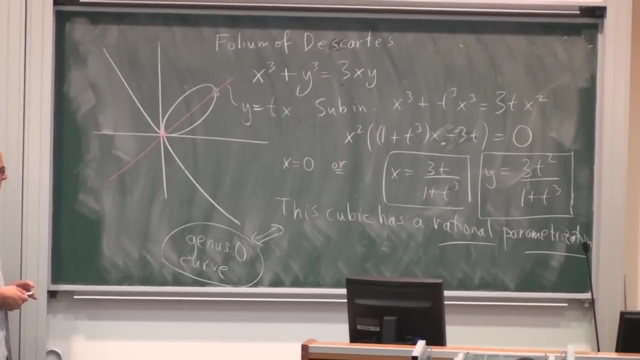 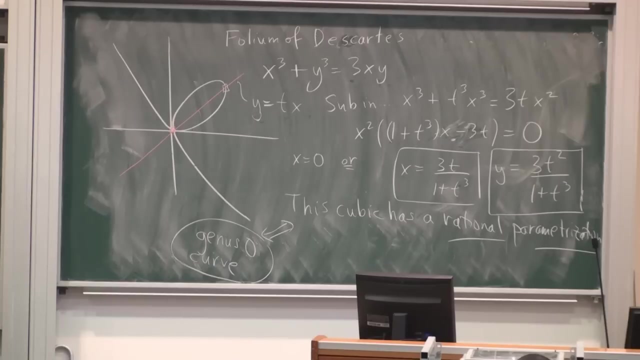 there is a big division between certain kinds of cubics and other kinds of cubics, And relating to this question of whether a curve has a rational parameterization or not, And perhaps, while I'm talking about this, I'll also draw another picture of kind of an interesting and important phenomena- 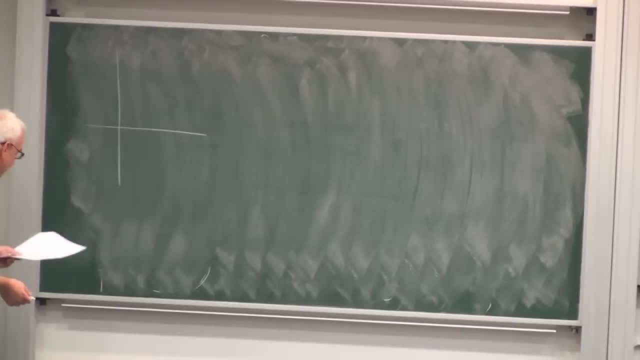 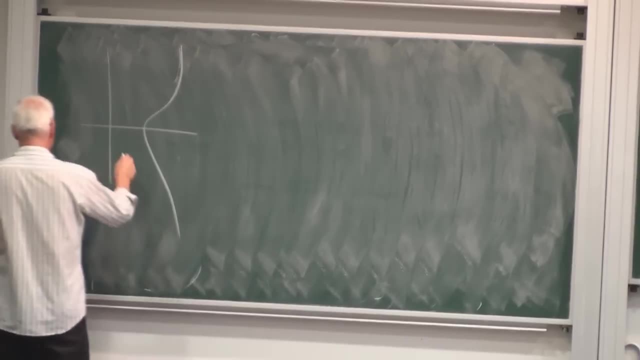 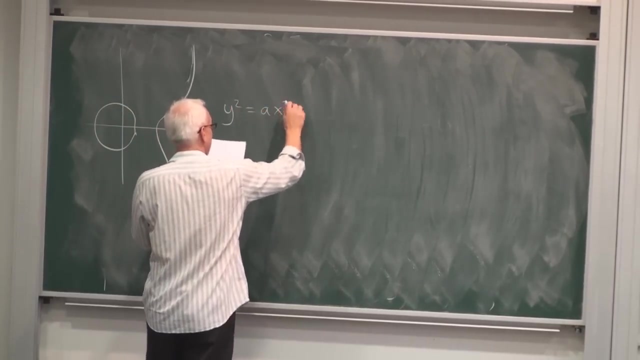 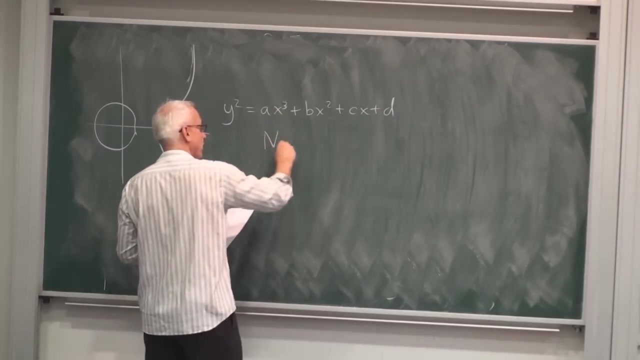 that happens with cubic curves that you will not have seen in high school. So if you have a cubic in that has the form y squared equals a, x cubed plus b, x squared plus c, x plus d, this is one of the Newton forms for a cubic. 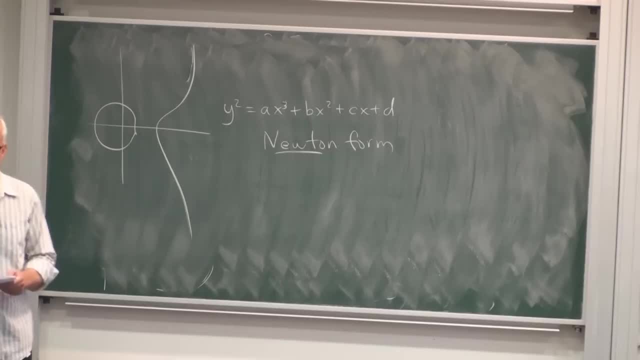 I remind you that Newton classified cubics and tried to put them in families like ellipse, hyperbola, parabola, something like that, And he had quite a long list, 70 or 80 different types of forms, And one of the things he did was find 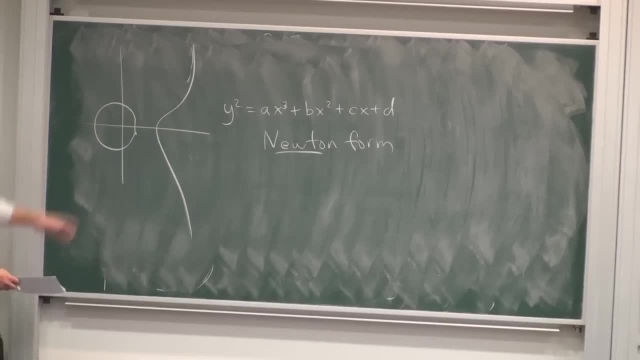 sort of standard forms for cubics. This is one kind of form, And if you choose the numbers a, b and c and d in the right way, then you can get a graph that looks like this: It's another kind of shape that a cubic curve can have. 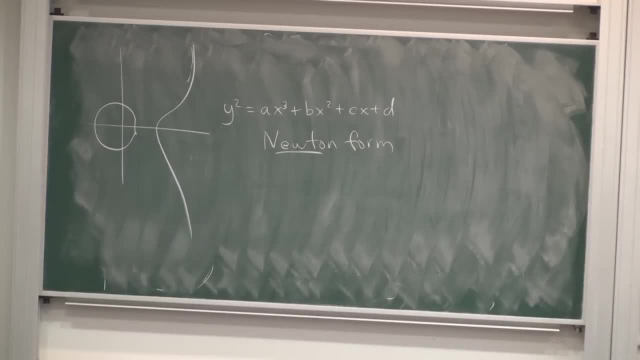 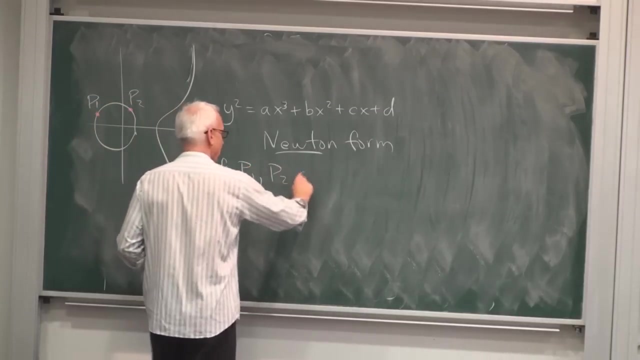 And sort of along those lines, sort of along the lines of what Fermat's thinking was going. here you can make the following observation That if you have two rational points, so let's say you have p1 and p2.. If p1 and p2 are rational points, 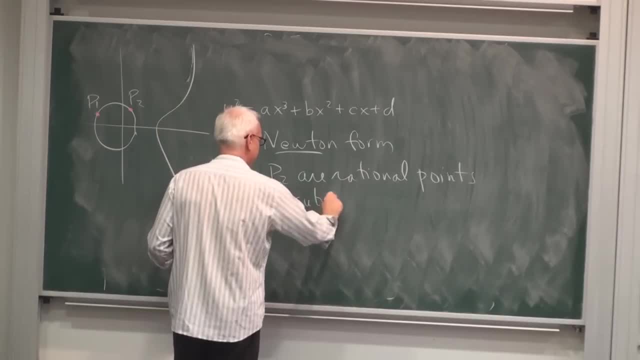 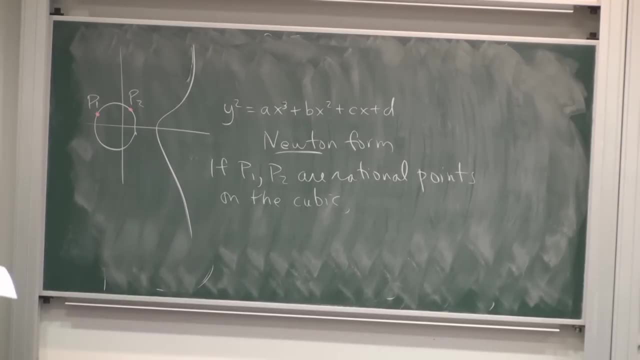 on the cubic, then we can obtain another rational point By essentially the same way, by essentially the same kind of thinking as Fermat was doing in that previous example. what we do is we just join those two points to form a line And that line typically meets a cubic in three points. 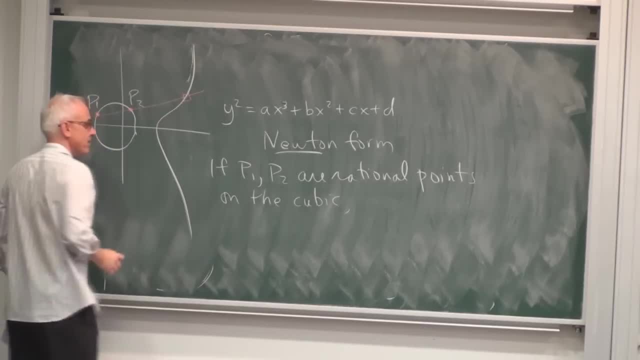 Because it's an equation of degree three. So there will be a new point And you can get that point without having to solve a cubic equation, because you already have two solutions. It's the same idea that we had over here, The fact that we already had two solutions. 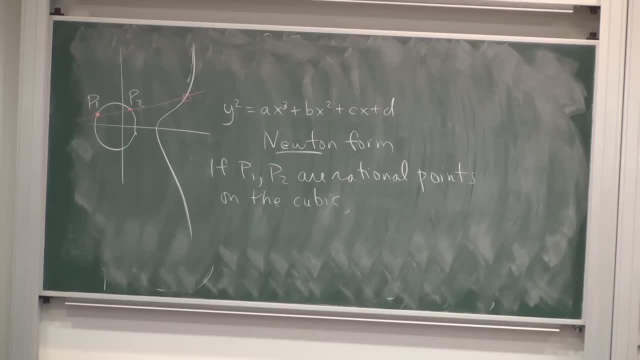 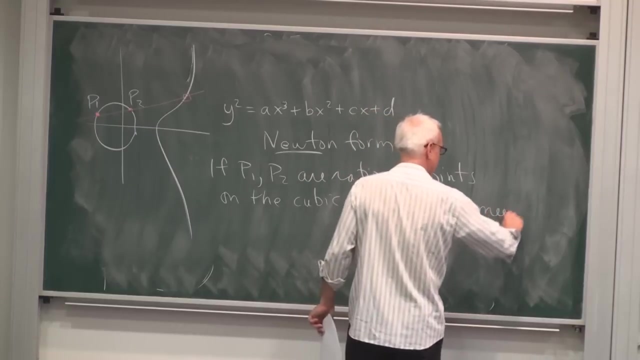 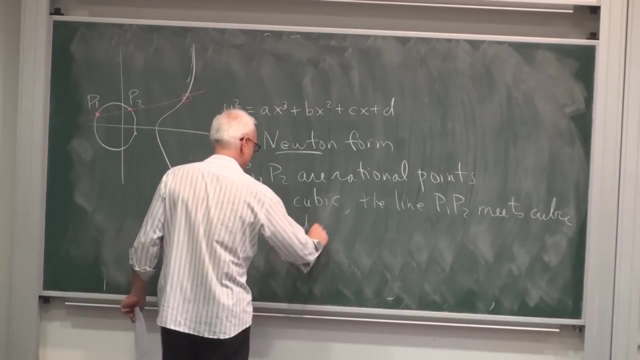 allowed us to find this third point. We didn't have to really solve a cubic. The cubic came down to a linear equation. The same way, if you investigate this, you find that the line p1, p2 meets the cubic in a third point, a third rational point. 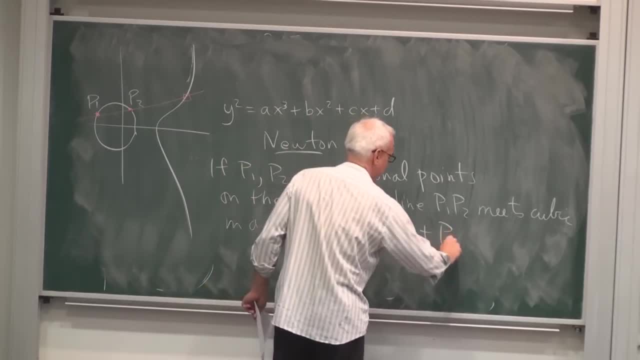 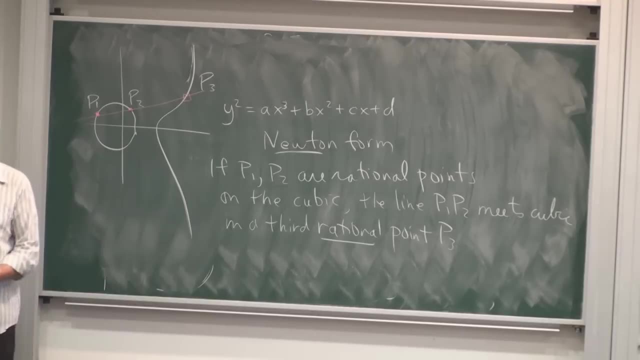 Let's say p3.. So this is now a fun game that you can do. if you have a cubic, If you know a few rational points, you can generate other ones by joining the dots, making lines and seeing where they meet, For example, in this case, here. 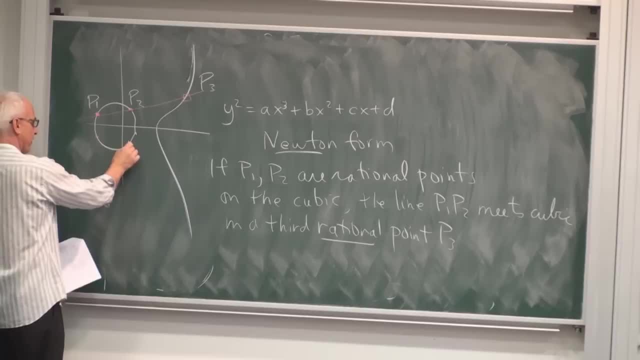 if this is a rational point, then its reflection will also be a rational point. This reflection will also be a rational point. That means we could say: join this one with this one, get another line which would meet again in some other place. 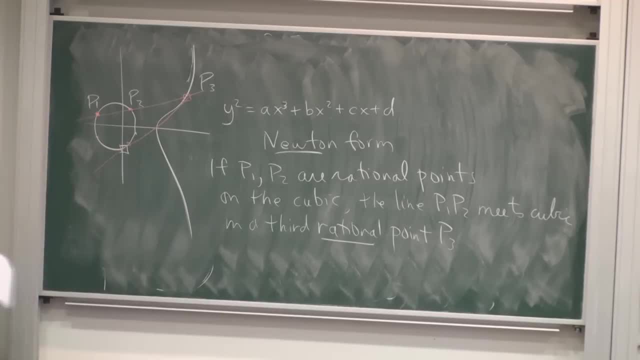 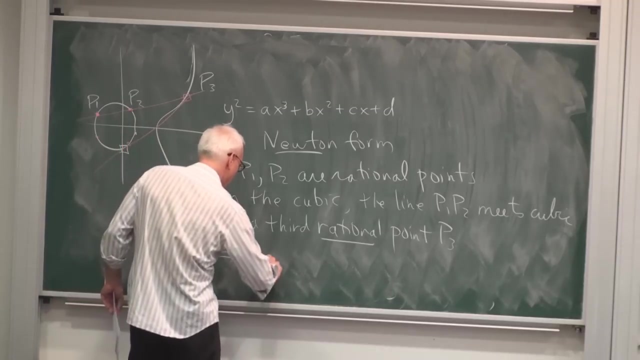 maybe here or here, I don't know where- It should only meet at once. That would give us another point. We can continue generating more and more rational points, And that turned out to be an important development that led to, ultimately, the group law on a cubic. 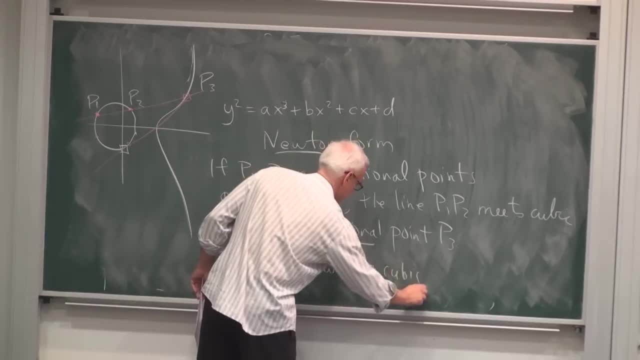 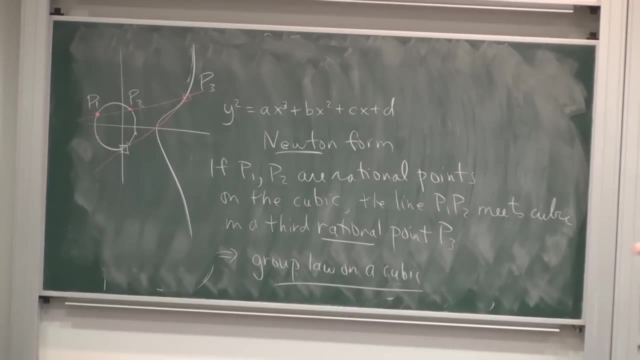 All right, that's a little bit advanced. It's sort of touching with modern algebraic geometry, And that area of investigation is still, even today, a very hot research topic, In fact related very strongly to the proof of Andrew Wiles. 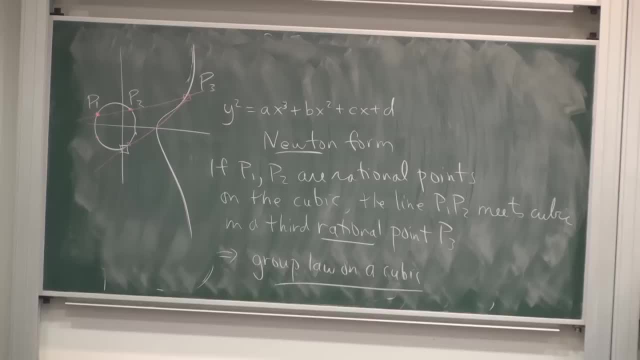 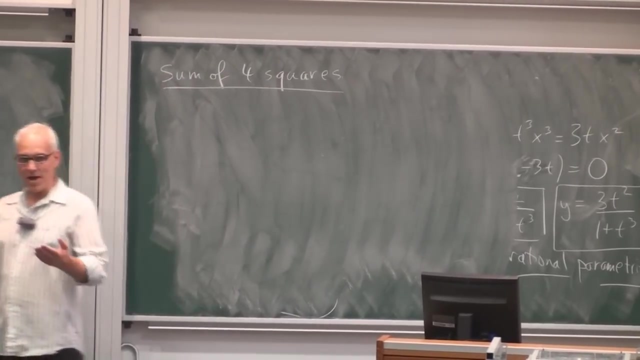 the Fermat theorem, And I'll end today, today's lecture, with just one more interesting kind of thing that Fermat was involved in, And that's a sum of four squares problem. So Fermat observed that not every natural number could be written as a sum of two squares. 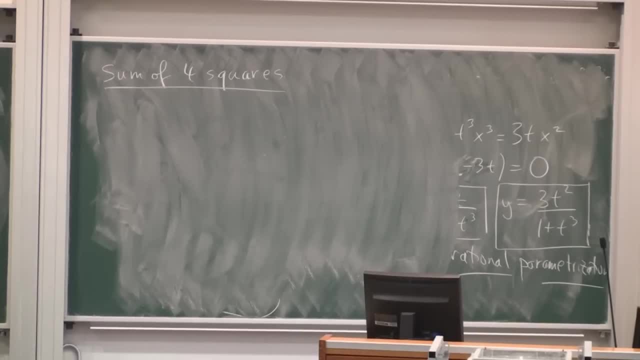 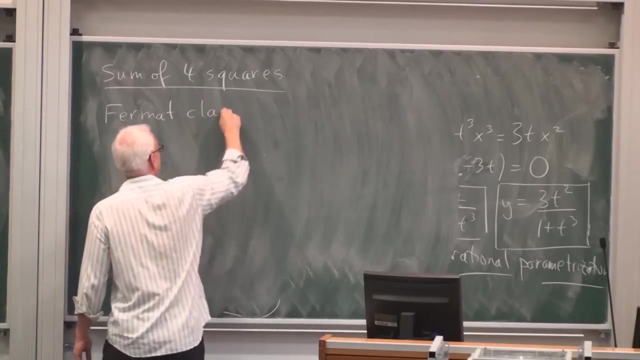 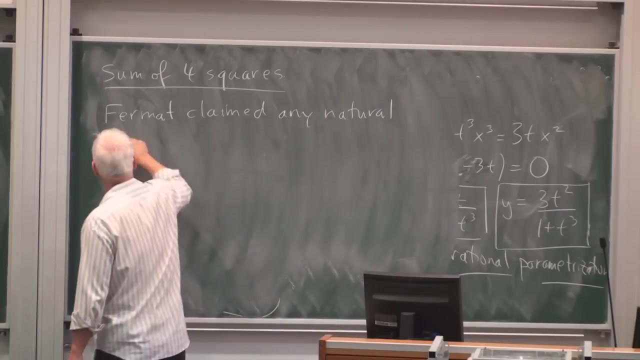 But if you allow yourself three squares, then a lot more numbers can be written as a sum of three squares, But still there are some numbers that cannot be written as a sum of three squares either, And Fermat claimed that that any natural number could be written. 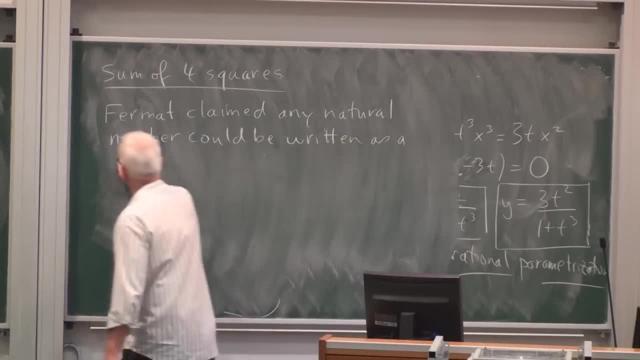 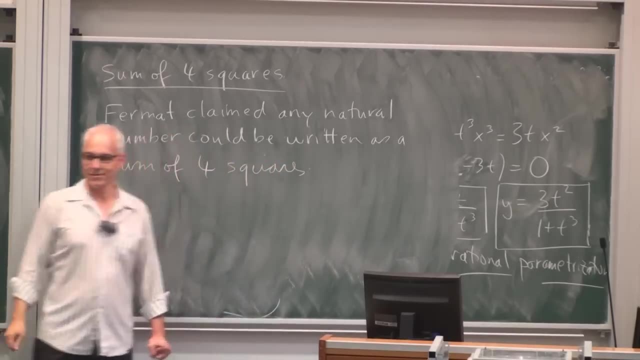 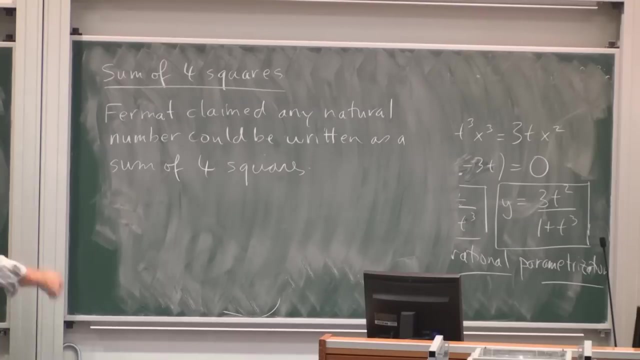 as a sum of four squares. So if you choose any natural number, then you can write that as a sum of four squares. For example, how about 35?? So 25, maybe, And we have to do 10.. 10 is 9 plus 1 plus 0.. 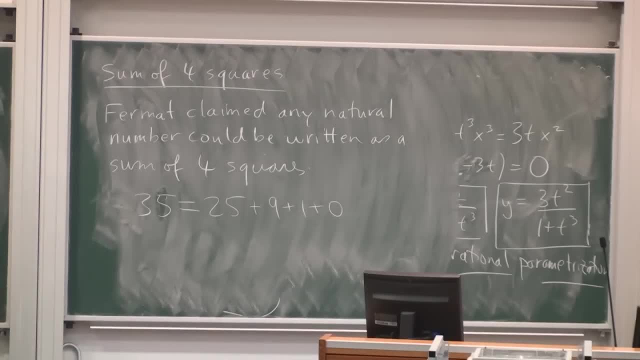 There's a sum of four squares, We're allowed to use 0, too. Maybe not so impressive when the numbers are small, but when the numbers are very big it's somewhat interesting. But again, this is a result that other mathematicians tried to prove. 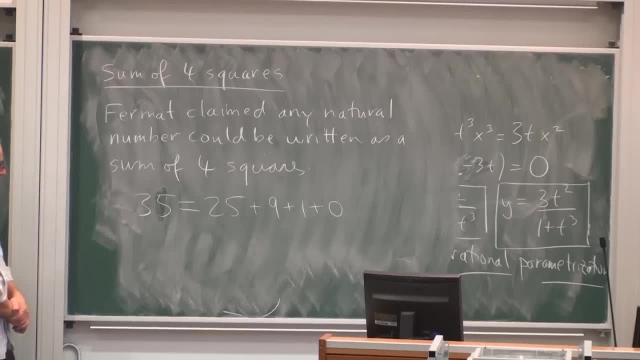 Euler tried to prove it and made some progress, And it was Lagrange who ultimately proved it. Well, I must of course tell you of perhaps Fermat's most important discovery in terms of actual practical applications. No discussion would be complete without that. 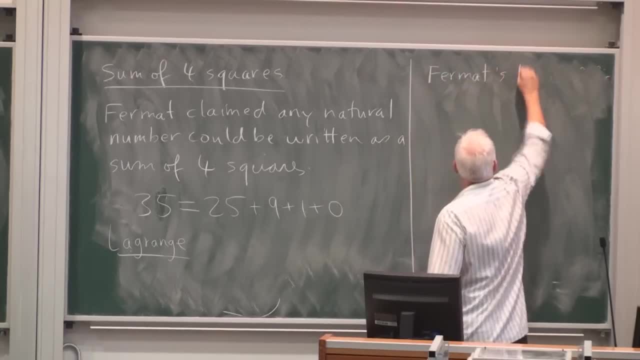 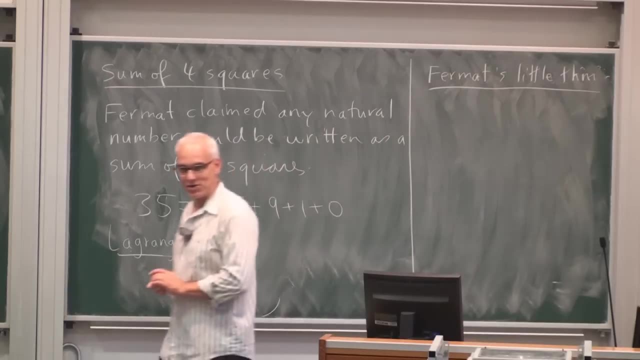 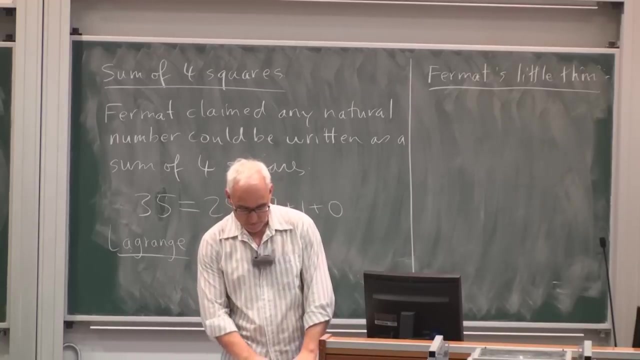 This is sometimes called Fermat's Little Theorem. For many years this was just a novelty in number theory. In the last few decades it's become vitally important for Internet security. So most of the powerful Internet encryption programs that we have. 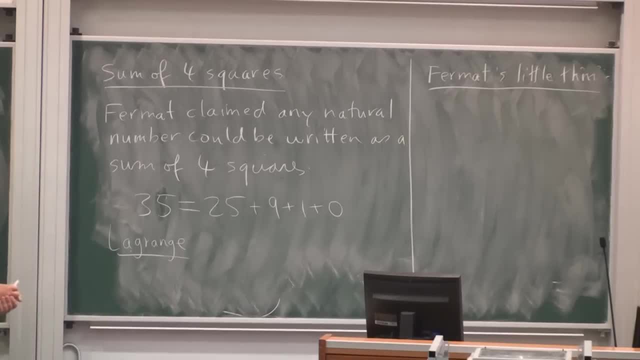 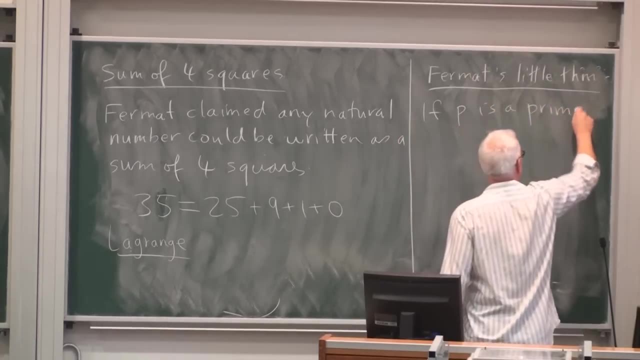 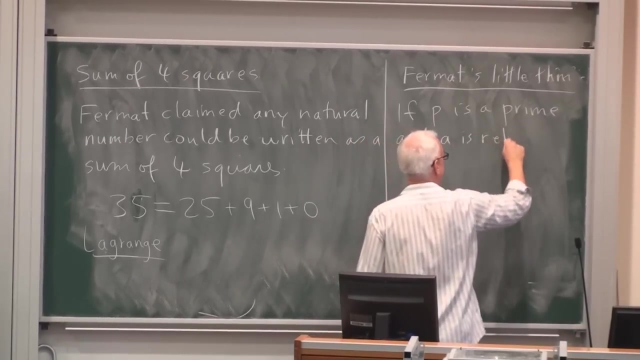 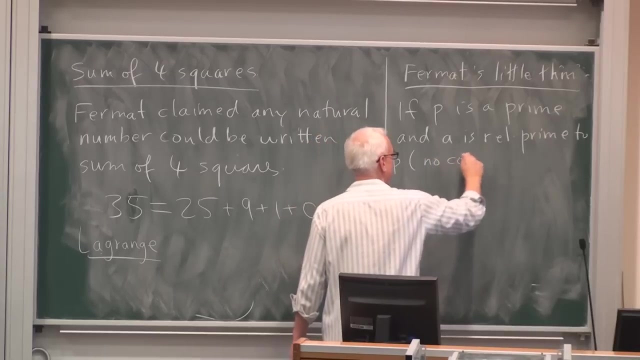 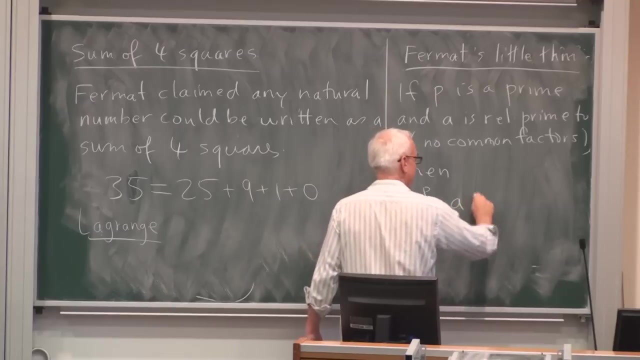 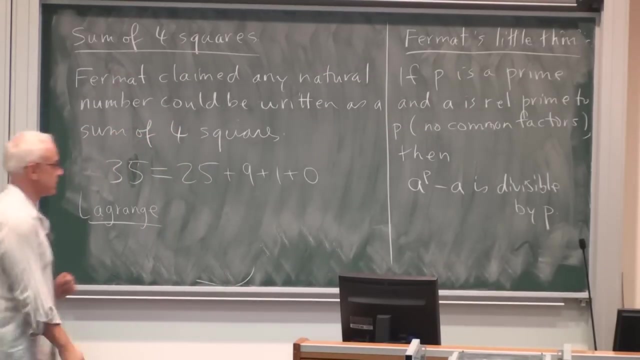 rely on this result and variants of it. So the result is that if P is a prime and A is a number, A is relatively prime to P. that means no common factors. then A to the P minus A is divisible by P. Fermat was very interested in divisibility questions. 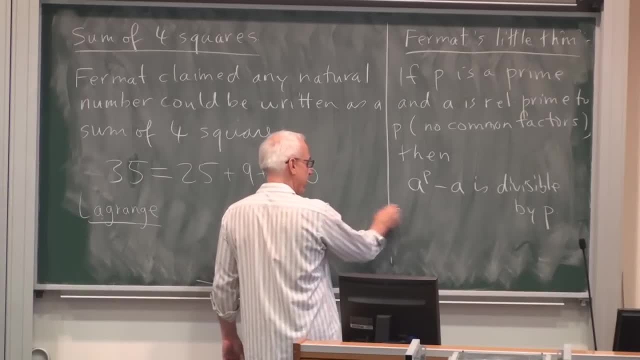 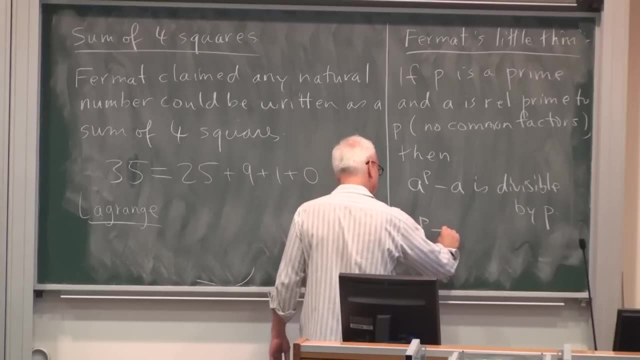 and he would have not written it this way. but later on Gauss introduced what was called congruence arithmetic And Gauss would have rewritten this in the form: A to the P is congruent to A mod P. That's an equivalent statement in using Gauss's congruence language. 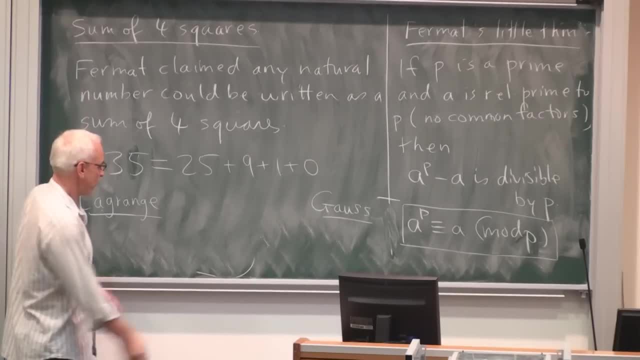 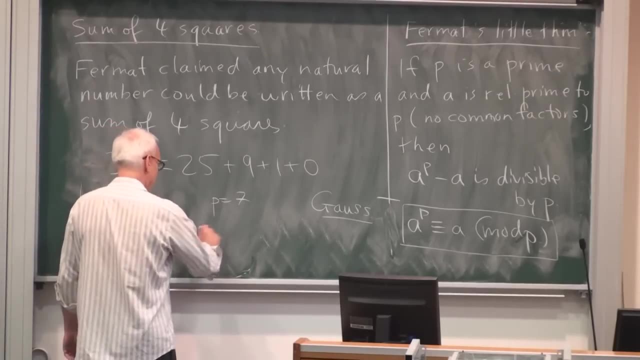 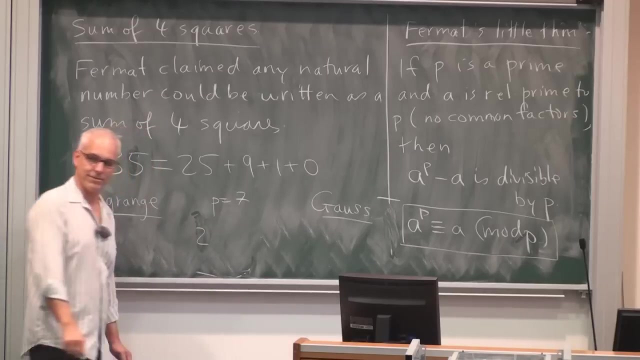 So, for example, if we take P equals 7, let's say, and we take some number, say 5, maybe 5 is a bit too big, Let's take 2.. What is 2 to the 7?? 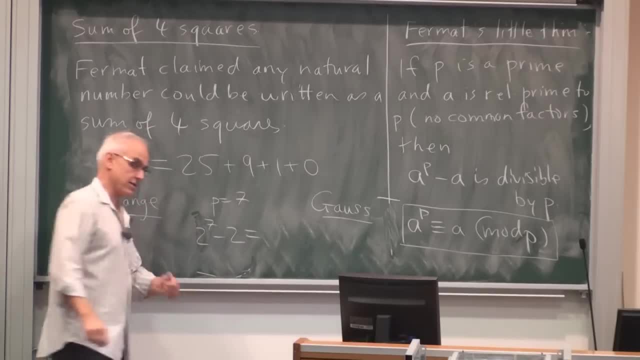 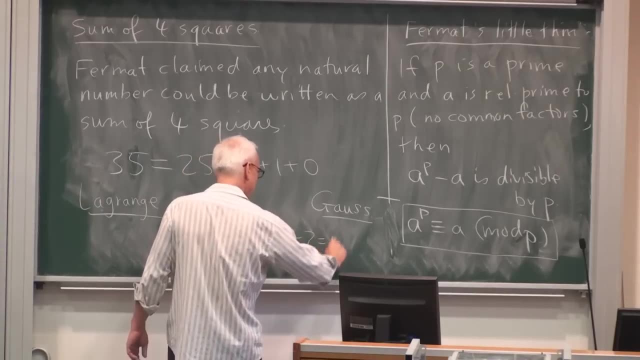 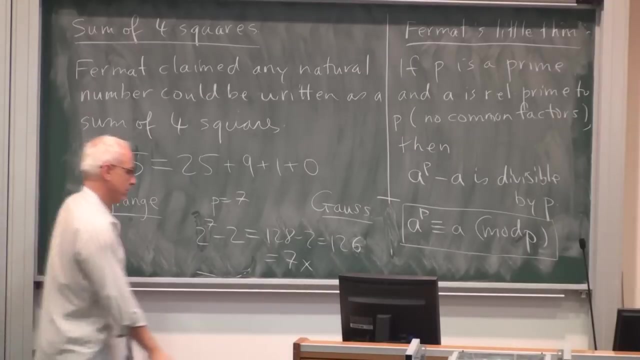 Minus 2.. Okay, so what's 2 to the 7? 128.. So this is 128 minus 2.. Which is 126.. And that is 7 times 18.. It's divisible by 7. And that works not just for 2,. 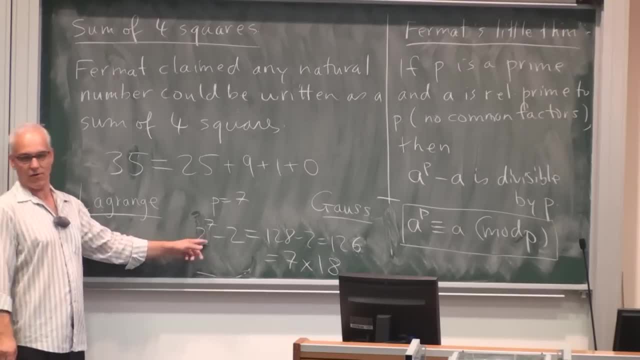 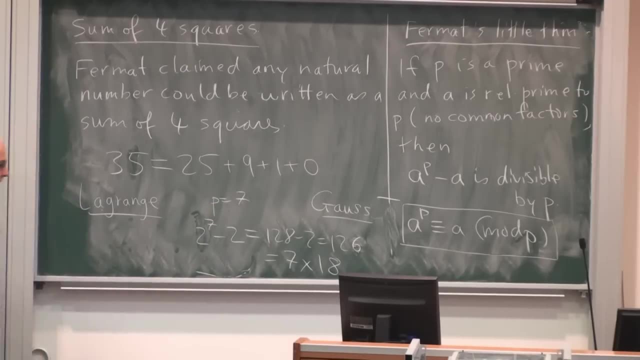 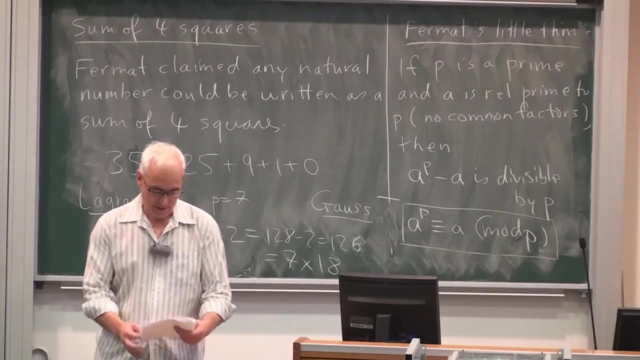 it also works for 3,, for 4,, for 5,, for 6,, for 723.. As long as 723 is not divisible by 7.. Alright, so Fermat was a great genius and sort of a mysterious figure in modern mathematics. 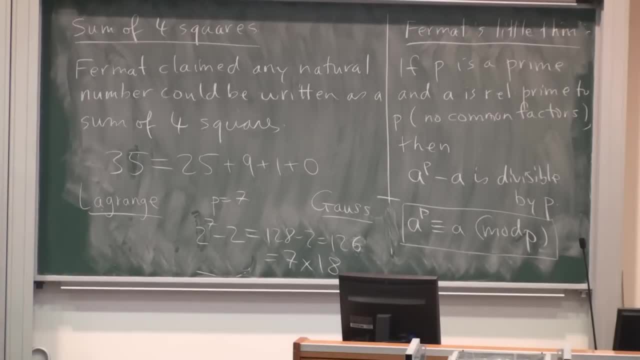 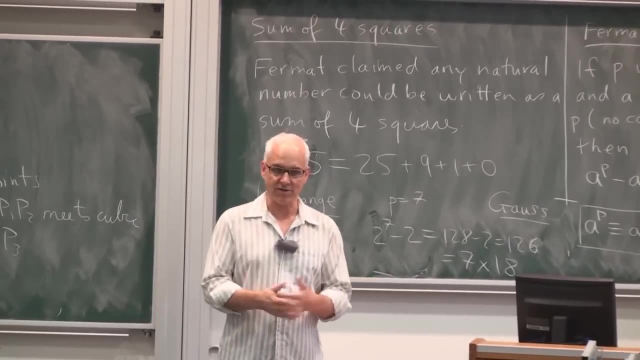 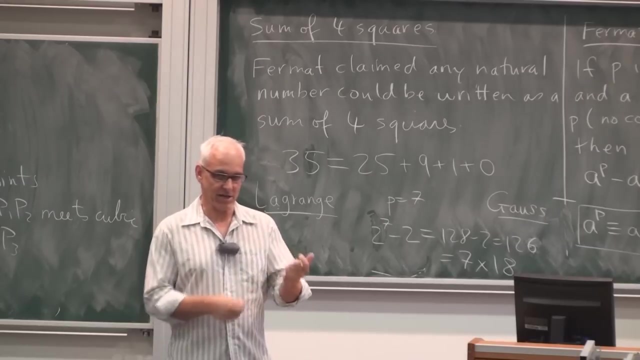 The founder of modern day number theory, and his legacy lives on very much, even today. Next time we're going to have a look at curves, Go back to some mechanics and some interesting curves that Bernoulli and others studied in terms of actual motions. 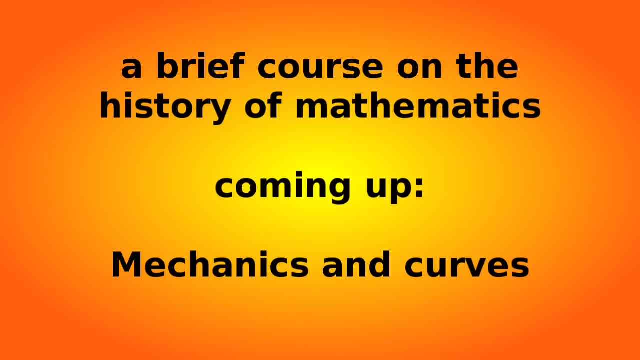 We'll see you then. © transcript: Emily Beynon. 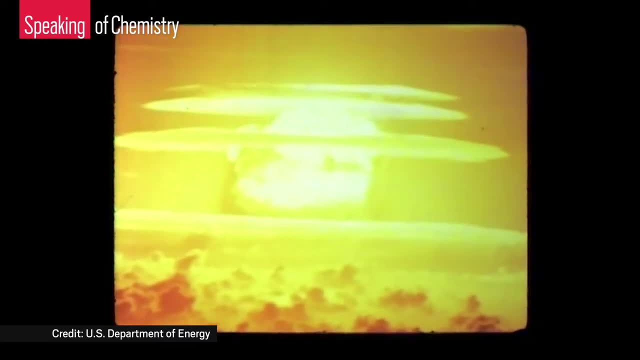 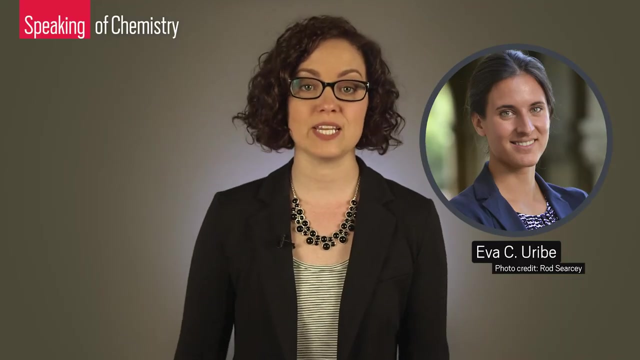 While you know, the revolution in nuclear physics was happening. they were understanding what happens inside the nucleus and what radioactivity is and what fission is. It was the chemists that figured it out. That's Eva Uribe, who studies nuclear chemistry and nuclear nonproliferation. 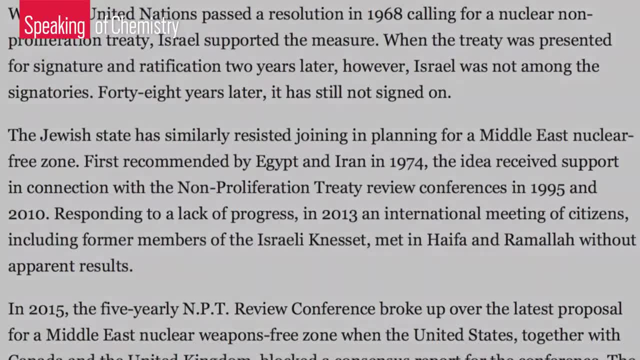 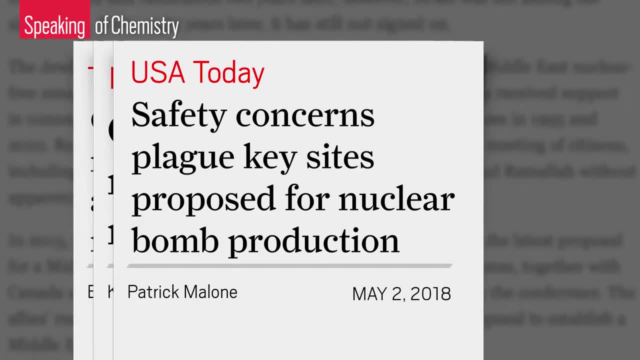 at Sandia National Laboratories. We're talking about those things because, well, they're on our minds And we wanted to know how chemistry is helping those who monitor nuclear materials globally keep tabs on who has which materials and what they might be doing with them. Those 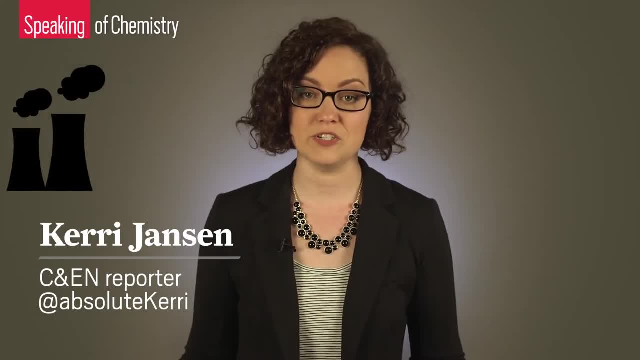 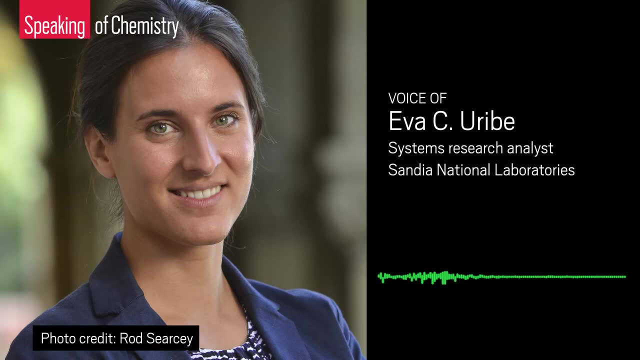 are hard questions to answer, especially since the same nuclear materials used to generate electricity can also be used to create weapons of mass destruction. There's huge benefits and huge risks to having this stuff around. So let's start with what this stuff is. The key materials used for weapons are plutonium-239. 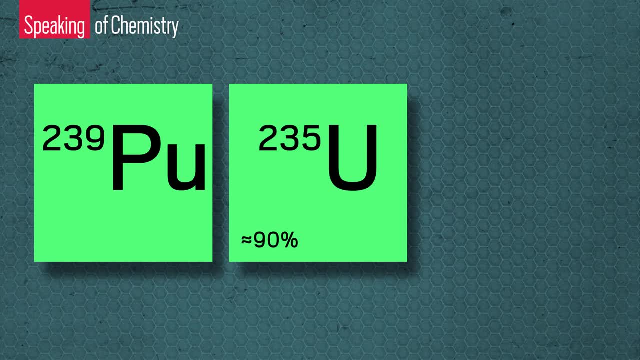 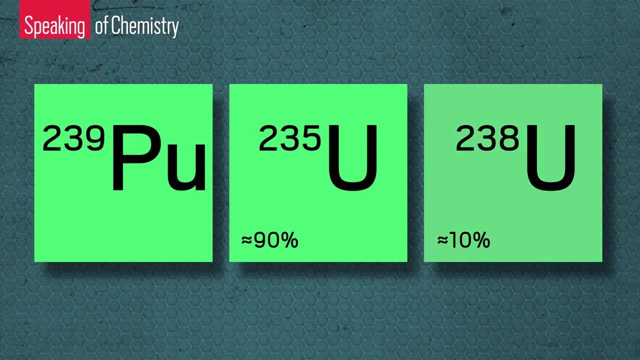 and highly enriched uranium. That is about 90% uranium-235,, which enables nuclear fission chain reactions, and 10% uranium-238,, which is about 90% uranium-235.. Uranium-238 doesn't really work as a weapon. Most nuclear reactors in the world run on.